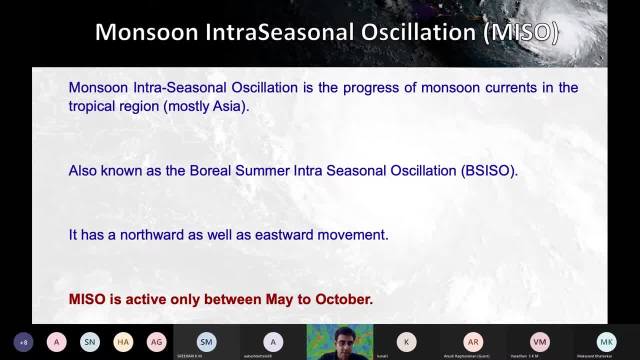 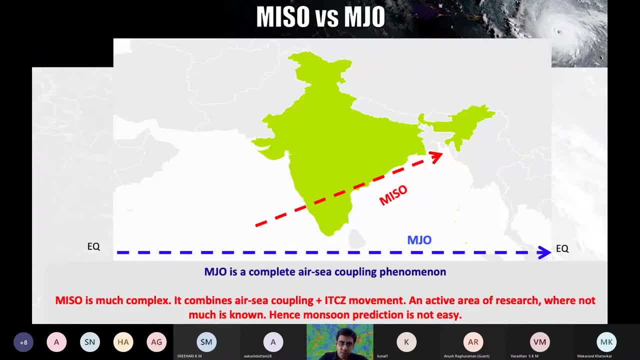 doesn't play a very primary role during May and October is because of the presence of this MISO, which is the monsoon intraseasonal oscillation. And I don't want to spend too much time, but I just want to show this one plot. Both of them are actually air-sea coupling, But MISO is much more. 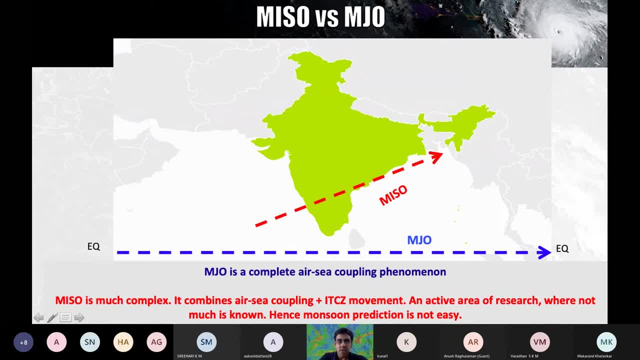 complex because It is the air-sea coupling. plus, it has to account for the ITCZ movement, which is the tropical convergence zone, which starts moving north during the onset of monsoon. So starting from May, this ITCZ moves northwards, correct? So this MISO has a very distinct feature where 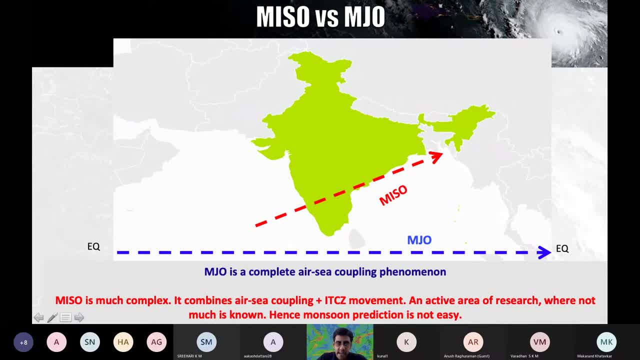 it moves from east to west- sorry, west to east, just like MGO- But at the same time it also has a north and south movement. So that is one of the important points that makes MISO very interesting, because it not only moves near the equator, but it 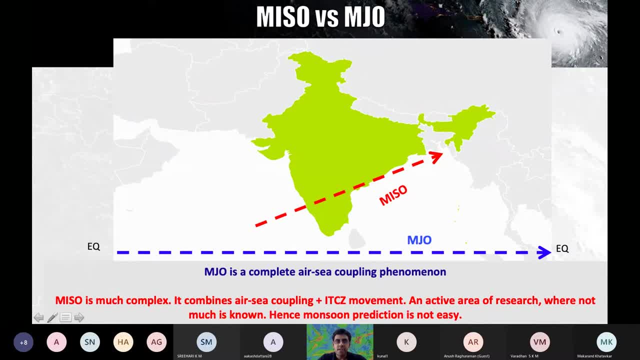 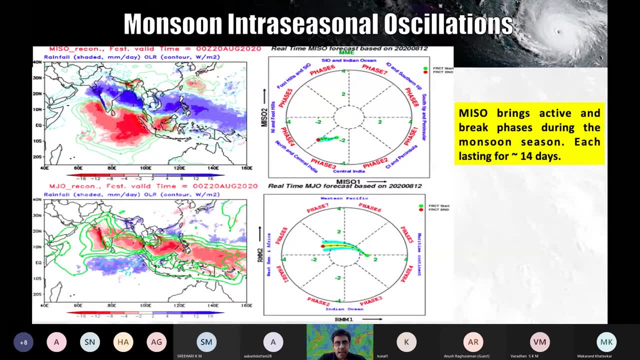 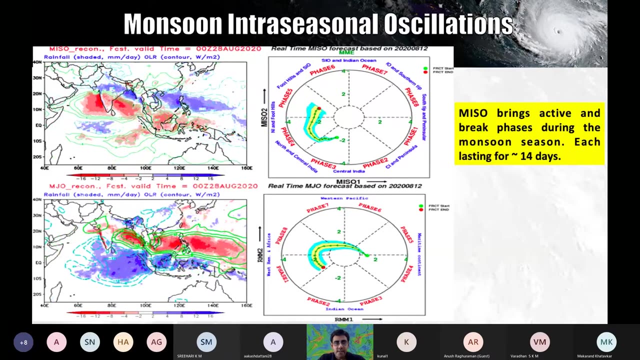 also moves along this meridional direction, which is north and south, And IATM Pune has an extremely nice MISO forecasting And it only puts out this forecasting between May and October, So only during the monsoon period. this MISO is present, because now, if you look at the IATM website, 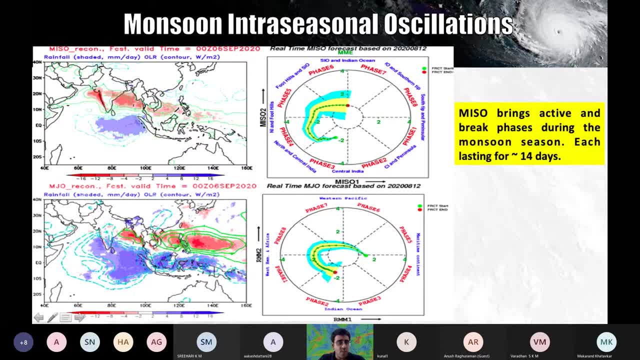 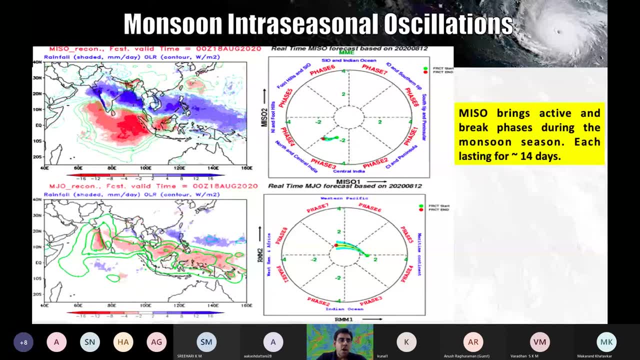 this MISO is not present because it doesn't make sense. ITCZ is not moving at all. right, ITCZ is not moving at all, in the sense it is not favorable for a monsoon system. So if you can see this particular plot during August, you can see. 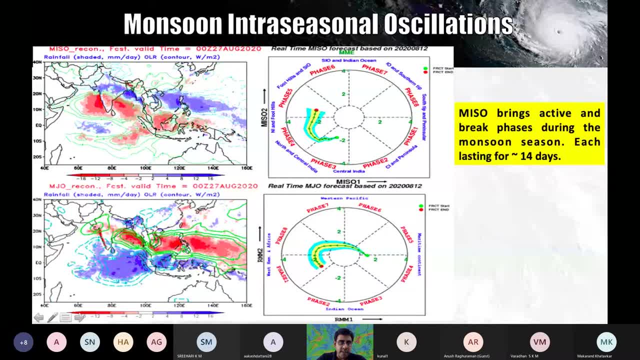 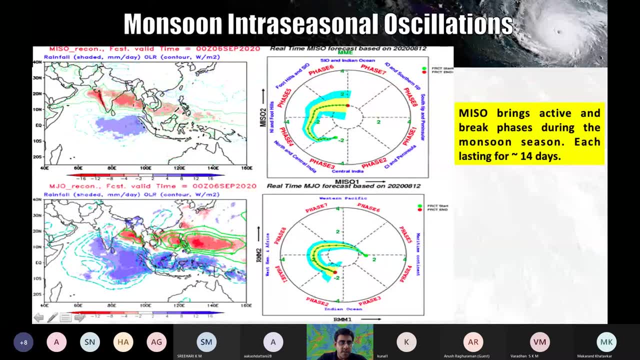 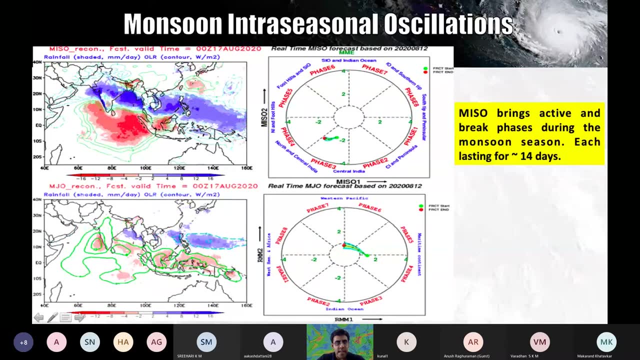 that red blue is the active phase of MISO, red is the weaker, is the break phase of MISO. So what happens is I'm always on the lookout for this active phase of MISO, which is this blue color, And I always want to see where is this blue phase. 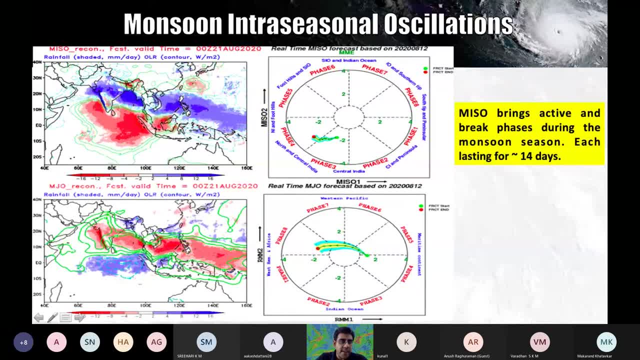 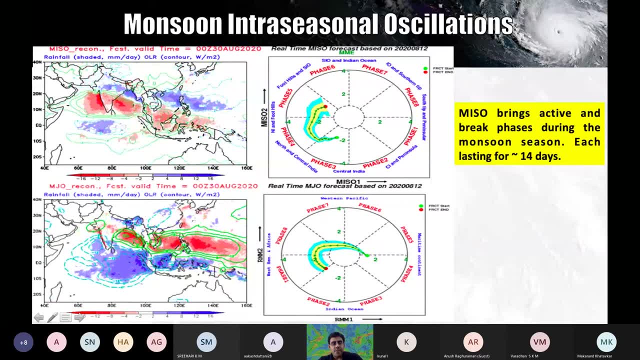 And that is going to tell me where the monsoon is going to be active. And, if you look at this, the monsoon is active over central India and west coast of India in around August period. And again, once again, this MISO is only as a guidance, but it gives a very interesting 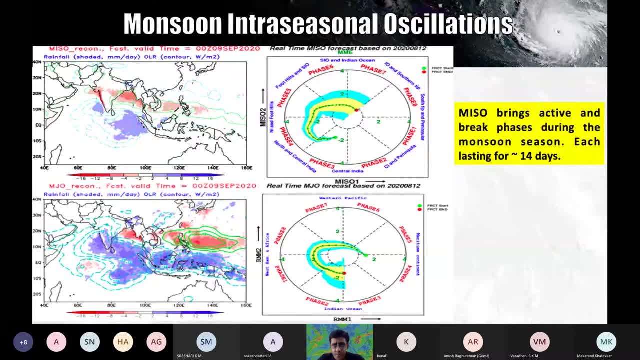 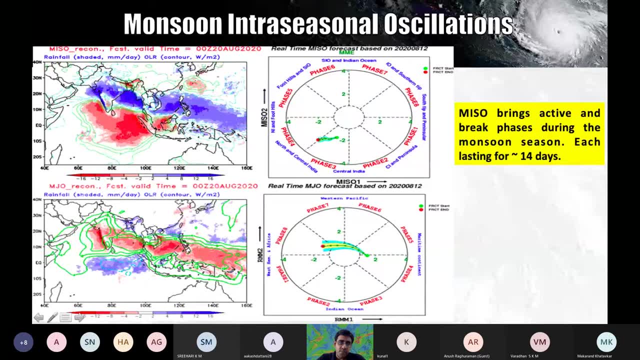 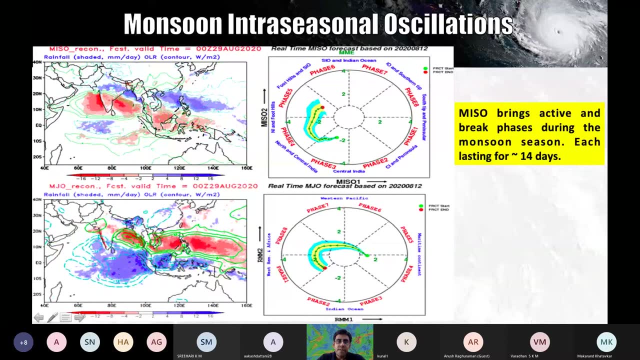 aspect of how the monsoon break and active phases are going to come towards India, And what IATM has done is it has divided into phases and each phase is actually named. You can see North India and foothills, foothills and South Indian Ocean. South Indian Ocean. 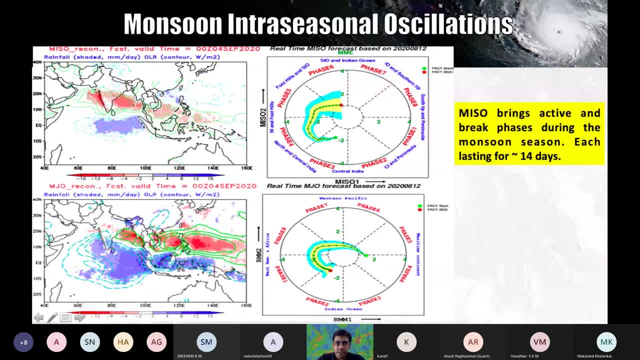 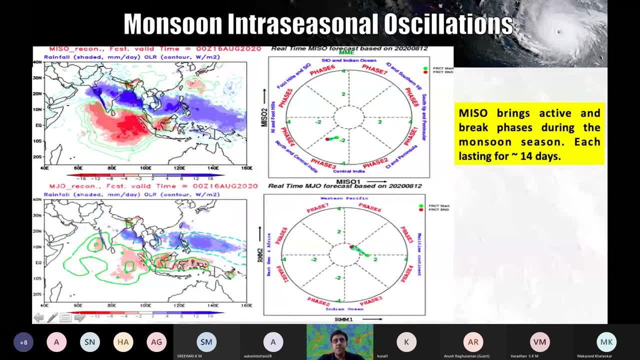 and Indian Ocean. Indian Ocean is North Indian Ocean, then the South Peninsula India, Central India, So it has given phases. So we are always on the lookout for in which block this MISO is in, because if the MISO is over Peninsula India, then Kerala will get heavy rains. Okay, 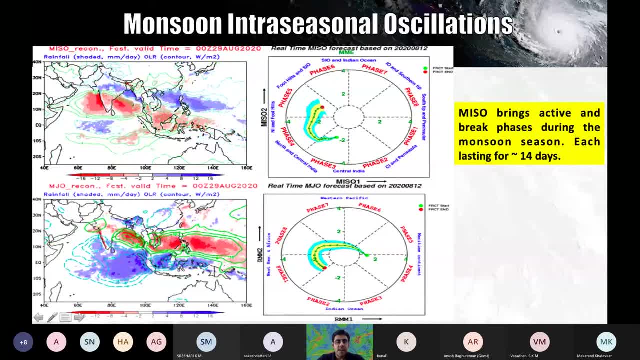 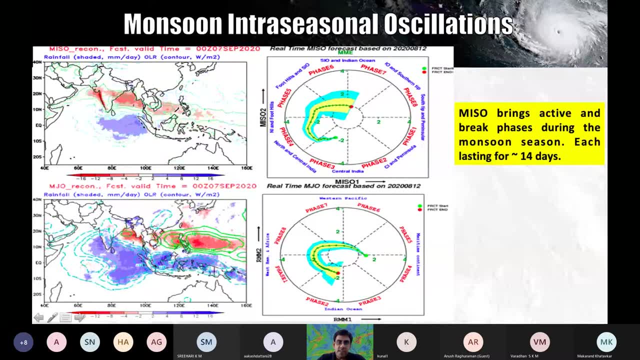 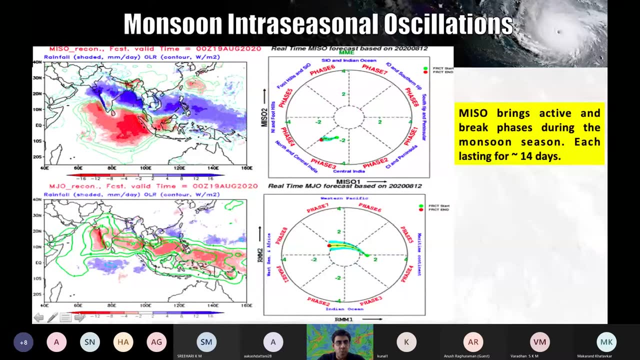 Whereas if the MISO is over central India, then the Konkan coast will get massive rains, Konkan coast plus Interior Maharashtra will get very heavy rains. When this particular MISO shifts to foothills of Himalayas, then the Northeast Asia, Northeast India and Northern India, like UP, Bihar, Northeast 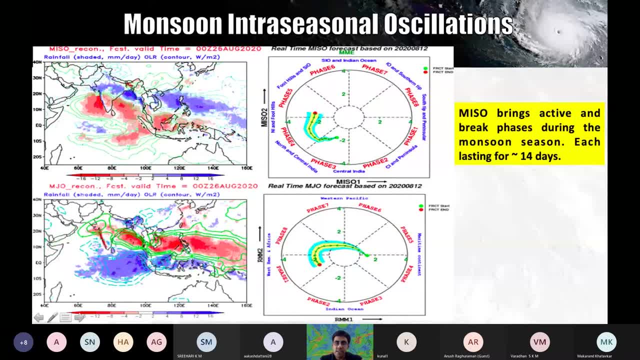 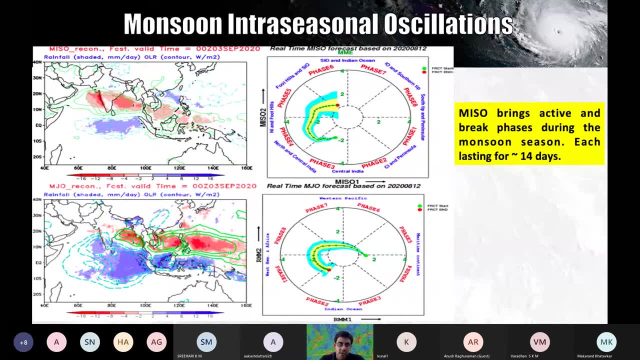 India and parts of North India will get rains. So this is the overall picture by looking at MISO which you can derive, which is a very interesting thing, I believe, because this is the large scale circulation of monsoon which is very important for understanding. 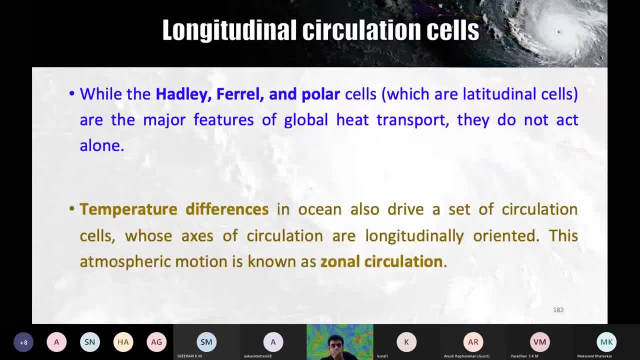 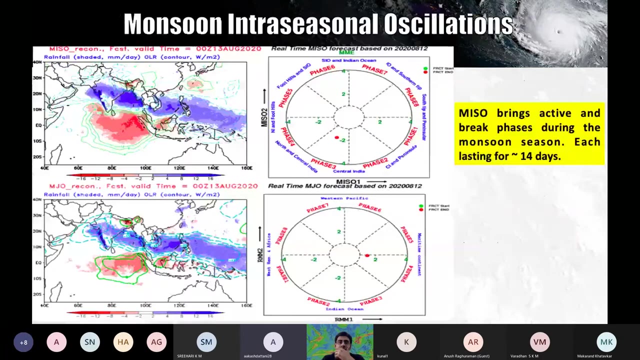 the active and break phases of monsoon. Okay, Two quick questions on the MISO please. So the MISO is synonymous with the monsoon trough, right, The monsoon trough is the MISO correct? And secondly, in the IITM chart one of the quadrants showed South Indian Ocean. So during 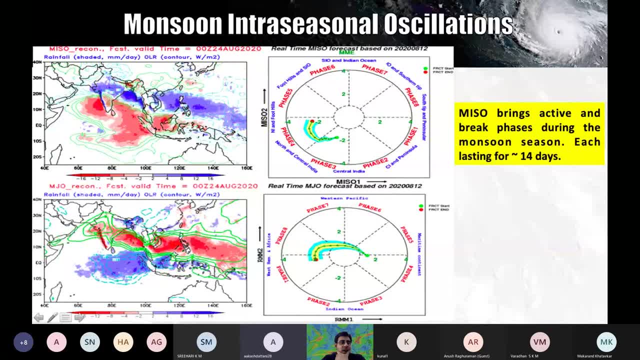 the summer monsoon? why? How would? how would you describe the monsoon trough? How would? how would you describe the monsoon trough? How would you describe the monsoon trough? Yes, So in the summer monsoon trough, as in, how would the monsoon be active in the 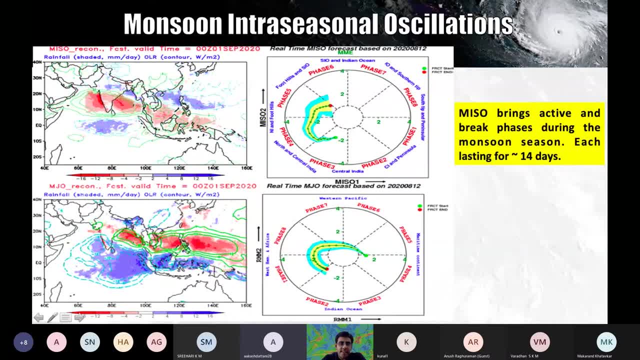 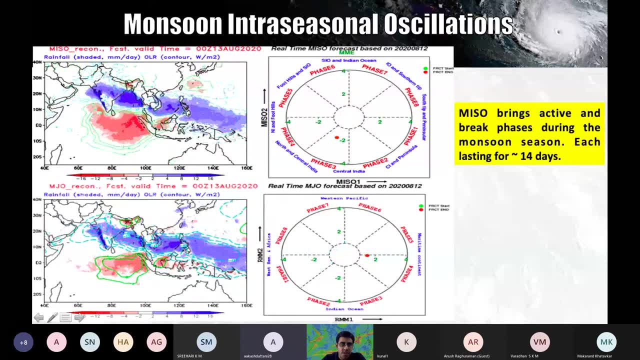 South Indian Ocean. So basically, that SIO in Indian Ocean is basically the not not South Indian Ocean, in the sense that it is starting from equator to the Indian Ocean And so so, of course, yeah, so it is starting from the. so, MISO, usually the, the, the forecast starts from the equator and it. 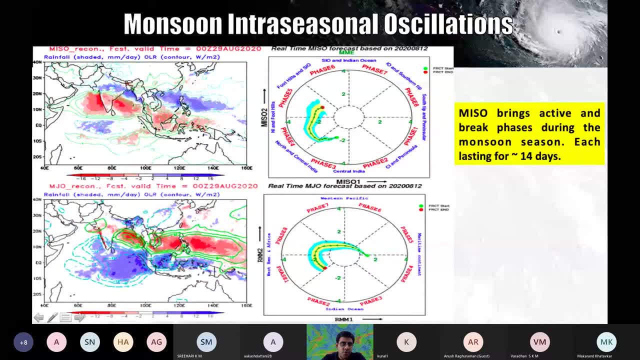 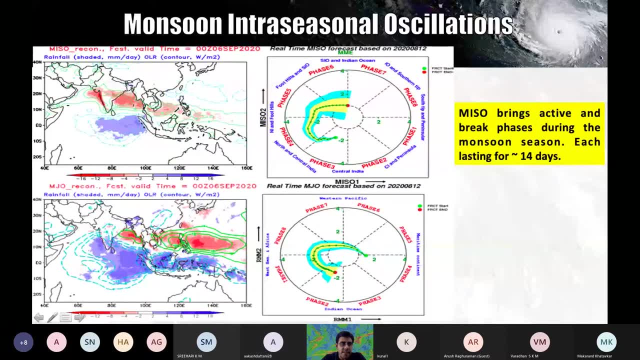 moves up north. So you can see, during monsoon most of the South Indian Ocean is very active, right. So you can see the monsoon activity in the south Indian Ocean. you know the monsoon very is completely inactive, right, it's only the indian part which is very active. 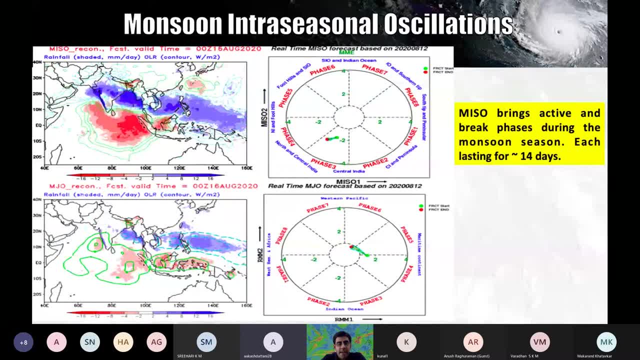 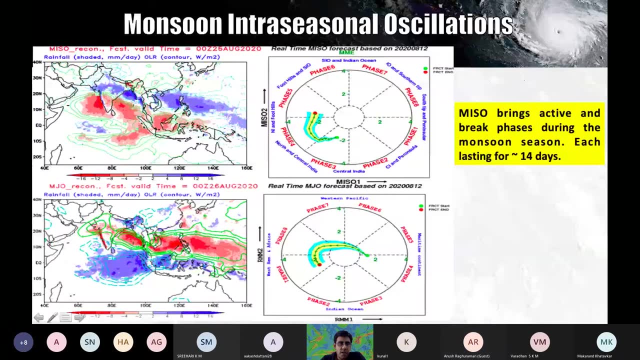 so this would refer to regions around, say, sumatra. yes, okay, thank you, sir. is the direction of miso similar to mjo, sir? it's it. what is the direction of miso, sir? so miso has moves uh west to east and also uh north, so it moves from the equivalent, it moves. 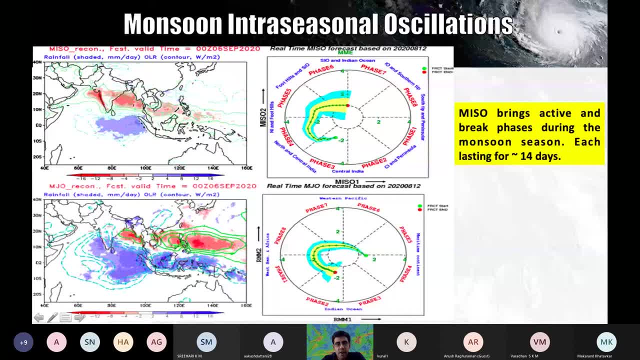 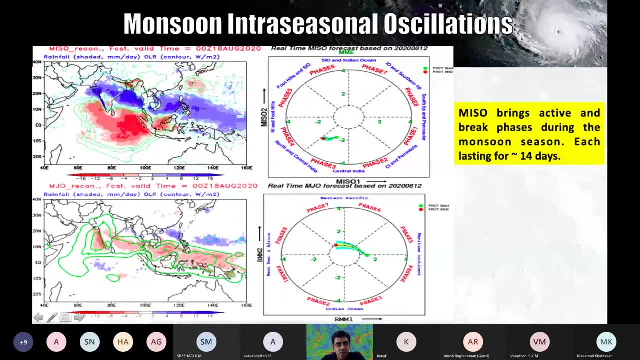 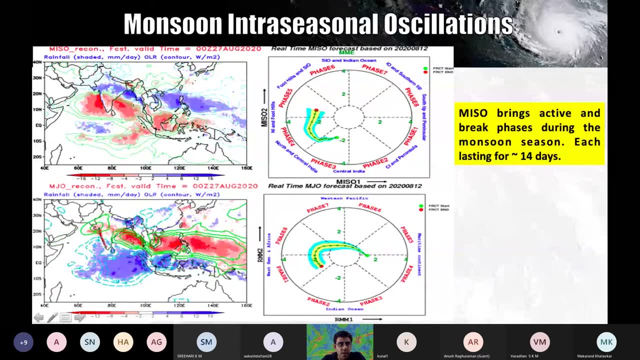 from, let us say, uh, somalia to sumatra or even further to south china sea, but at the same time it also moves north. that is what is very important. so if you look at the miso chart, then you can slowly see that. so this is that entire span and you can see that this also moving north, eastwards. 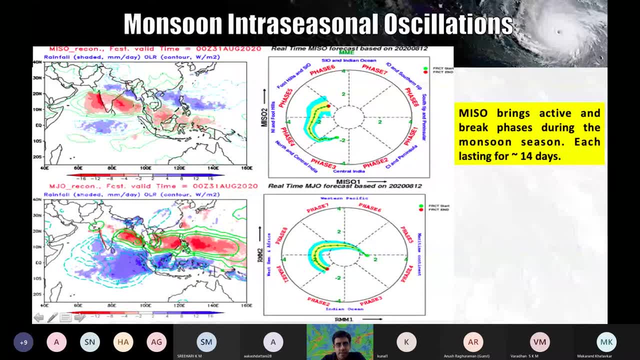 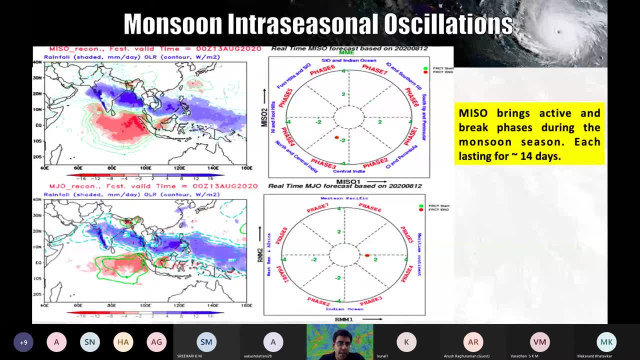 so see. so this: there's an eastward movement as well, so it has a direction similar to mjo, but on top of mjo it also has a northward movement, which is very important for monsoon. mjo doesn't give it, so that's why mjo is not a good indicator during monsoon season. okay, sir. 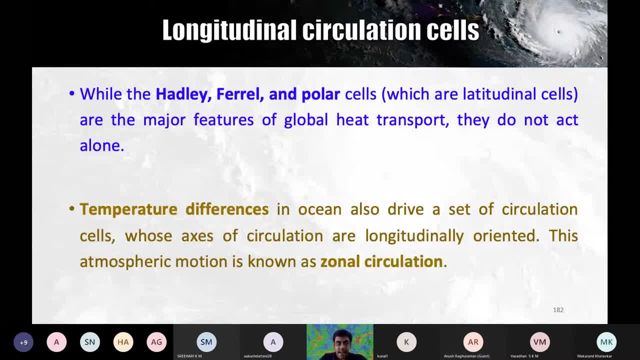 uh, sorry. so there is one more topic, which is the elleno and larina, which i forgot, so so maybe we can. we will try to cover that as well. so, uh, along these longitudinal cells, which are the hadley cell, uh, which we saw you also have. 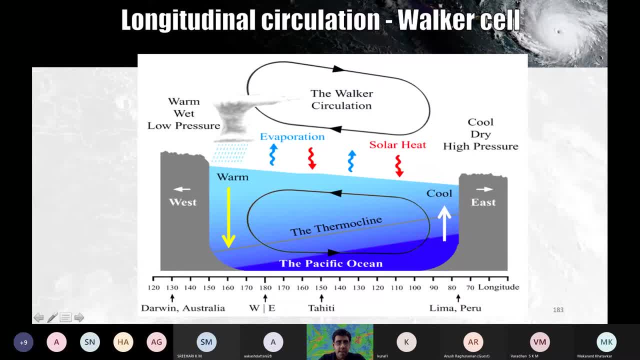 something known as longitudinal circulation cell, which is the walker cell. so walker cell occurs at a particular latitude which is close to the equator and the it. it is a longitudinal cell which extends along the ocean, so it extends from one end of the ocean to the other end of the ocean. 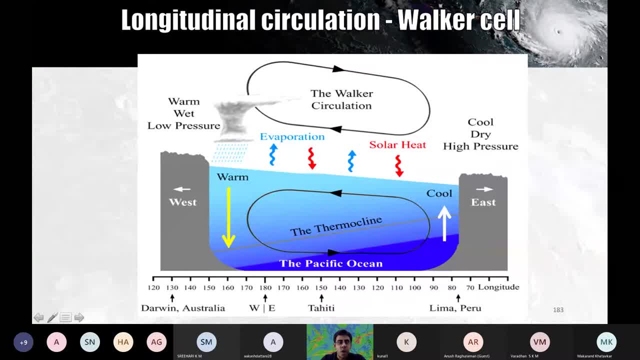 and that walker cell is very important because the strengthening of the walker cell is what allows the agencies to explain or kind of tell whether the enso phase has coupled with that atmosphere or not. so the walker circulation cell is nothing but a complete circulation cell in the atmosphere which is uh, which is over the ocean and uh, which actually tells uh whether the 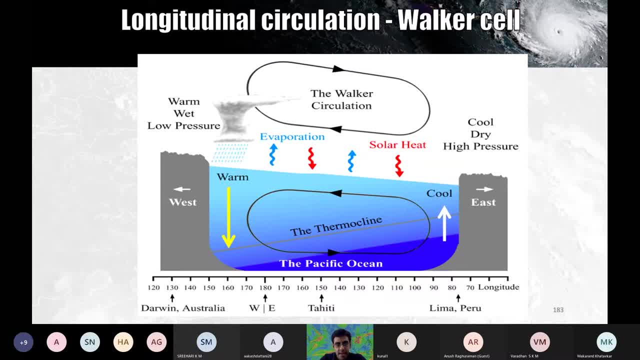 enso has coupled or enso has not coupled. and same with iod, also indian ocean time. okay, so this is not a meridional circulation cell, it is a longitudinal circulation cell extending along the longitude from one uh, from eastern, let's say western, pacific, all the way to the eastern pacific. 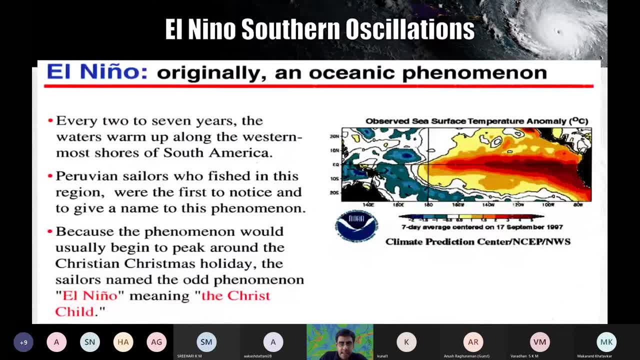 so it has different phases. we will talk about that, uh, when we talk about enso. so enso is, uh, basically the leno southern oscillation, uh. so in a very simple terms, uh, let us not get into the background because we don't have much time- 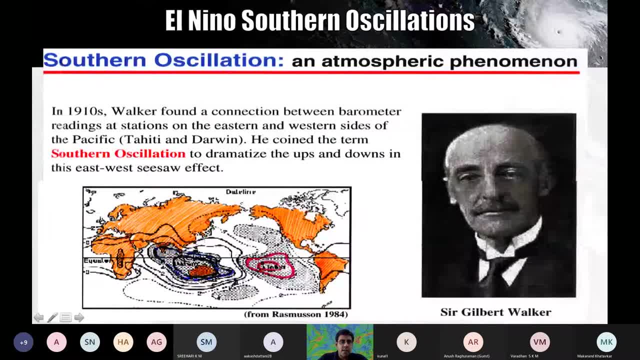 but it was walker who actually found this el nino phenomenon for the first time in 1910. what he did was he looked at these pressure pressure charts, again looking at the pressure charts, and he saw that in the western pacific sometimes what happens is the the pressure over. 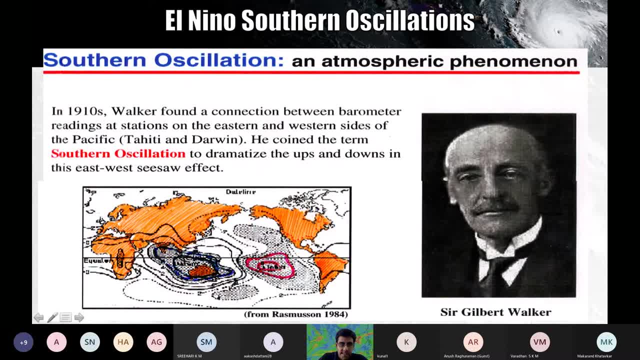 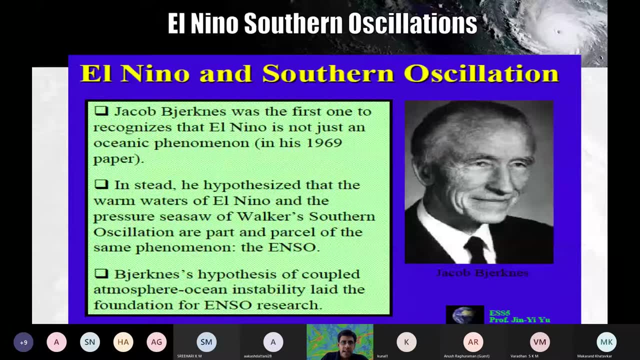 australia changes, uh to low. i mean, there is a seesaw in the pressure difference between australia and south america. okay, and then that's how he gave this term, which is southern oscillation. and at the same time, what people also observed was that in the ocean there is anomalous warming and anomalous. 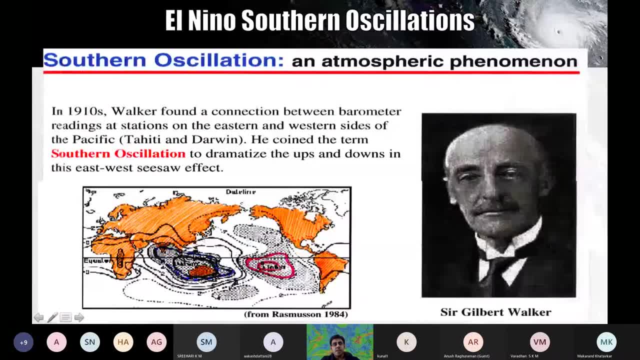 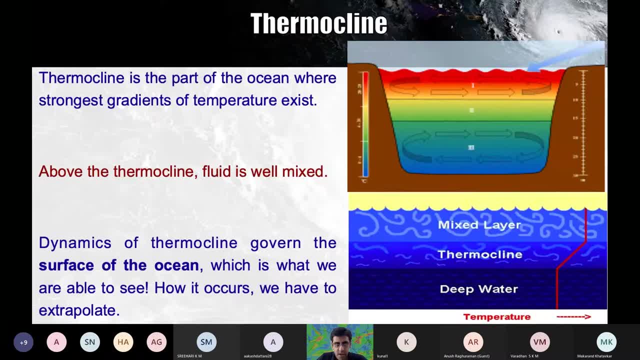 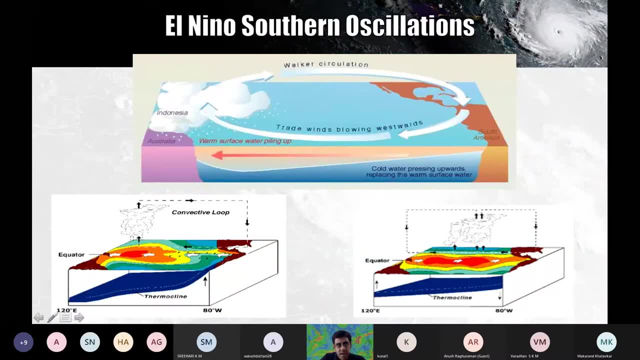 cooling along the pacific ocean. so this leno is a coupled ocean atmospheric phenomenon which is coupled into the atmosphere. okay, so let us look at what is this leno? southern oscillation. so what happens is during normal time. during normal time, there is warmer water over australia and there is 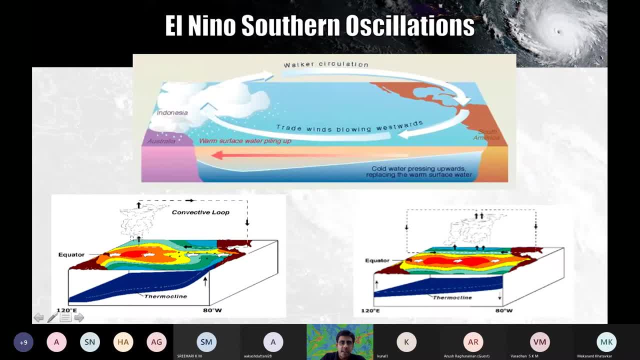 colder water over south america, which creates a walker circulation cell which has an ascending branch over australia and which has a descending branch over south america, thereby giving a lot of rains to the south asian countries as well as australia. now, during the phases of el nino, what 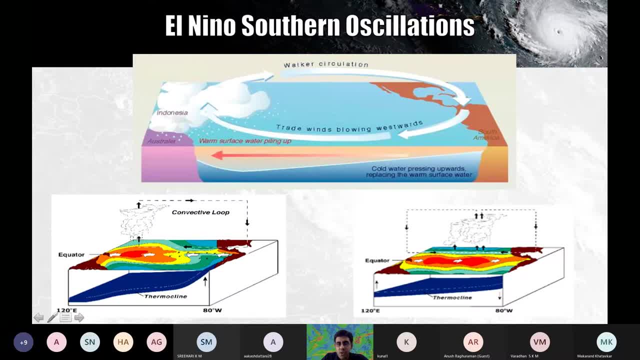 happens is the warm water from here moves to south america and the cold water from south america moves to australia, thereby changing the direction of the walker cell. so now the walker cell direction changes where the ascending limb is over south america and the descending limb is for the is. 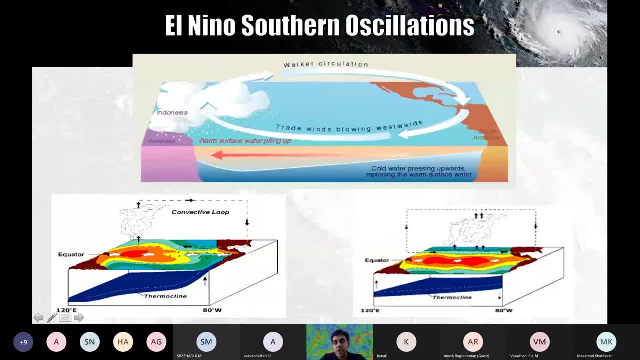 over australia. so the reversal of walker cell is all is what is called as, what we call as el nino. so this is the, this is the el nino. so you can see that the walker circulation cell has reversed. now there is a descending branch over australia and an ascending branch in the central pacific. 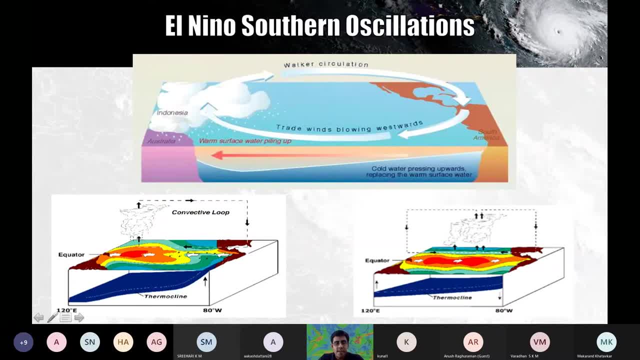 whereas this is the lanina where the walker circulation cell actually strengthens, in the sense that it becomes much stronger compared to its normal state. so the normal state of walker circulation cell in the pacific is ascending branch over australia and descending branch over south america when it strengthens. so when, when the pressure over australia drops further down, then it 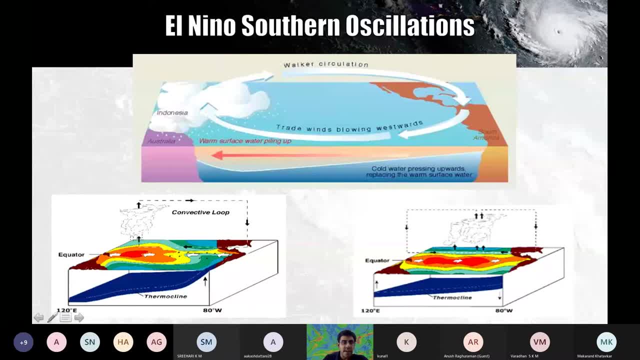 is a signal that larina is going to emerge. when the pressure signal over australia increases, then that means that there is a possibility of el nino. so this el nino and lanina are basically governed by the movement of the water along the pacific, between the western and eastern pacific and the 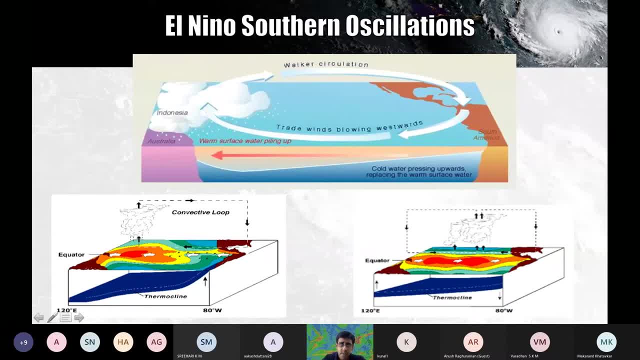 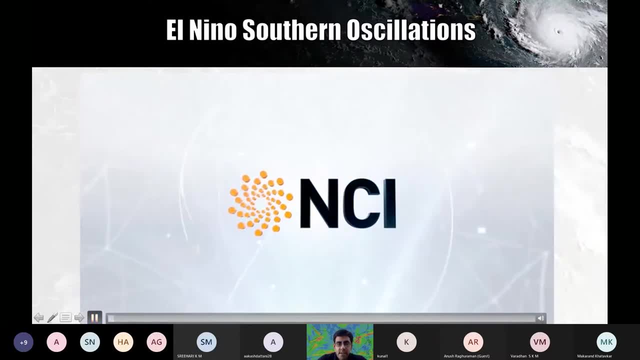 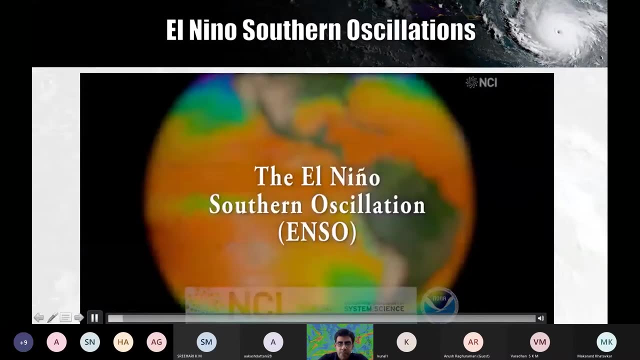 associated walker circulation cell that forms in that class. okay, uh. so if there is a very nice movie, uh which is uh, which was uh which is present, uh, in this particular, i have taken it from youtube, so it is from the climate system, science and la nina events, collectively known as enzo, generate profound 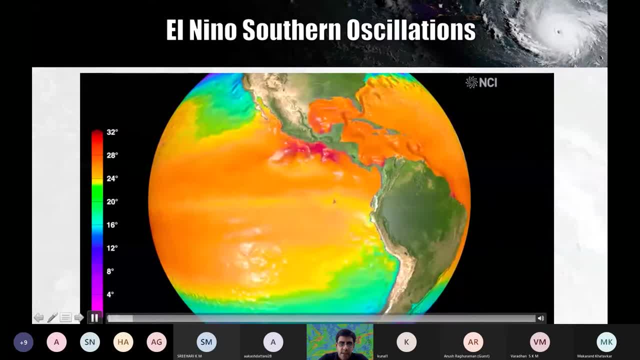 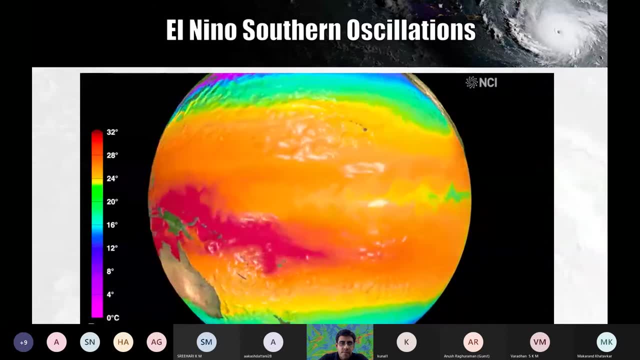 year-to-year changes in weather patterns around the world. so i will share this with you and you can see that supercomputer we have recreated the strongest el nino on record in late 1997. that was followed by two back-to-back la ninas. the heart of enzo is in the vast tropics. so this is the. 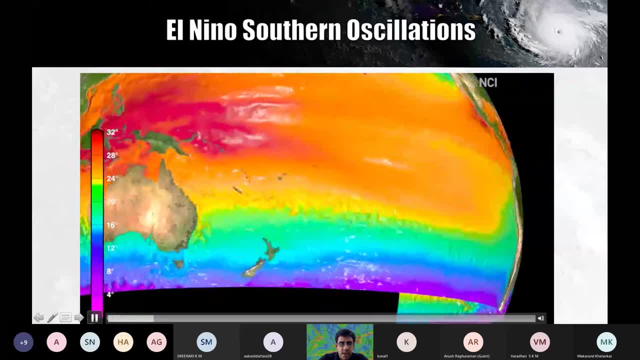 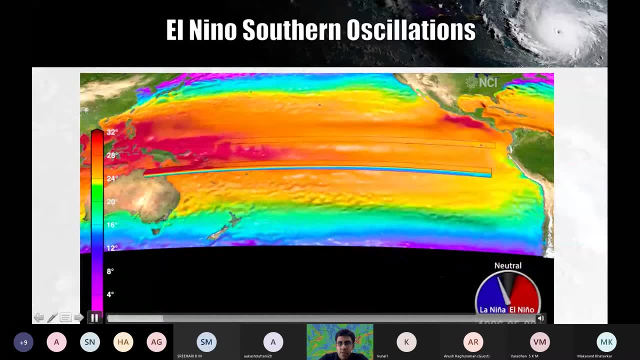 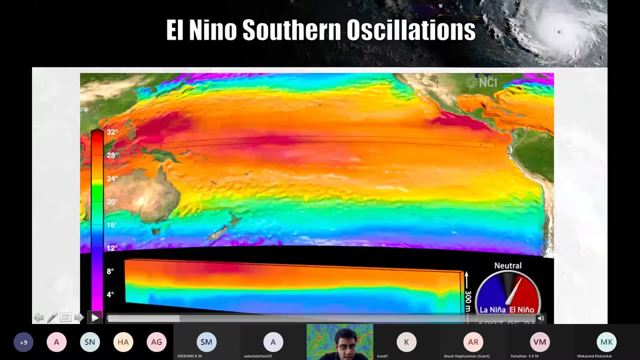 australia, where there's much of the action occurs below the surface. warm water to see. you will see that there's warm water slice of the ocean along the equator and slowly this warm water will move. a massive pool of warm water sits in the west. so this is the normal state. this is the normal state of the ocean. 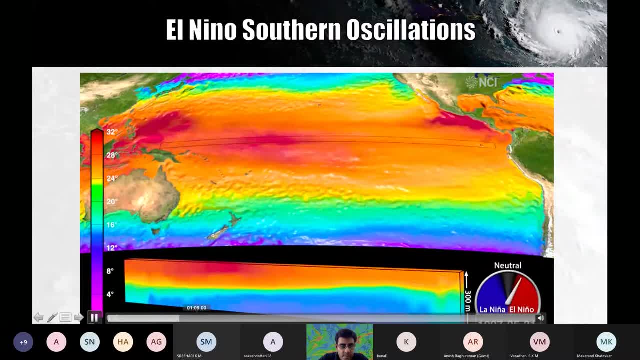 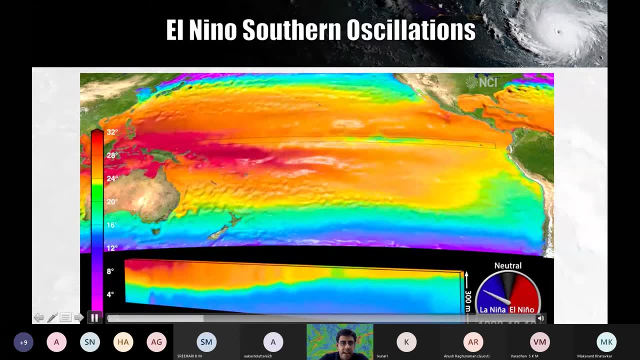 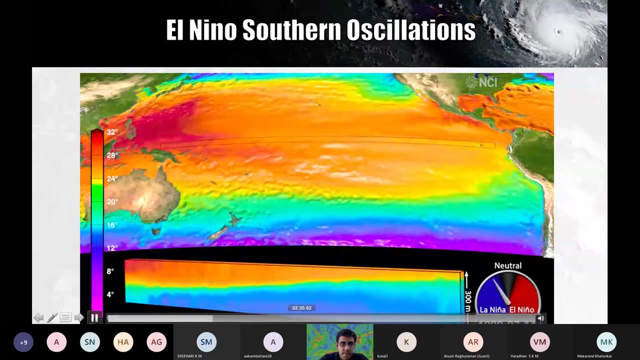 and for. so this is uh. it's for el nino to form cools and the warm pool reforms in the west. so this is lanina, where the warm water is getting warmer and warmer. thereby, this temperature contrast across the equatorial pacific is linked to the westward blowing, and if you look at ld no, i think i will share this video. you can look at it. 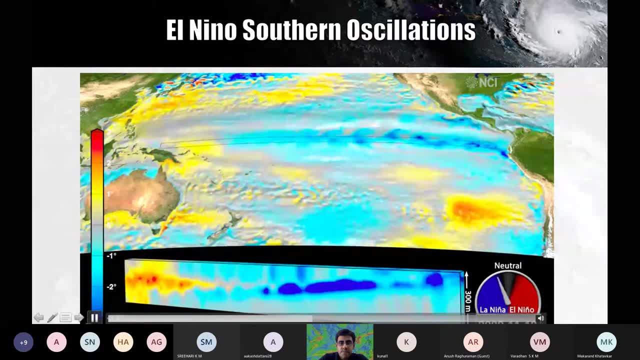 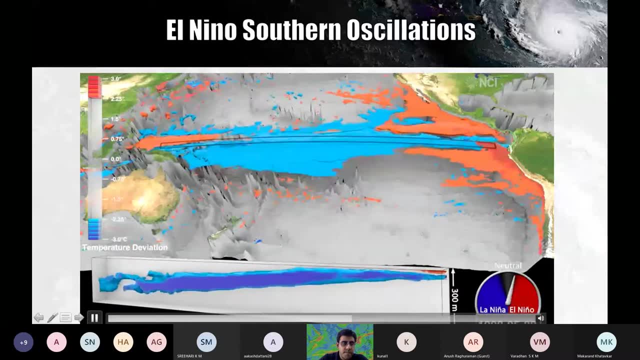 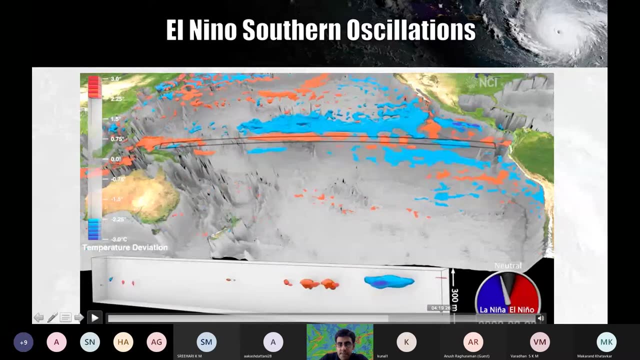 see during el nino what happens is by peeling away the ocean surface, we can see how ocean currents move heat around into the indian ocean through the indonesian archipelago. so you can see that now the water waters have collected over south america. i'm just trying to find this. el nino changes. 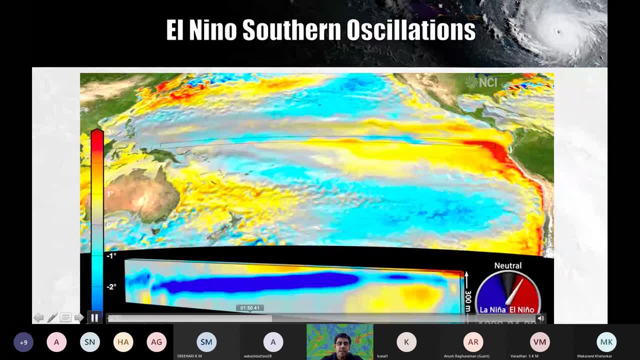 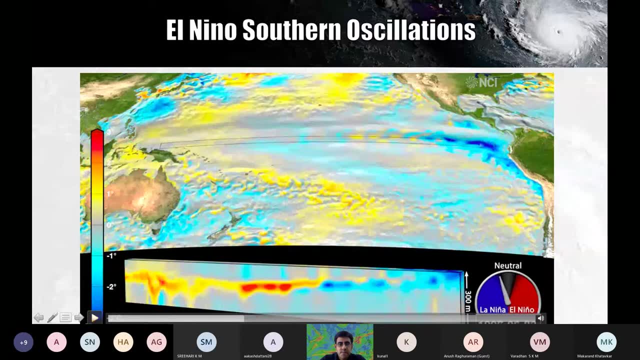 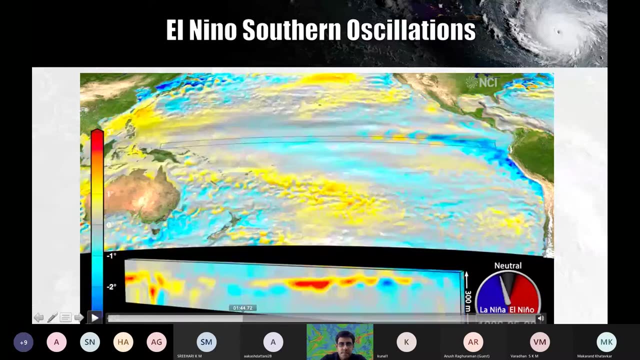 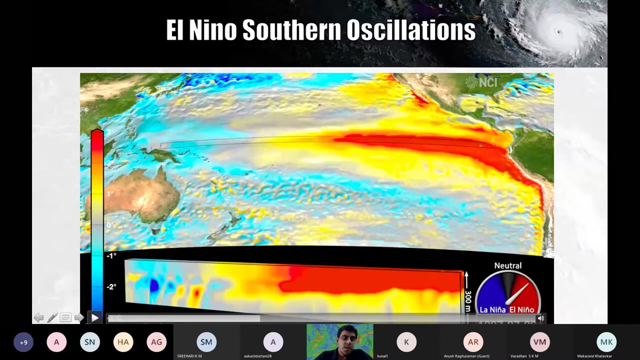 just give me one second here. yeah, so this is el nino, where the warmer water is now. yeah, so, i mean, yeah, so this is the classic el nino, where the warmer water ships to south america and the colder water is over australia, and this actually leads to the reversal of the walker's. 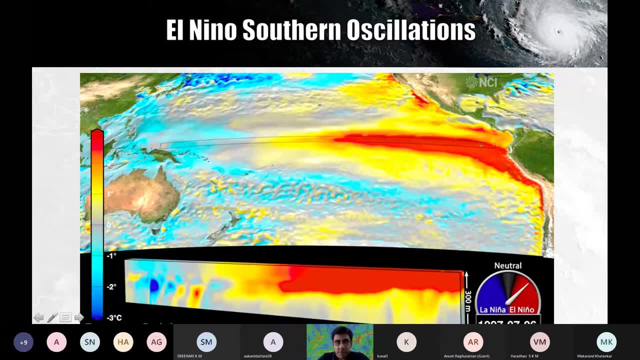 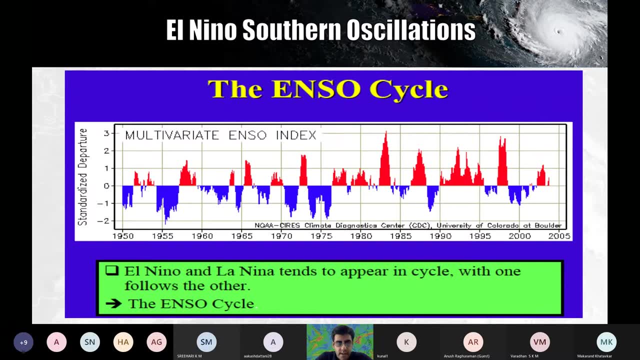 location cell And these are the patterns that we are on the lookout for. okay, So ENSO cycle. there is a cycle which used to be there. If you look at the record, then after every El Nino there has to be a La Nina. 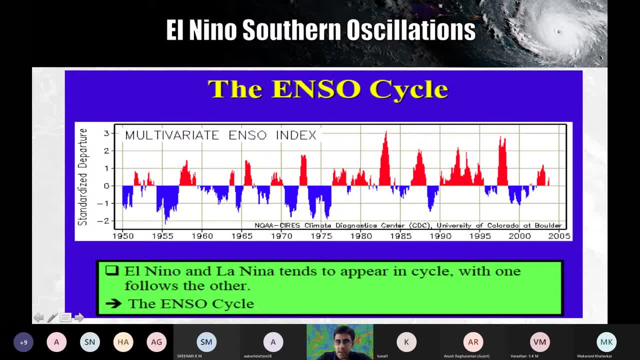 So you can see that they come in phases, But over the years, with climate change, you can see that this pattern has been disrupted, where you are now seeing longer periods of El Nino and shorter periods of La Nina, And this is a classic example where you saw El Nino persisting for a very long period of time. 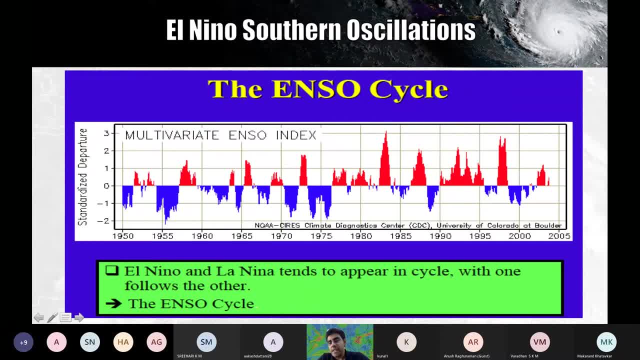 And now also, we did not have a La Nina after 2013.. 2013 was our last La Nina year And now 2020 is the. I mean by La Nina I mean moderate or strong La Nina. So 2013 or 2012 was the last strong La Nina. 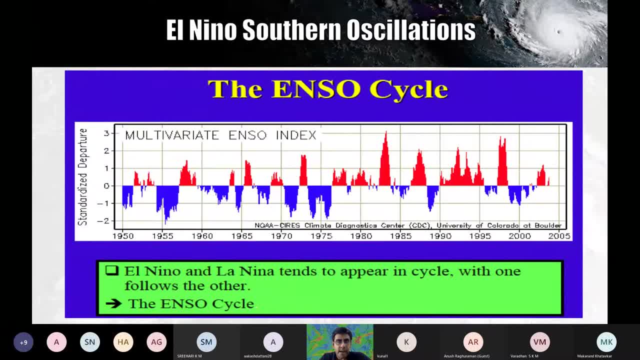 After that, after eight years, we are producing La Nina, So the ENSO cycle, so El Ninos have increased whereas La Nina has decreased. The reason people are pointing it? mainly because of the way the ocean is responding towards this global warming that we are putting into the atmosphere. 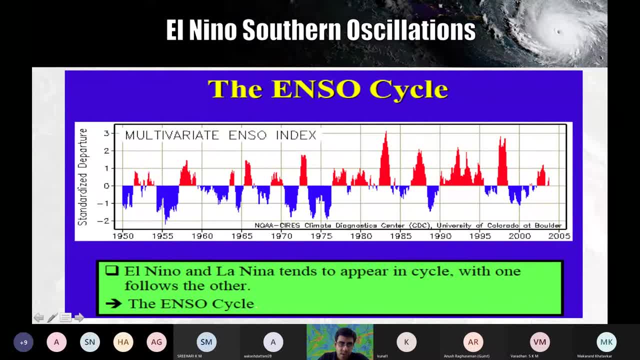 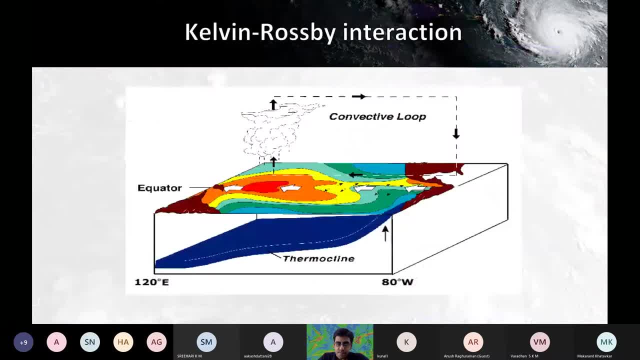 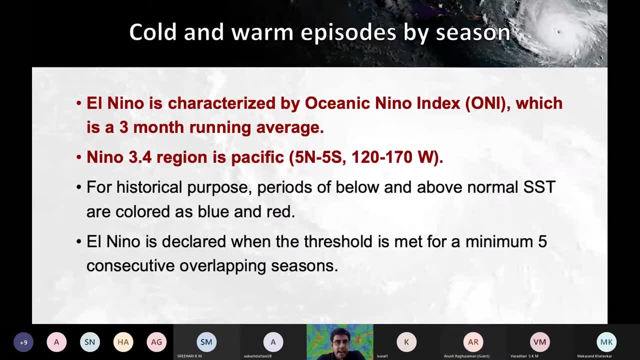 So this cycle is something which it used. there used to be a pattern, but that pattern is getting disrupted, So we need to understand that particular pattern. I'll skip this, Which I don't think we need to. So how is El Nino and La Nina characterized? 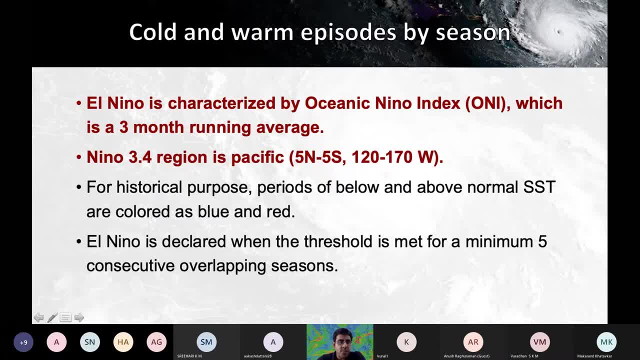 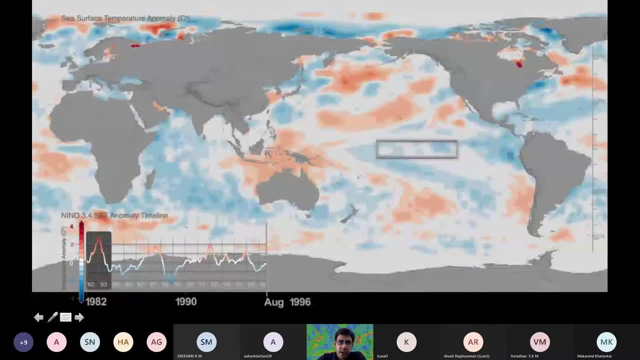 So El Nino is characterized by looking, Looking at something known as a Nino 3.4 index, which is the region in the Pacific, which is this particular region. So what climate scientists do is they look at the temperature variation over a period of one month or over a period of three months in this region. 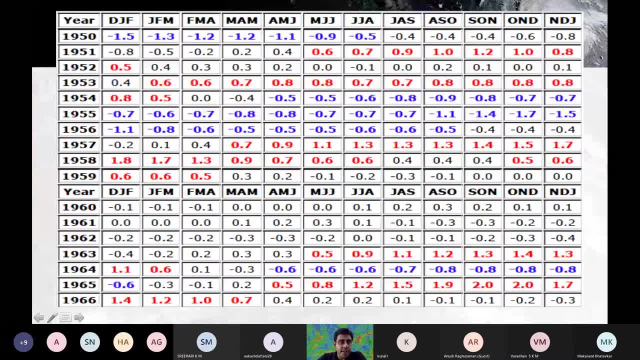 And they come up with a. they come up with a three-month average And whenever the three-month average sustains so, minus 1.5 means lower than normal temperatures in this region, Okay, And red means higher than average temperature over that region. 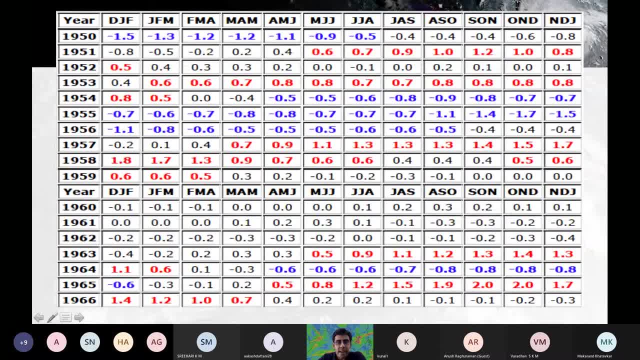 So lower than average temperature in that region means La Nina. so the blue means La Nina and red means El Nino. and they look out for this index. it should if it sustains for five consecutive months. Okay, So if you see this index in red for which is up, which should have a value of greater than 0.5, if you see this index for consisting consistently for the five months, 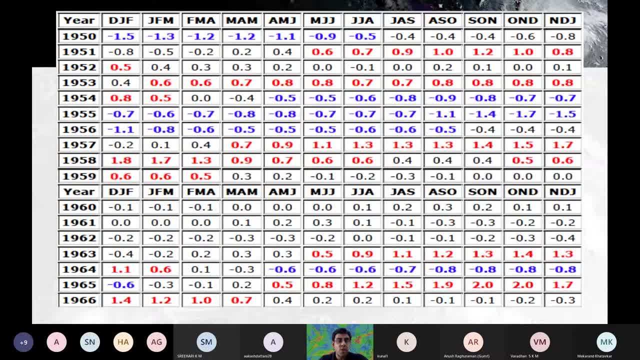 Okay, Then they signal that El Nino watch, they give a El Nino watch, So there is a watch, then there is an alert and then there is an El Nino announcement or La Nina announcement. Okay, So this particular anomaly should sustain itself for consecutive five months. 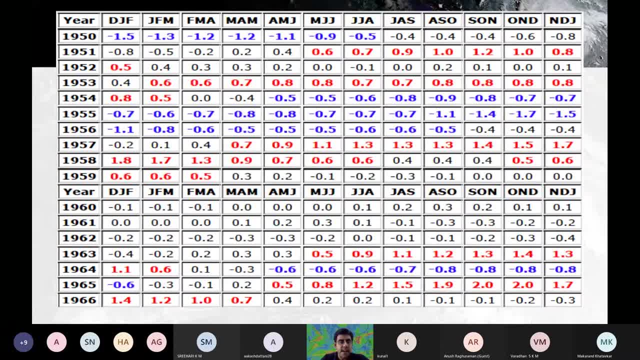 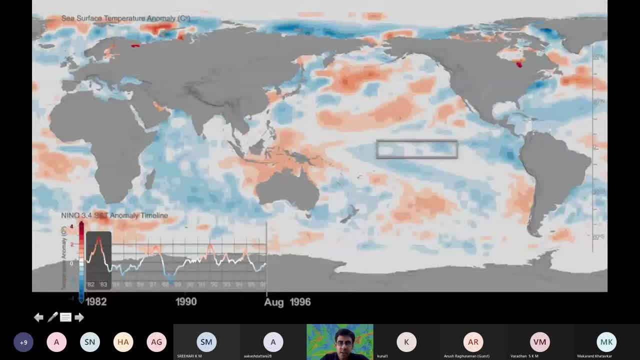 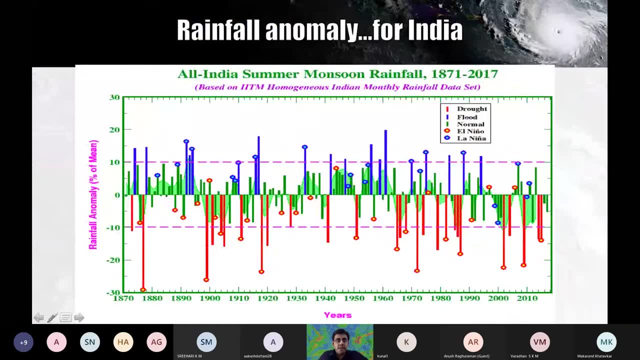 Then only ocean and atmosphere will couple itself and an El Nino signal, full-fledged El Nino or La Nina signal, would have emerged. So climate scientists usually look at this particular area. So if there is an El Nino or La Nina signal, they will announce whether an El Nino or La Nina is going to form or not. and why is the El Nino not good for India? the reason is because from this again, from this all India, summer monsoon rainfall from 1817 to 2018 or 2015,. they have taken and they have seen that most of the so this is La Nina. most of the La Nina years are associated with above normal rainfall and most of the El Nino years are deficit. 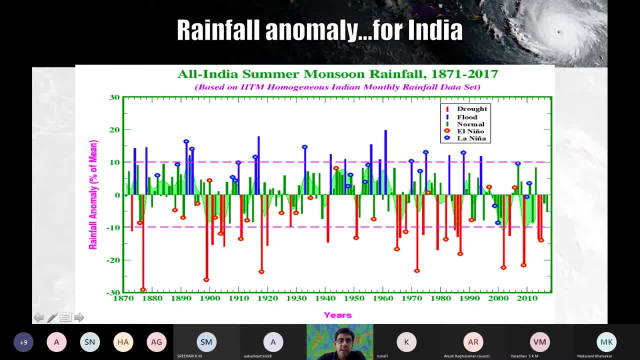 So you can actually correlate this black- sorry, this red- circle and the Whites and the green and the blue circles and you can see that El Nino is bad whereas La Nina is good, except some years which- this is 1997, when it was a very strong El Nino but rainfall was normal, mainly because of the presence of IOD. 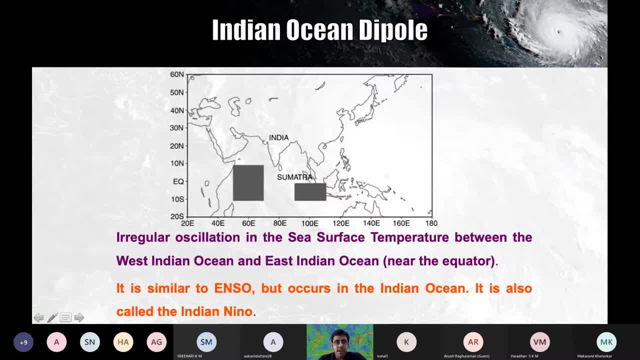 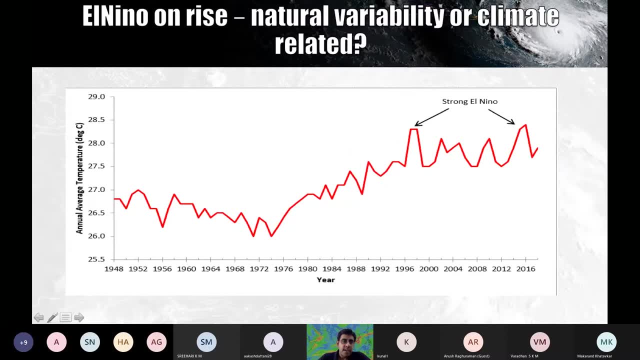 So around 1997 is when people started looking at the Indian Ocean Dipole, which is the counterpart of El Nino. Okay, So I will go to Indian Ocean Dipole, but before that I just want to show you this average annual temperature of an ocean of the Pacific Ocean. 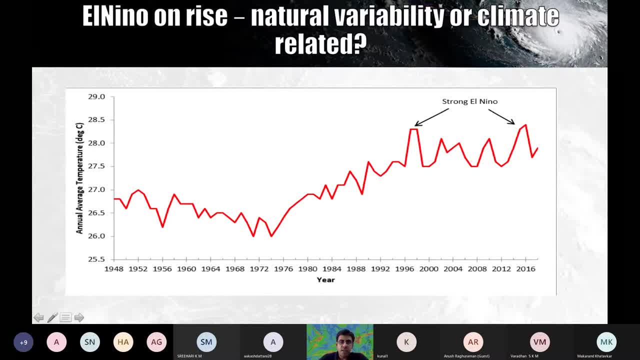 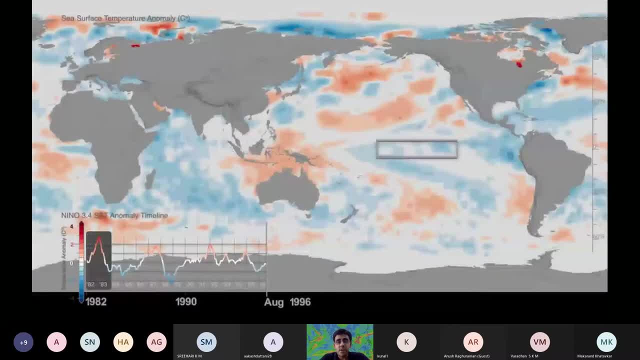 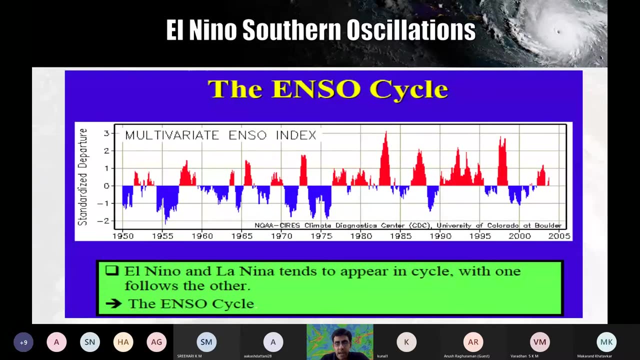 Which is actually increasing over the past few years, triggering strong El Nino and longer El Ninos. so the phases of, not the phase, the cycle of ENSO is now favoring more towards El Nino than La Nina. That's what I'm trying to tell you. 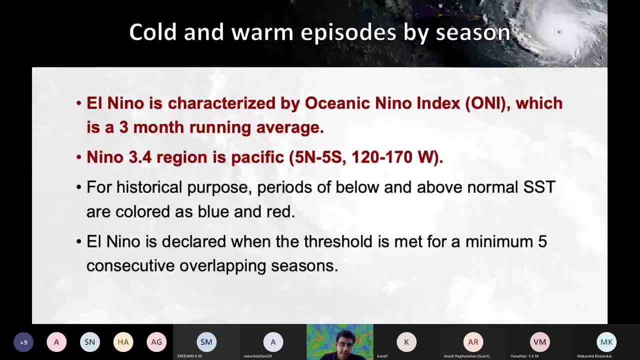 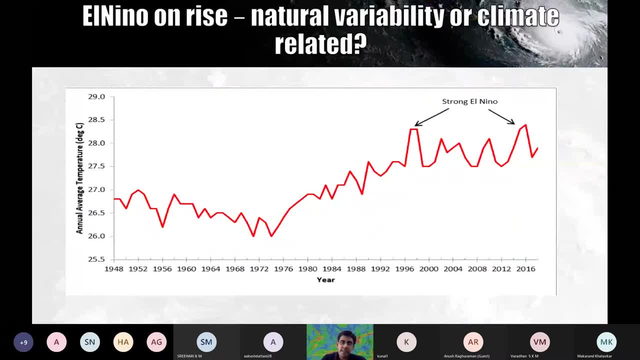 Okay, So we should be, we should embrace ourselves for more El Nino type of events compared to La Nina type of events, because that is what the statistics is saying. But that doesn't. That doesn't mean that our monsoon will will be deficit. 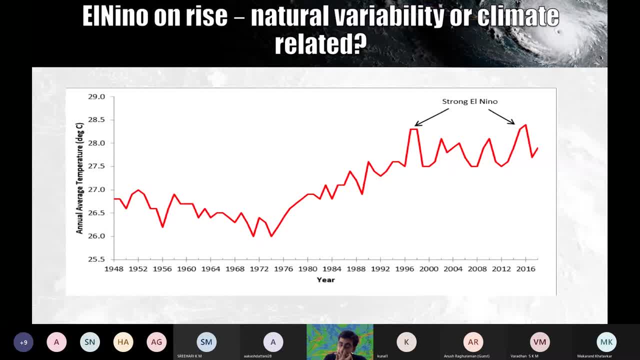 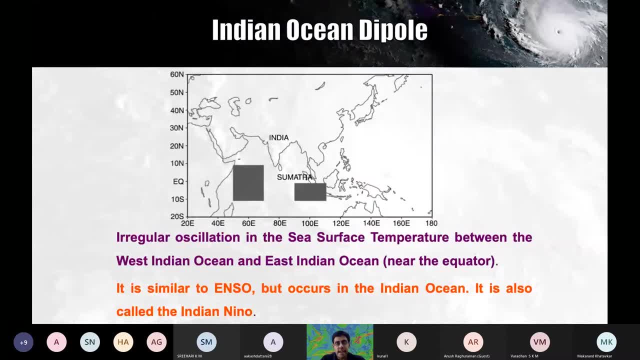 And the last two years, we have seen that 2019 was a classic example of a very low excess monsoon, even though El Nino was present last year, And that is what pushed the scientists to find out this other phenomenon in the ocean, which is the Indian Ocean Dipole. 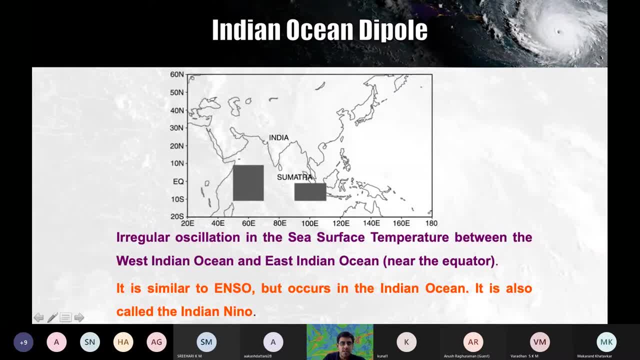 This Indian Ocean Dipole is a very local phenomenon to Indian Ocean, which is between the Somalia coast and the Sumatra coast. Okay, It is very similar to ENSO, but it occurs in the Indian Ocean, Hence it is called Indian Nino. 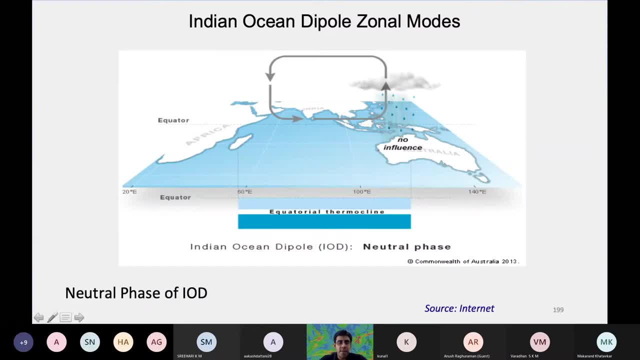 So let us look at this Indian Ocean Dipole. So during the normal Indian Ocean Dipole, the neutral phase of Indian Ocean Dipole, what happens is you have a colder water near Somalia and you have warmer water near Sumatra. 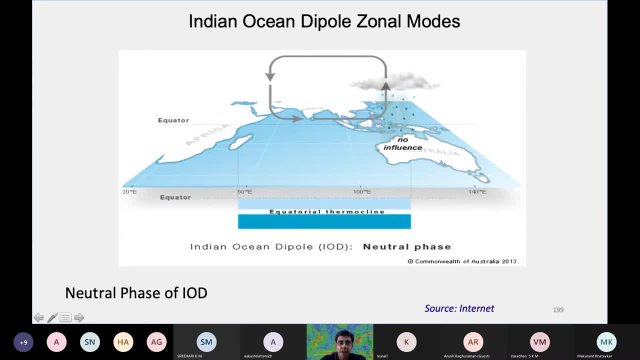 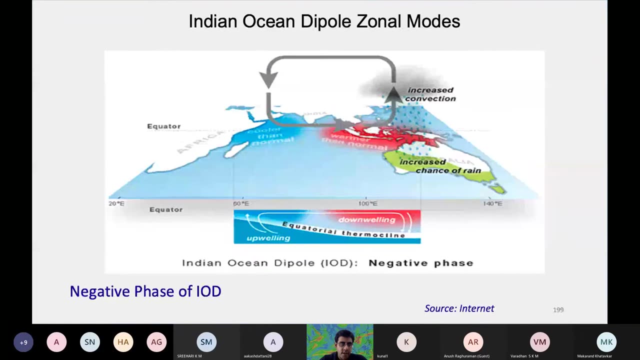 So that kind of gives favorable rains to, or more rains to, Southeast Asia compared to India during the neutral phase. But during Indian Ocean Dipole phases- neutral Indian Ocean Dipole phases- India gets normal rainfall Okay. However, During a negative phase of IOD, the cooler water becomes more cooler and the warmer water becomes more warmer, thereby triggering a stronger walker circulation cell near Southeast Asia or Australia. 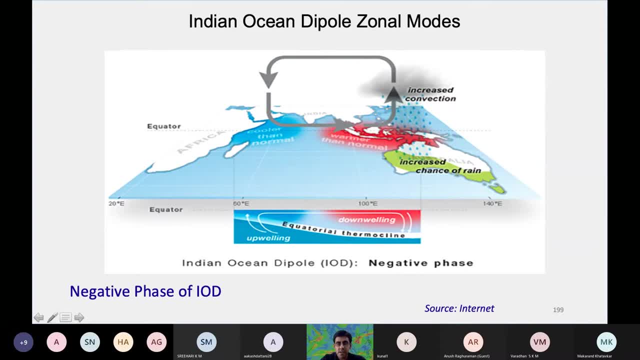 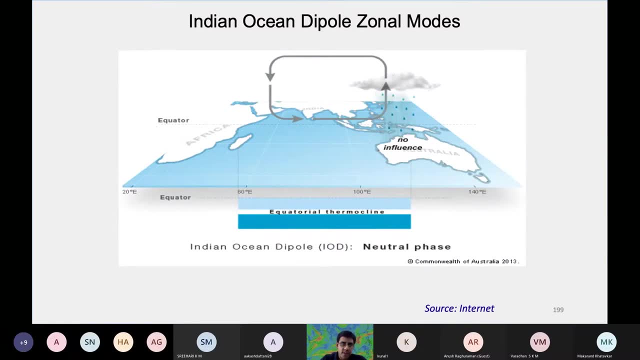 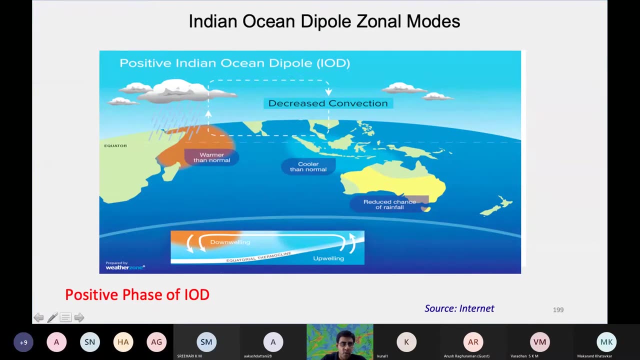 So negative phase of IOD is mostly favorable for Australian region and thereby Indian region gets a deficit. Okay, So then you have the positive phase of IOD, where during the positive phase of IOD what happens is the West Indian Ocean or the Somalian region becomes warmer. 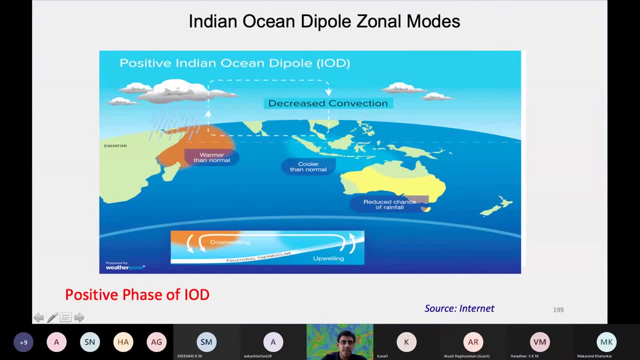 So then you have the positive phase of IOD, where, during the positive phase of IOD, what happens is the West Indian Ocean or the Somalian region becomes warmer than normal, and this becomes cooler than normal and that drives a strong walker circulation cell that gives a lot of rain to the Indian subcontinent. 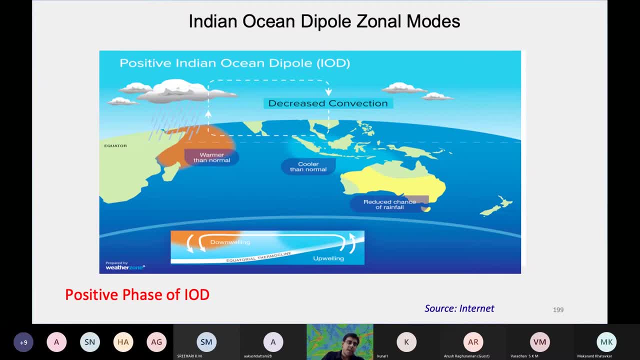 Okay, So these are the three phases that scientists have actually given and recently. what people are saying is: the Indian Ocean Dipole is a more correct representation of rainfall over India, and that is the reason why a lot of research is being done over Indian Ocean Dipole. 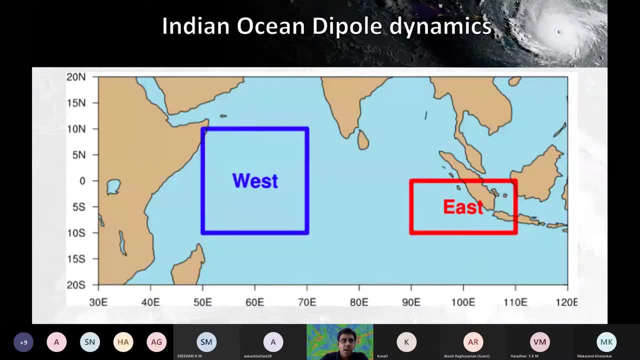 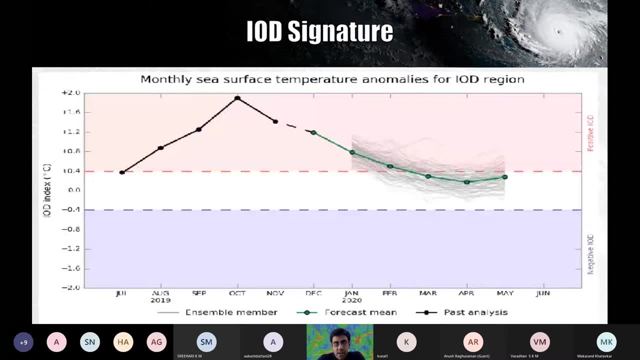 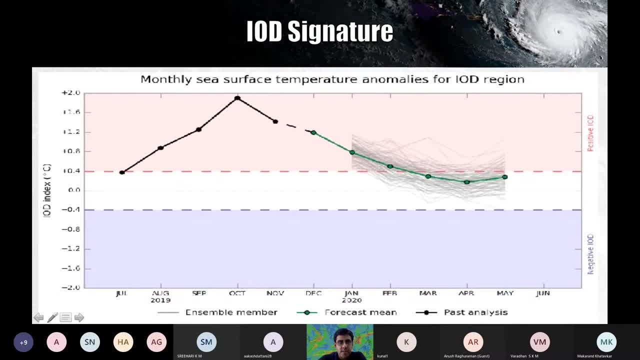 So you're on the lookout for these kind of positive IOD events, because that means that even if it's an El Nino year, the Indian Ocean Dipole will make up for it by giving more moisture from the Indian Ocean, Because previously it was thought that most of this moisture is coming from the Pacific. 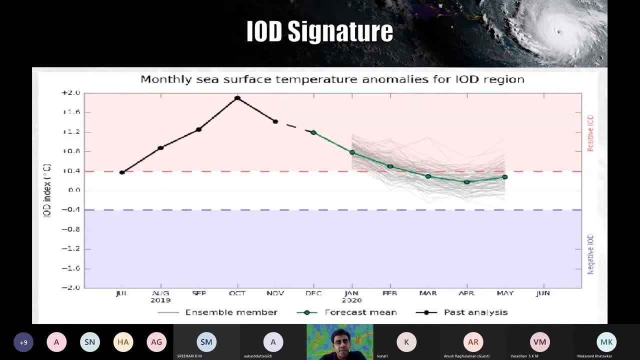 Even for the monsoon systems in India, most of the moisture is coming from the Pacific, which was true probably two, three decades back, But now the warming of the Indian Ocean has actually changed the dynamics And most of these moisture that we are talking about- more amount of moisture- is coming from the Indian Ocean compared to the Pacific. 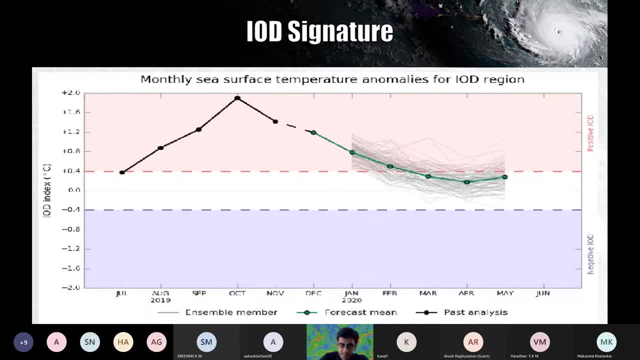 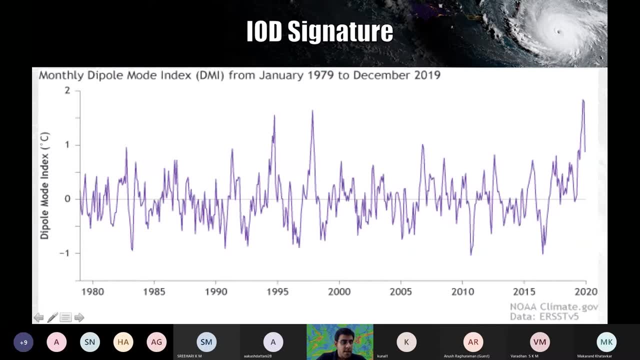 And that is one of the important aspects of monsoon which we need to embrace. OK, so what we? what we are now doing, is we are actually putting a IOD report where we see these phases of IOD which were and when this IOD peak, and when it did not. 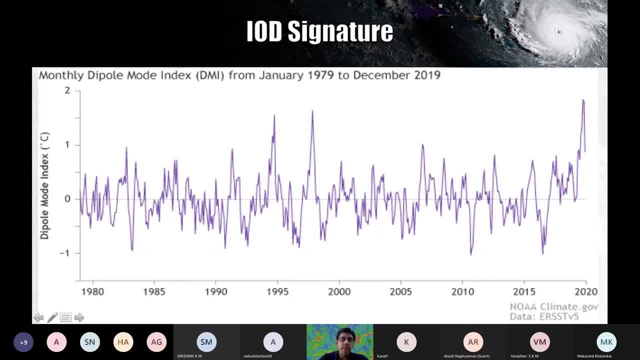 And we are actually putting together what happened during these years when IOD was very strong, And there is a very strong teleconnection that when, whenever the IOD values have been strong, which is 1994,, 1997 and the recent one, 2019,. 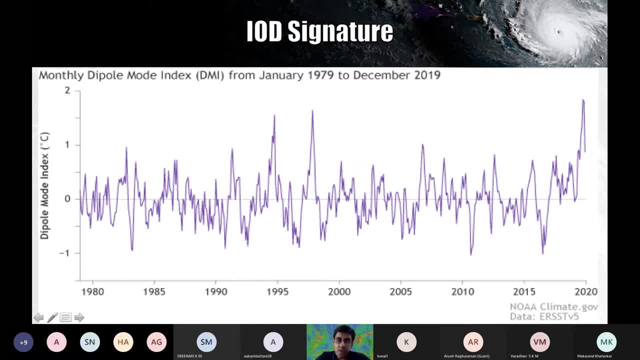 there has been heavy rainfall over India. OK, the second thing that people are seeing is negative IOD, even though negative IOD is not good for India. But when the negative IOD actually coincides with the La Nina year, then we actually have a very strong rainfall. 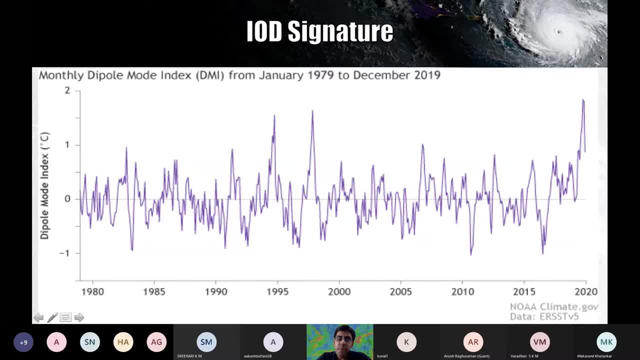 So which happened in 2012, when there was a negative IOD, But we also had a very strong La Nina year and hence it was a good monsoon year for India. And same thing in 2020: also neutral IOD, but we had a very strong El Nino, or moderate La Nina, this year. 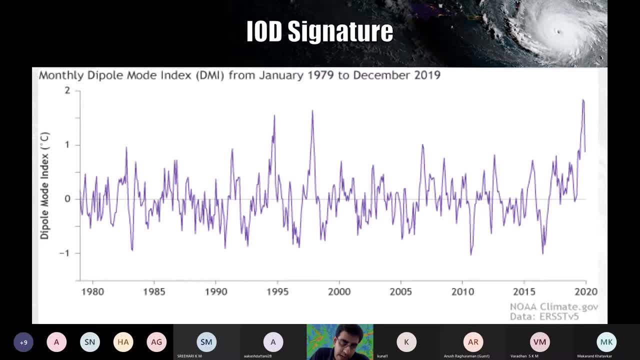 So it was a good rainfall. So what I? what we are, what I'm trying to say is that now people, and now the climate scientists, are actually putting IOD plus ENSO plus other features together to actually give the performance of the rainfall over the period of three months. 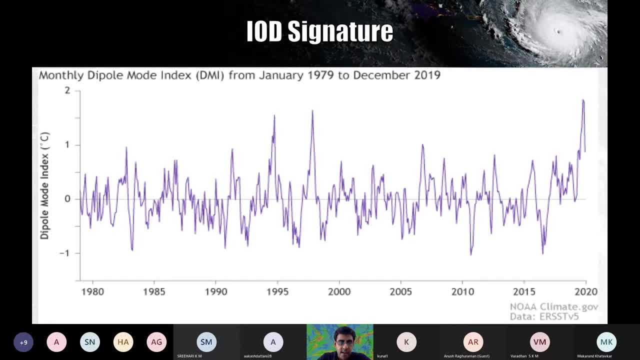 OK, and that is why revisions are being done every year, because new, new metrics are emerging for monsoon. So hence, we have to be very clear that this is not- I mean, this is still a work in progress, that the how much rain we get from monsoon is still a work in progress. 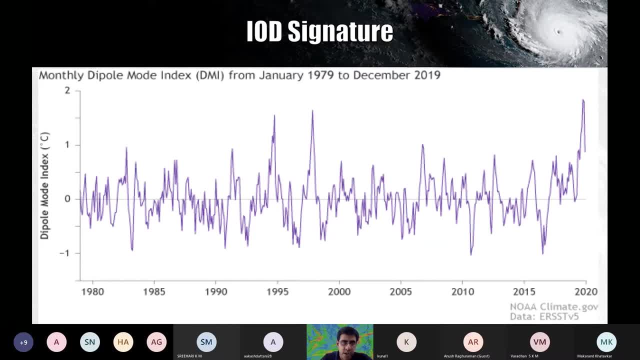 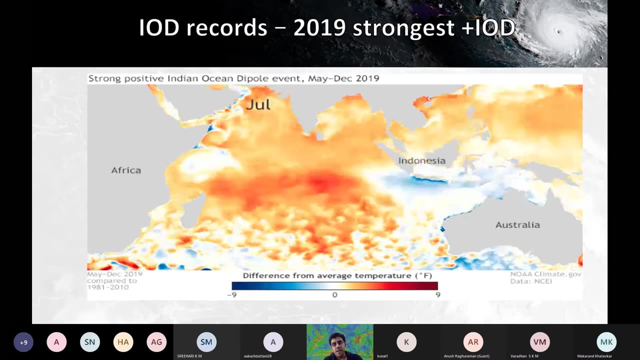 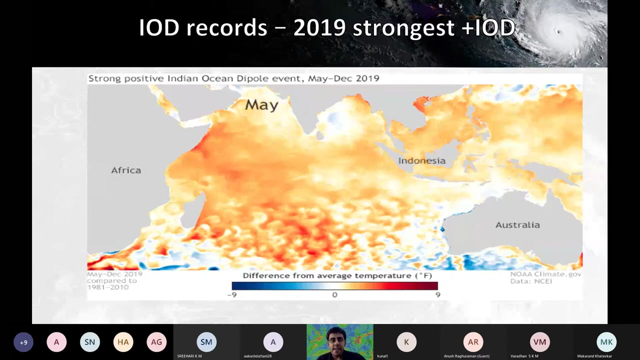 OK so, but these are the indices which one should look at before Committing to anything about the performance of the monsoon, and IMD has a very, very good handle on all these signatures and whatever they actually forecast, most of the time it happens because they look at this complete picture rather than just looking at El Nino and some of the agencies, private agencies in India. they actually have made a claim that ENSO is the only phenomenon which, by looking at ENSO, we can understand Indian monsoon. 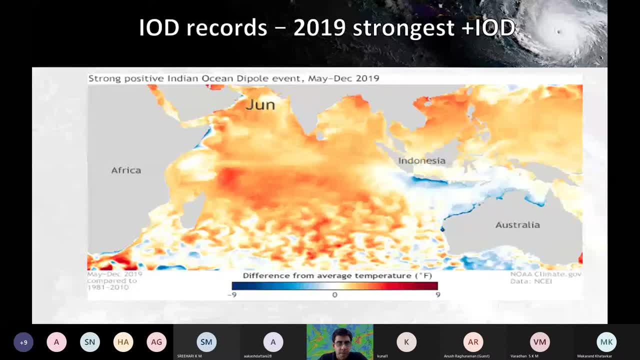 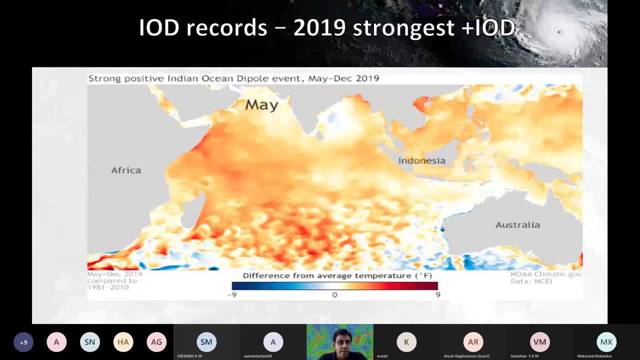 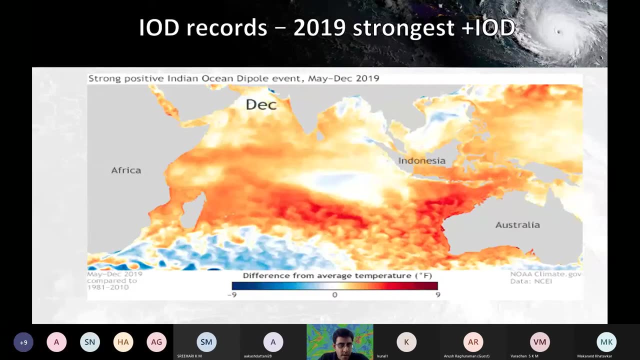 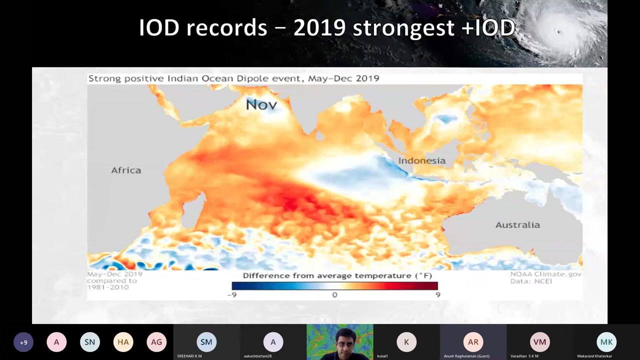 So these kind of statements are extremely dangerous because it's not true. OK, so there is. It's very important that we understand these things and we don't. I mean so. IMD has a very good handle, and that's why I think we should- we should have more trust on what IMD tells us, rather than these other private players in India- which, which, which, which, whose forecast is not as good as IMD. 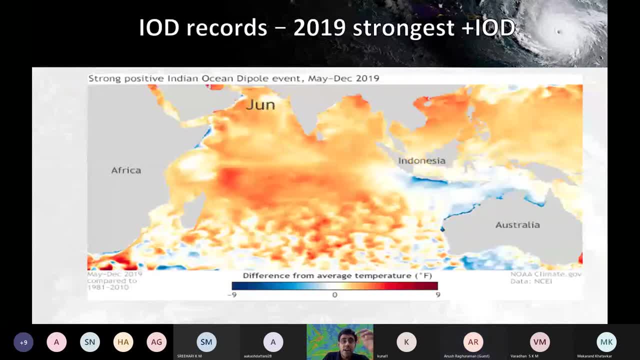 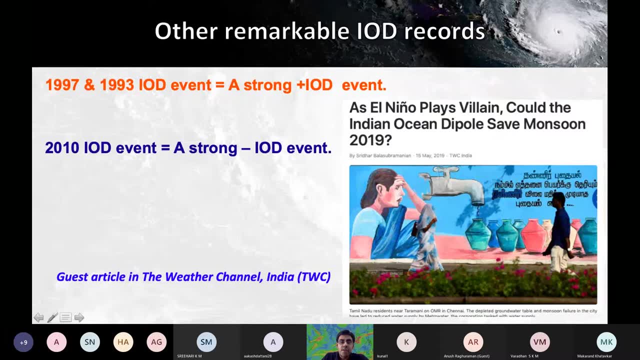 Sir, I'm just showing a 2019 record and this was one, So this was an article that I wrote for the Weather Channel. It was in May, So this was actually. this came true because 2019 was a not a very strong El Nino year, but it was a moderate El Nino year. 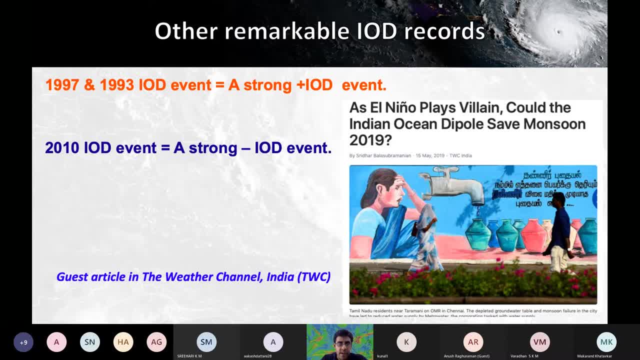 And that was a time when one of the private agencies, in February, had announced that the monsoon 2019 is going to become an Indian deficit, And that was purely based on the El Nino thing. El Nino is going to make the system- I mean make the monsoon- poor. 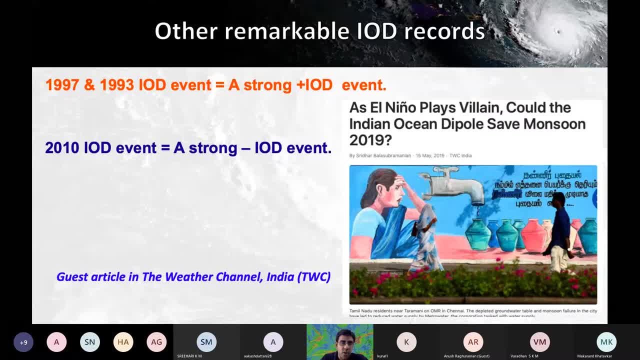 But then the Indian Ocean dipole aspect was compromised, So it was completely ignored, And this is when I thought that it's important that we we tell them. I mean, this kind of information should not be proliferated. So then I introduced this idea of Indian Ocean Dipole in an article and it ended up that 2019 actually ended up as a positive, very strong Indian Ocean Dipole here. 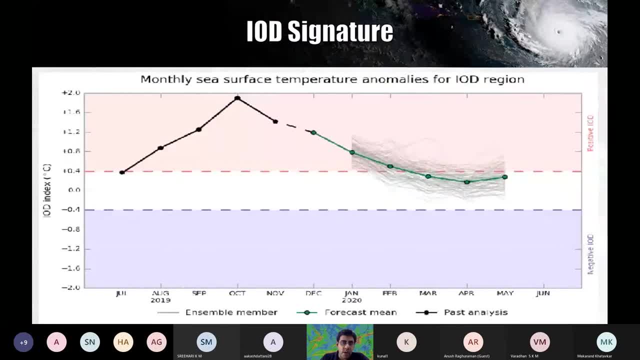 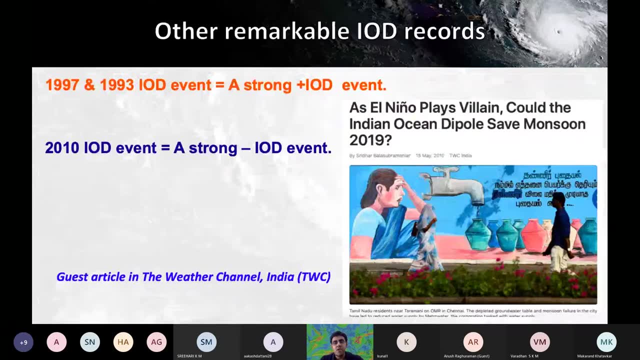 And these kind of metrics that I talked about actually help us in understanding how IOD is going to develop, And if you're on the lookout for these signatures, Then you can actually make a decent prediction about monsoon. So, although it was, I mean IMD and many other weather bloggers predicted that 2019 would end up as a normal year, which is 100 to 105 percent, but it ended up in 110 percent. 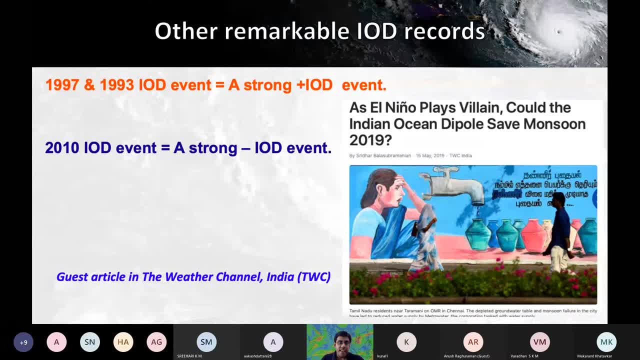 But still that is good, because what I'm trying to say is saying below normal and getting excess is bad than saying normal and getting excess. So because when you say below normal, then there is this, there is this farming community, There is this agricultural community in India becomes- I mean there is a negative thing that sets and sets, I mean gets set in their mind and it's not actually very good. 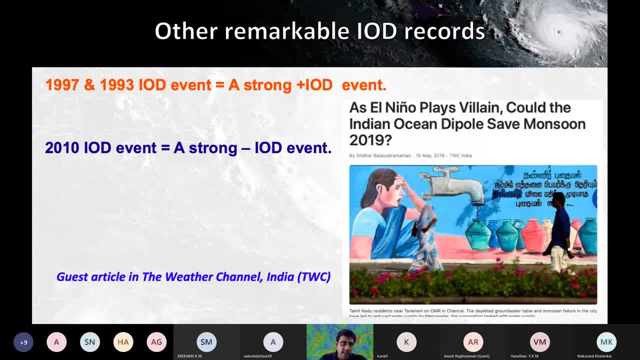 So we have to like, we have to give a decent forecast and the most likely forecast, looking at all the pitch, all complete picture, rather than only looking at El Nino. So this is the whole. the whole reason about this particular model was to tell you that El Nino is not the only thing that actually governs the monsoon. 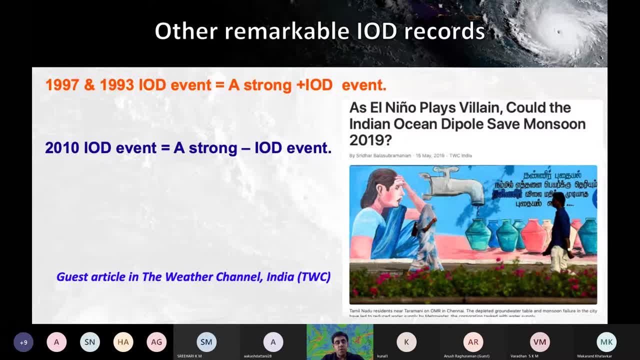 There is Indian Ocean Dipole, There is also the Indian Ocean surrender in the Indian Ocean, And so I, on top of that, there is also this monster circulation, which is very local to India, which we don't understand very kids. that circulation, we don't understand it very well. 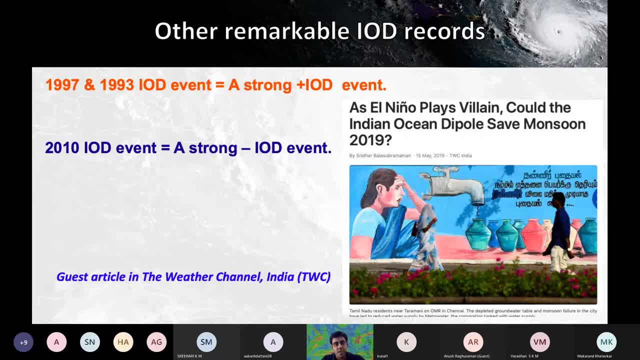 So these three things are the ones we should actually pay attention- And so are you- and how the monster circulation cell actually sets up. And the setting up of this monster circulation cell is actually related to the Siberian cooling that I talked about, the Tibetan plateau heating that I talked about, and how the jet stream moves up. 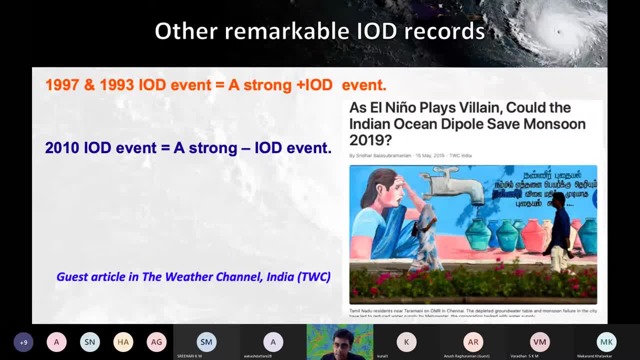 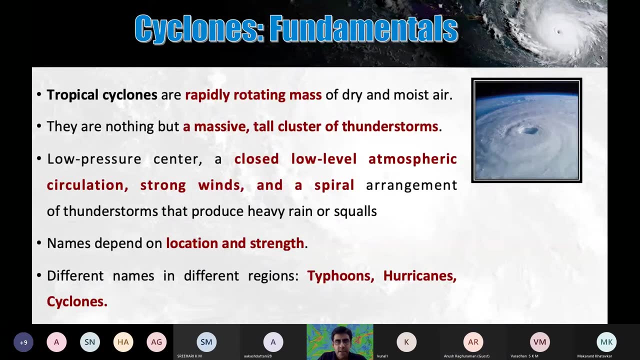 framework and then only a nice forecast about monsoon should be given, which imd does, i know. i know for a fact, because the reports clearly mention that. okay, so any doubts? before we have a very quick session on cyclones and then i want to spend at least half an hour talking about monsoon. 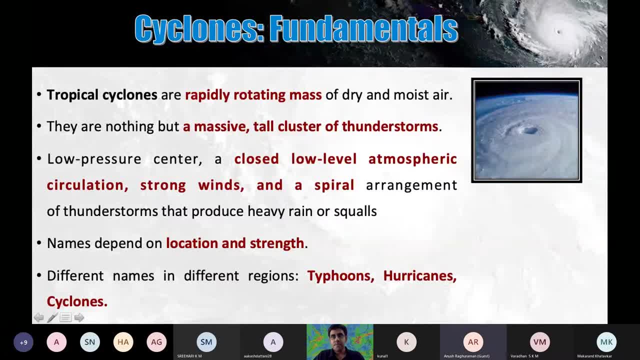 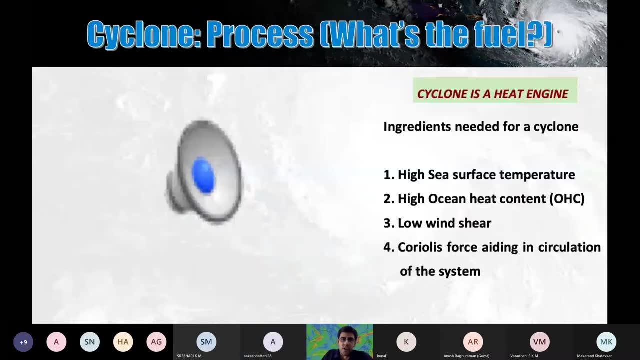 um, sir, okay, so i mean. so cyclones, we we know that they are rapidly rotating mass of air and there are different names. so the only thing that i want to ask questions on the end- so what are the? what is the fuel? okay, so what is the fuel for a cyclone? so the main fuel for a cyclone? 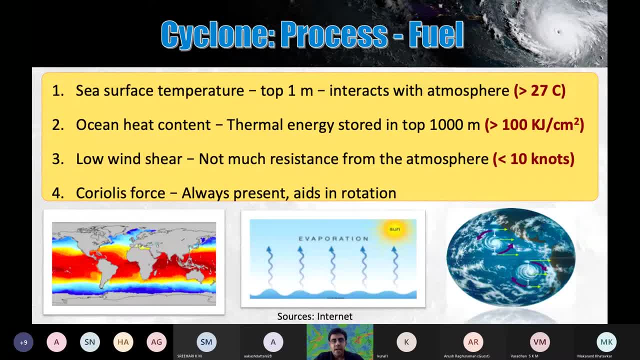 is the sea surface temperature, which is 27, which should be greater than 27. actually, 28 degrees is what now? uh, we are, we are, we are saying it should be greater than 28 degrees. the ocean heat content should be, uh, greater than 100 kilojoules per centimeter squared. this is measured as the energy stored in the ocean. 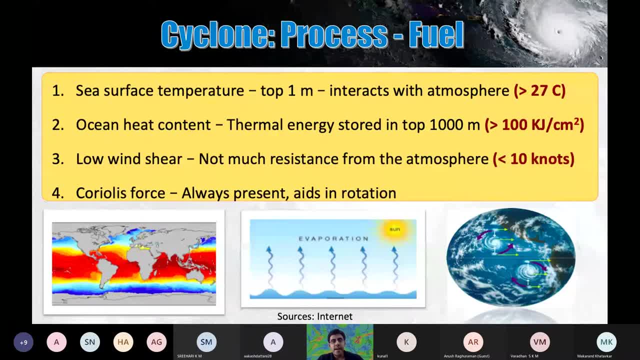 in the top thousand meters. uh, how it how it is done. it is done, uh, using, uh, the data that we have up to 100 meters and then the next next few meters. we know that ocean is in a quiescent state, so we don't take that much into account, but the thermal energy stored in that 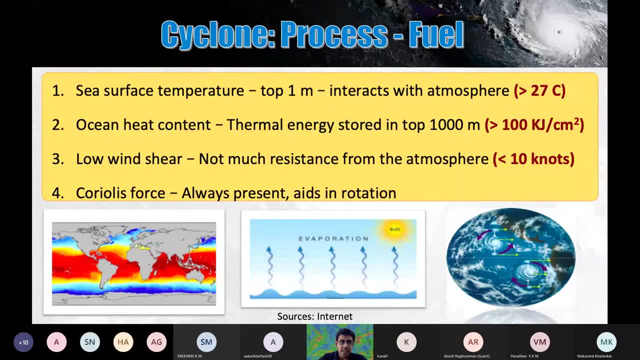 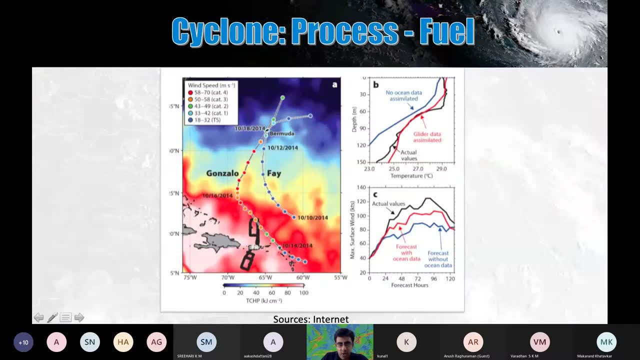 top 500 meters is very important because that is what is going to give energy to the atmosphere: low wind, shear and the coriolis force. these are the four important aspects. uh, so there are the places from which you can actually get all these values. okay, i will show how, from where. in the after. 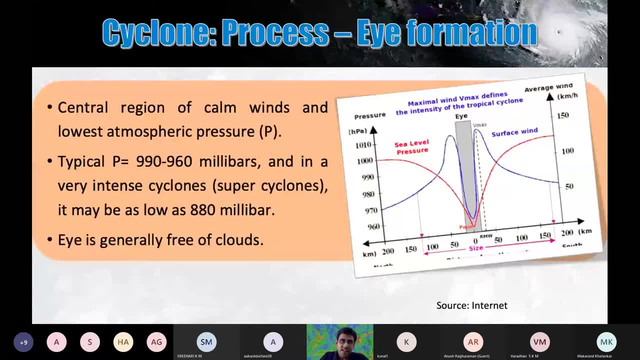 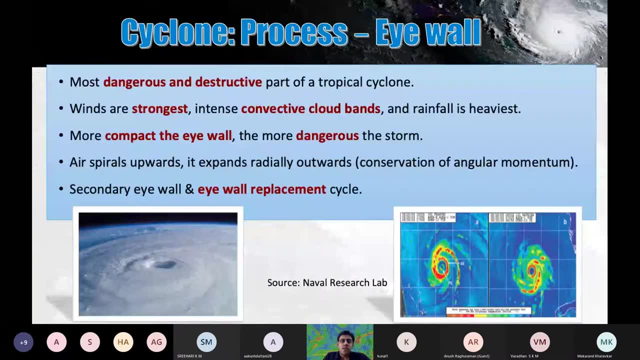 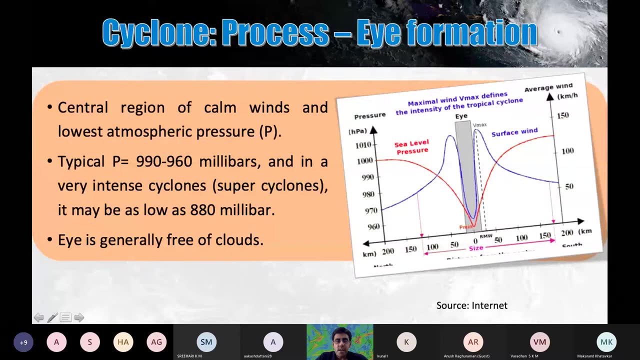 in the afternoon session. uh, it has three distinct features: i eyeball and the rain bands- so i'll just quickly touch upon them. so the eye of the cyclone is the calmest portion of the cyclone. the reason is because in the eye, whatever air is updrafted, it comes, it condenses and falls down as 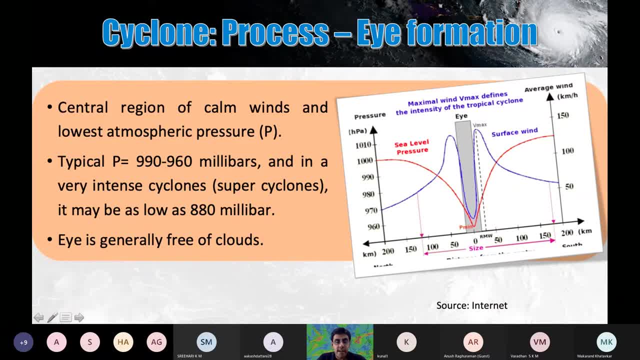 cool air. okay, so eye of the cyclone is the cleaner, is the clear and the calmest part of the cycle. but the most the, the, the, the pressure is the lowest in the eye of the cyclone. so that is, that is what is the uh is is the powerhouse of a cyclone if the, the pressure falls. 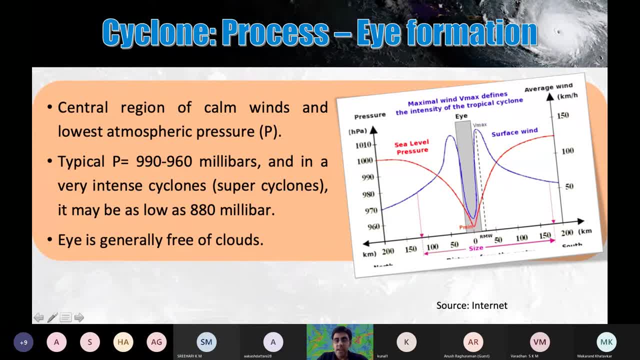 then it will actually take in a lot of moisture and it will allow updraft of the moisture. so the eye of the cyclone is mainly known for the lowest pressure, but in terms of cloudiness and winds, it is the calmest. so then the so which is very clear because we see the eye of the cyclone. 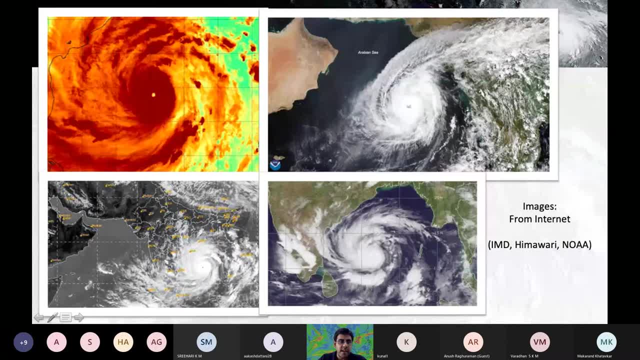 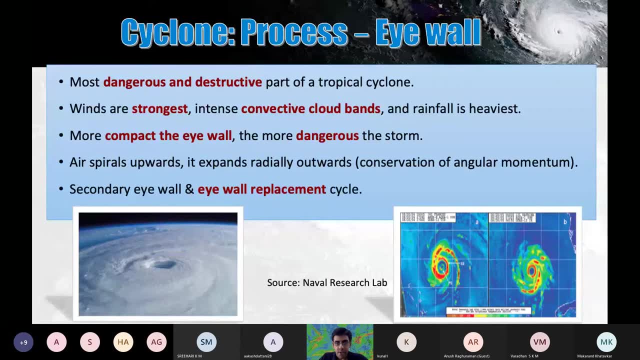 from in satellite images and then we can. then we see that it is a very clear part without any clouds. okay, so the most destructive part of a cyclone is the eye one that is the most dangerous part of the cyclone. uh, we all know why: because in a very slightly more lackluster moment of time its more. 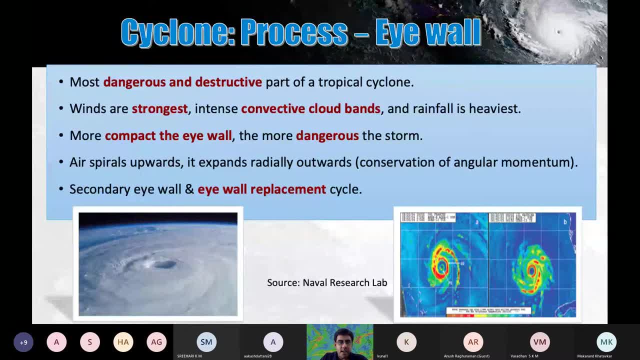 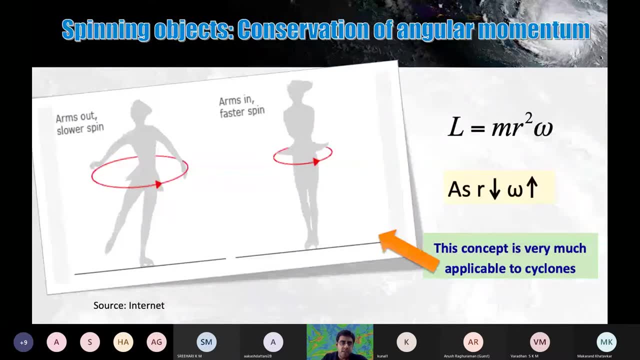 We all know why: because it carries the strongest convective bands and it has strong winds. And more compact the cyclone, more dangerous it is. Again, you can prove it from the conservation of angular momentum: If it is more compact it will rotate very fast. 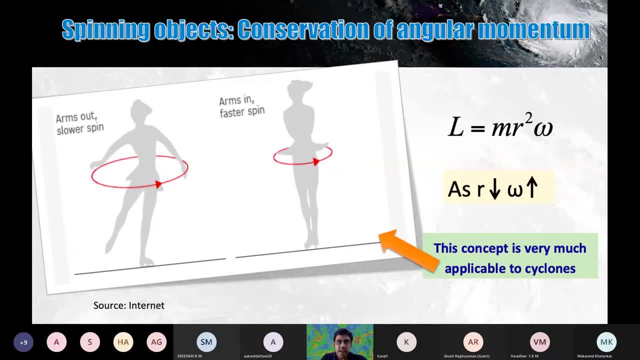 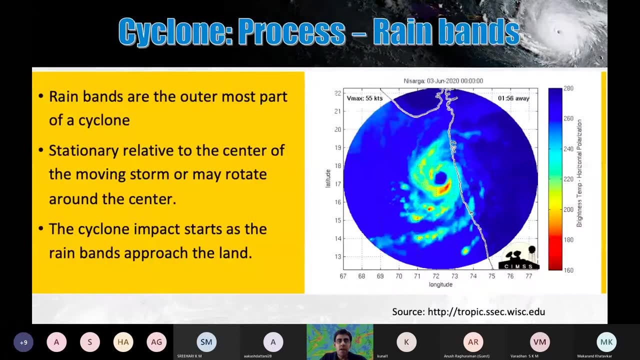 And rotating very fast means it will actually have high vorticity, And high vorticity means it will take in a lot of moisture And it has the capacity to become a very strong system. So this is something that I wanted to put in the life cycle of a cyclone. 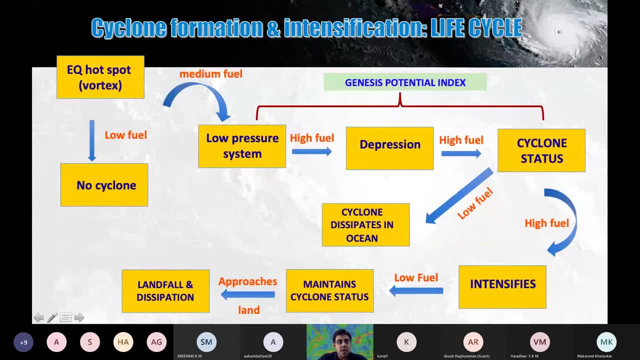 All these cyclones start as an equatorial hotspot, very close to the equator, So they start off as a vortex. So what is this vortex? It is a disturbance. It is a disturbance, So it is very similar to a wave. 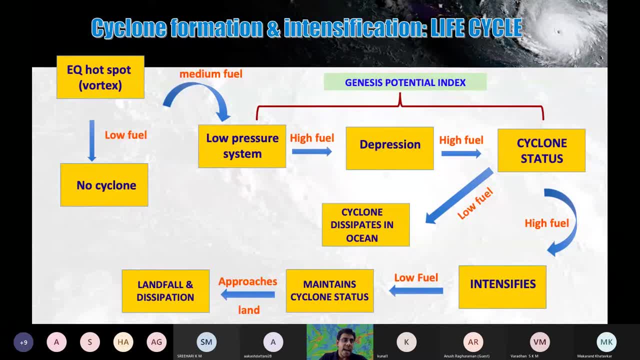 So a wave has passed by in some region of the ocean. Can it create that vortex in the ocean or in the atmosphere Just one meter above? If it has created that, then that is the starting point for a cyclone. And if the fuel is high, the fuel is basically the sea surface temperature, the ocean heat content, the wind, shear and coriolis. 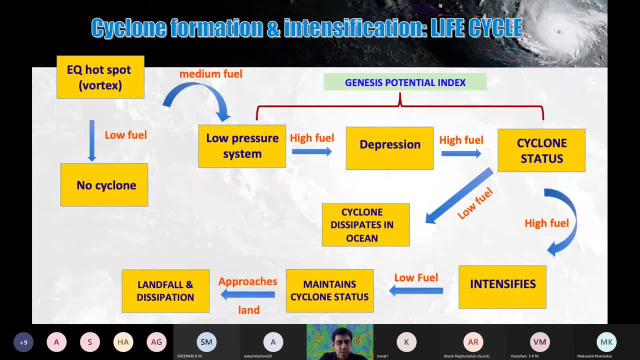 Coriolis is always present, So we do not care about the coriolis. So if other three things come into picture, then that particular small disturbance that is present in the ocean will become a low pressure system. That low pressure system, if the fuel is maintained it will become a depression. 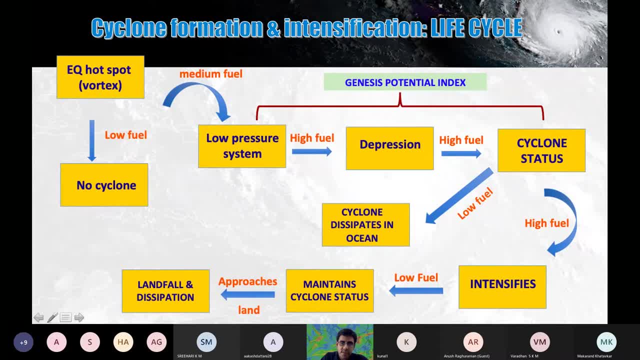 And then it will become a cyclone And this fuel, if it is sustained for this long period of time, that is known as the Genesis Potential Index of a cyclone. So for the Genesis Potential Index, the vortex, a hotspot, should be there, followed by the fuel, which takes it to a cyclone level. 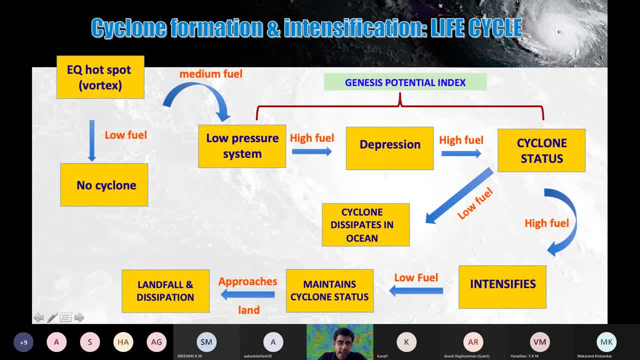 Once it goes, then if the fuel is present, then it will intensify and then it will maintain a status and then approach land and dissipate. So what we are always on the lookout for is we are on the lookout for water. 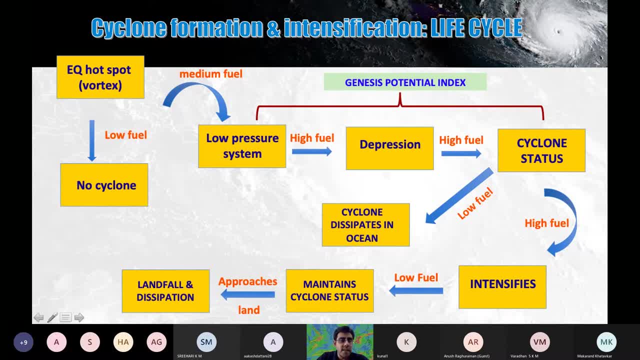 For MJO, which has the capability to plant this seed. We are on the lookout for MJO. We are on the lookout for wave action, which is Rossby wave most of the time We are on the lookout for. So these are the two things. 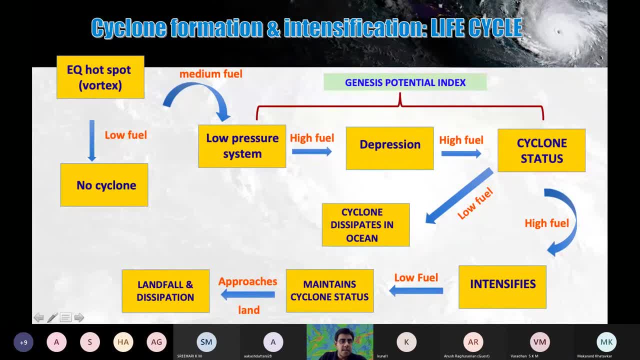 MJO and Rossby waves are the things which can actually put in this seed which is required for cyclone formation. After that, if a seed has formed, then we are on the lookout for these other, These parameters, like the ocean heat content, the ocean temperature and the wind shear. 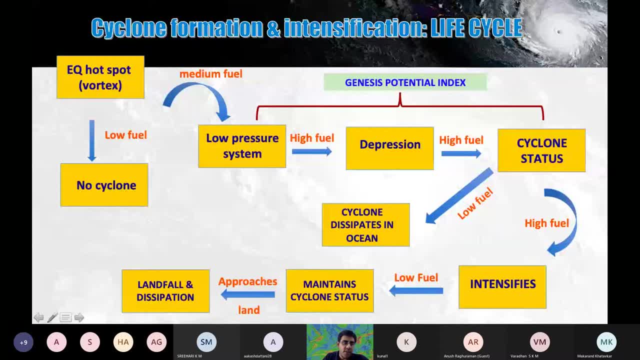 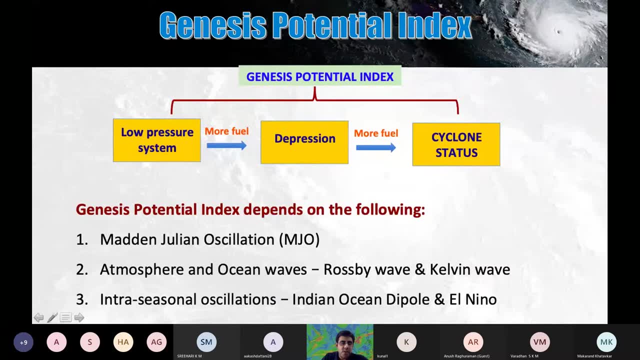 when to see if this particular seed can become a cyclone or it will die off as a low-pressure system. So that is what is the Genesis Potential Index. Like I have written here, the Genesis Potential Index of a cyclone is gauged by MJO and the wave action. 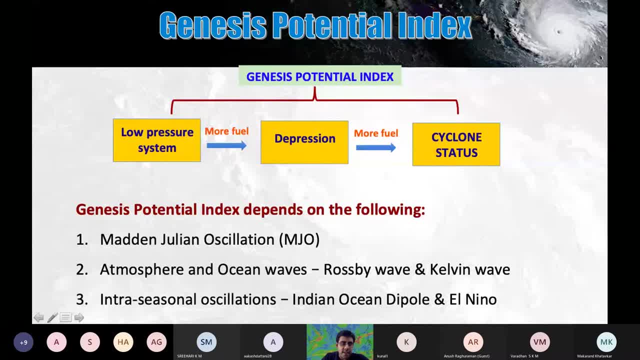 And sometimes it is also gauged by the intra-season oscillations, which is kind of the Indian Ocean, Dipole and El Nino, But I am- I am not going to touch upon that because that's a little bit more complicated, but these two are, most of the time, the things. 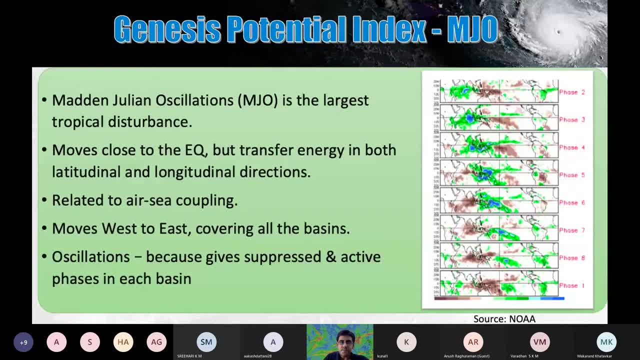 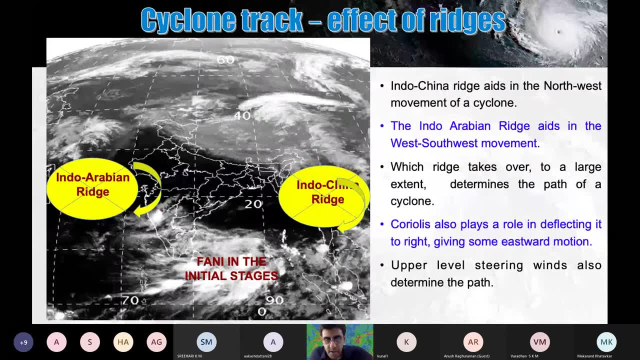 that actually plant the seed for formation of the cyclone. So let's say, the cyclone has formed. Once the cyclone has formed, how do we track the cyclone? So that is a very important aspect, because I know how a cyclone forms. So then 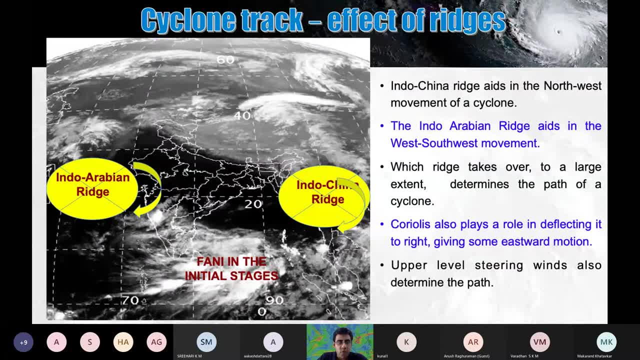 I need to find out how the cyclone is going to move. So the movement of the cyclone is governed by these two things, which is the Indo-Arabian ridge and the Indo-China ridge. So there are two ridges. So ridge is nothing. but at the 300 millibar chart you will see. 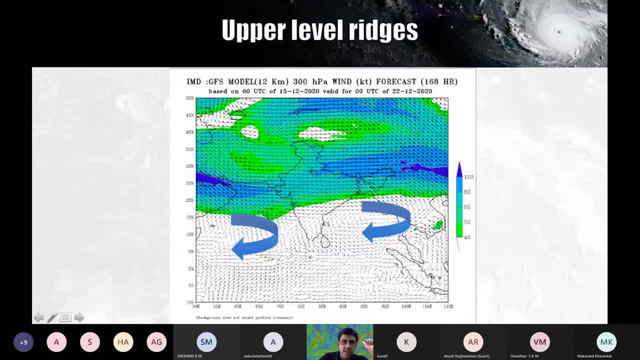 a high-pressure system. So this is the ridge. So if you look at the GFS, IMD, GFS output, you will see that at 300 millibar or 300 HPA level I see these two anticyclones which 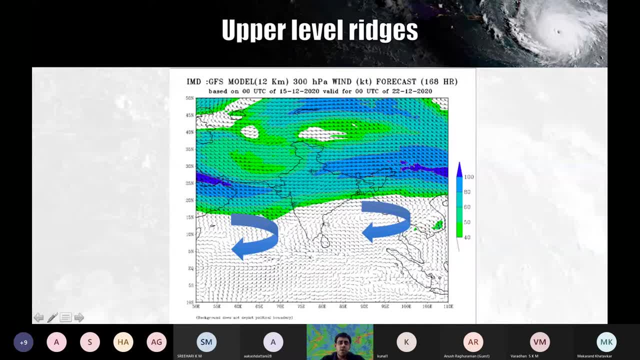 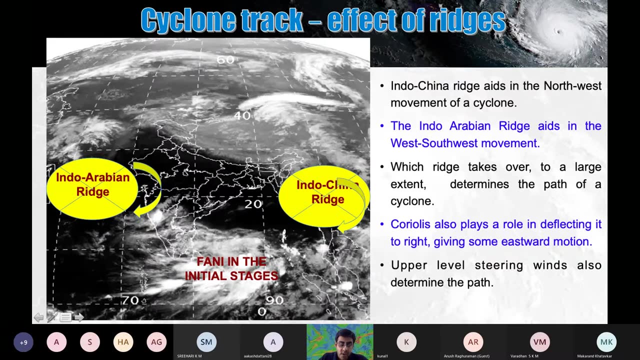 are high-pressure zones. Okay, So these two zones, these two high-pressure zones, are going to govern the track of the cyclones, because cyclones tend to move along the ridges. Okay, Cyclone tends to move along the ridges. So this Indo-China ridge is the ridge which actually gives the cyclone its 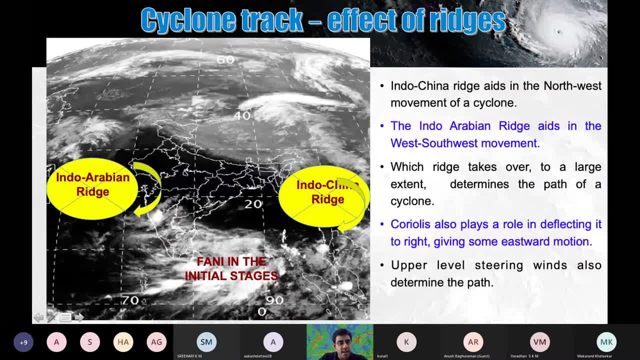 northward track And this Indo-Arabian ridge is the ridge that gives it the westward track. Okay, So when a cyclone is governed by the Indo-China ridge, then it it can, it has to move north. That is why, during April- May, most of the cyclones move up north, because 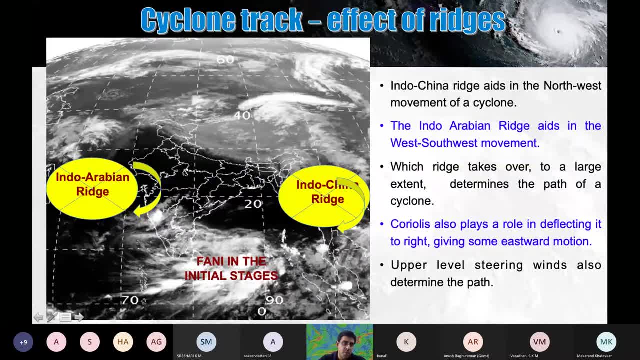 they are governed by the Indo-China ridge, So either they go to Odisha or they go to. they go to West Bengal or Bangladesh or Myanmar. Indo-Arabian ridge is the ridge that actually takes most of the cyclones away from the Indian coast towards Oman or Somalia. Okay, So maybe 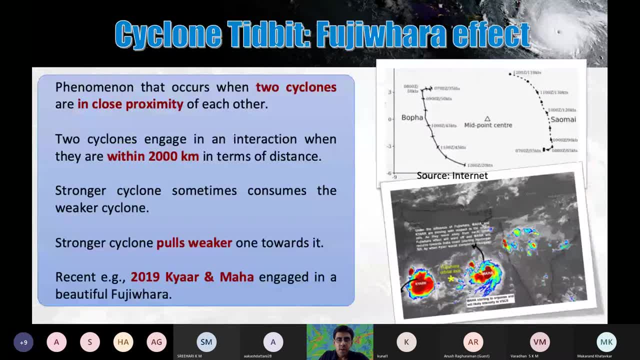 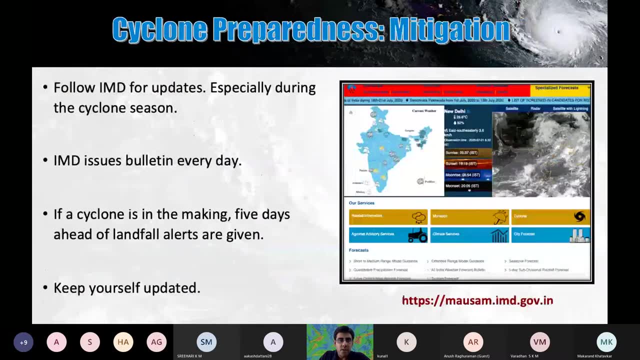 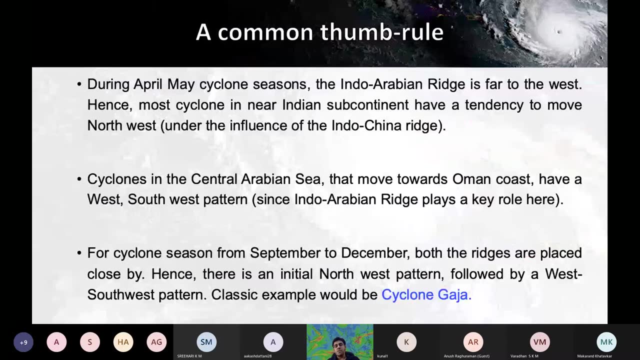 I will. there are a lot of things I just wanted to talk about, but maybe I will skip these things and I'll just come to one point again about these things. you can read up, because I'll be sharing it anyways. You can read it up: A common thumb rule. This is something. 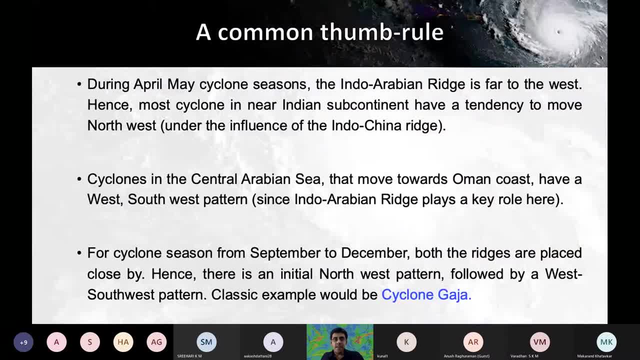 important because if you are interested in tracking a cyclone, then this is something that may come handy. This is what I have observed, So during April and May cyclone seasons. the Indo-Arabian ridge is far to the west, Okay. 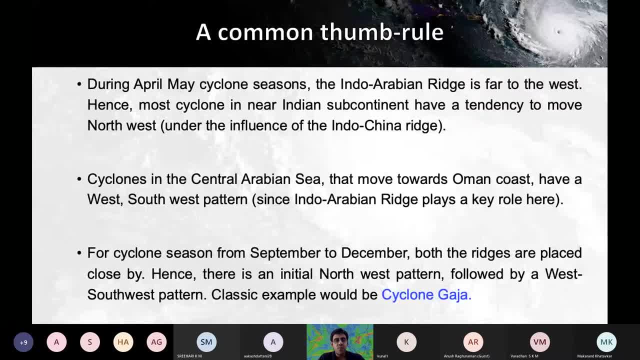 Hence most of the cyclone that form near the Indian subcontinent. they have a tendency to move northwest under the influence of Indo-China ridge. So during the April- May seasons Indo-Arabian ridge doesn't favor very much. It is the Indo-China ridge that governs the 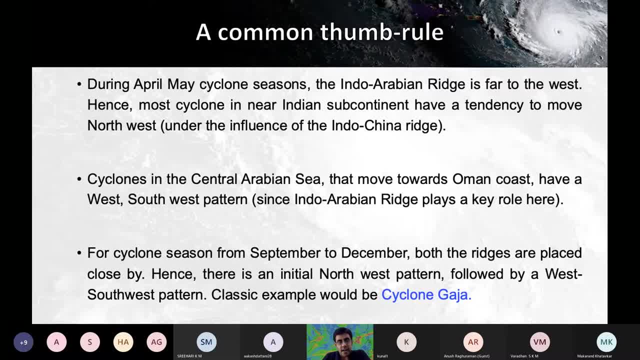 cyclone, and hence they have a northward track. Okay, Or north westward track. On the other hand, the cyclones that form in the Arabian sea during April and May, they move towards Oman coast because they are governed by the Indo-Arabian ridge. 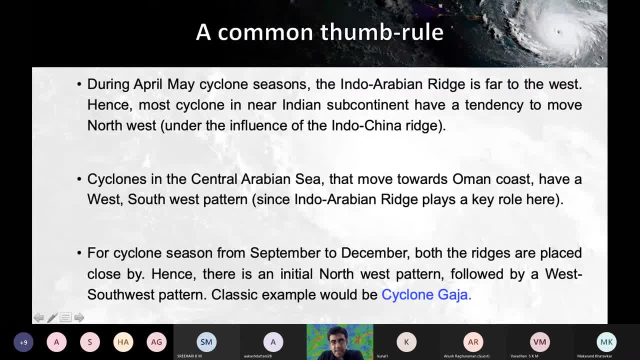 However, if you look at the September to December season, then both the ridges are close by, So they are very near to India And hence most of the time what happens is they initially have a northwest pattern and then they have a west-southwest kind of a. 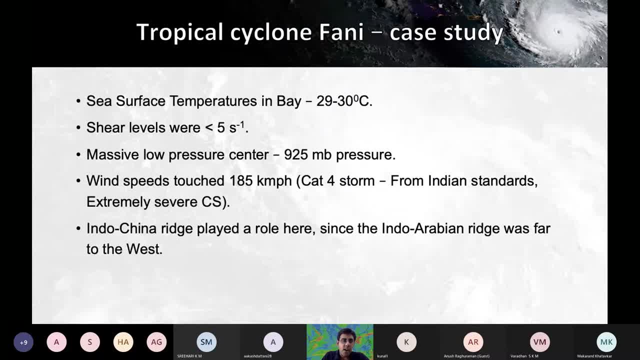 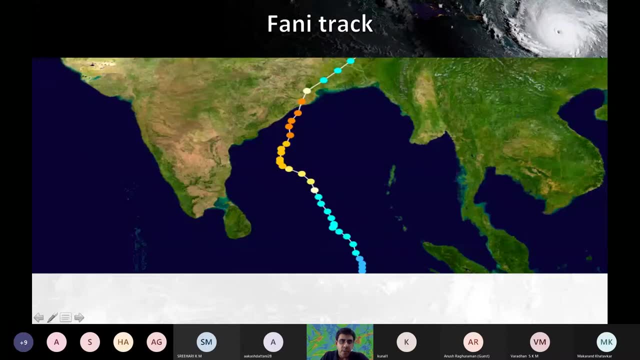 pattern. So I'm going to take two examples: Cyclone Sunny, which was a category four cyclone, extremely severe cyclone. The Indo-China ridge played a very important role because the Indo-Arabian ridge was far away, Okay. And then Cyclone Sunny had a fully northward, northwest track, So it started from equator. 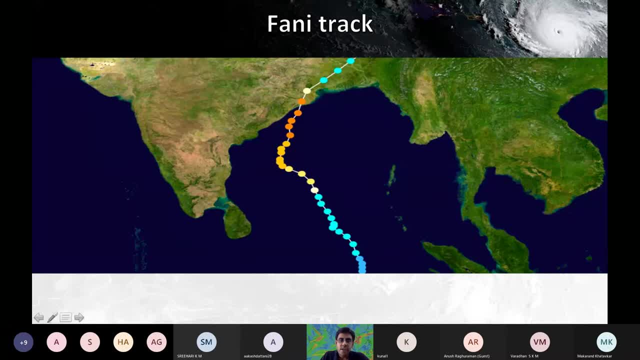 You can see it simply move towards the north. Okay, So it was fully governed by the Indo-China ridge, because the Indo-Arabian ridge was very far away. There was no influence of that. This was in May 2019.. Then you have Gaja, which is a cyclone which formed in October. 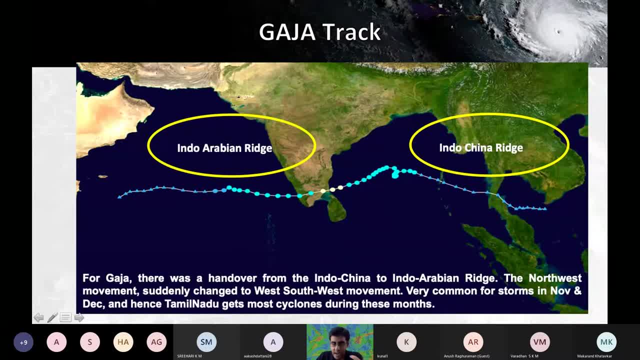 2018.. If I'm right- I'm not sure whether it was October or November, but it's okay- The both the ridges were very close to India, So initially it came as a remnant of a storm from South China Sea And initially it was governed as a northward track, which was due. 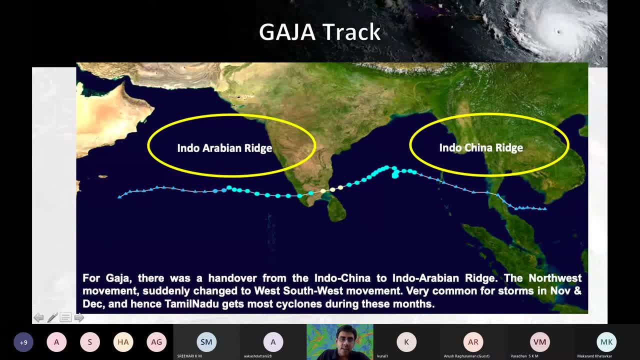 to the presence of the Indo-China ridge, And then there was a handshake between the Indo-China ridge and the Indo-Arabian ridge because this Indo-Arabian ridge was also present. So the cyclone kind of waned its influence of Indo-China ridge and now started to get influenced by 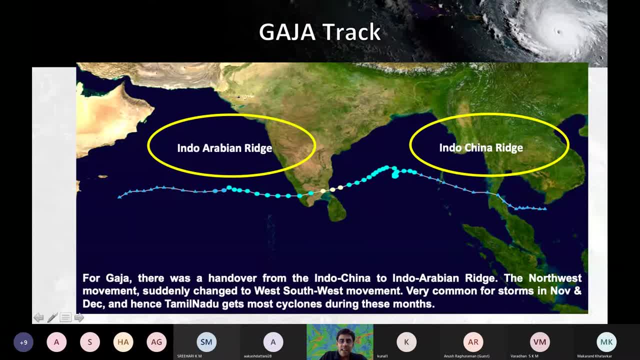 the Indo-Arabian ridge. And the interesting thing about Gaja- which is something even I don't know why it was- it stood in this region for 24 hours and it made a circle, So you can see that there was an inertial loop. It simply made a circle here before. 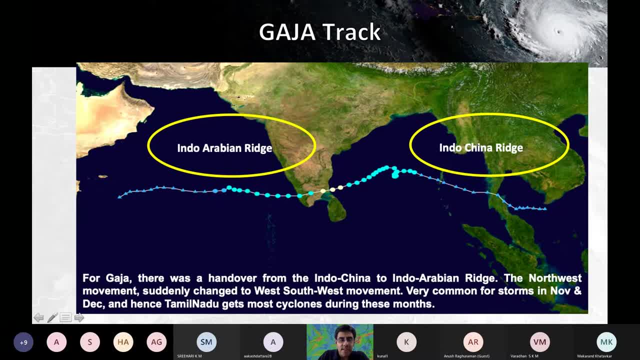 it was completely governed by the Indo-Arabian ridge. And then after that, once it was governed by the Indo-Arabian ridge, it just kept moving towards India, Okay, Towards Somalia. So it was fully a full west-southwest track. You can see that it is not moving north. 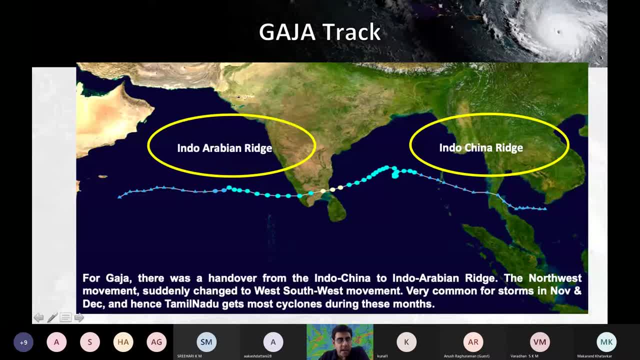 it is moving west. So Indo-China ridge usually takes cyclone to the north and Indo-Arabian ridge usually takes cyclones to the west. So this is something which is very important And during the April-May seasons Indo-China ridge is very active because Indo-Arabian 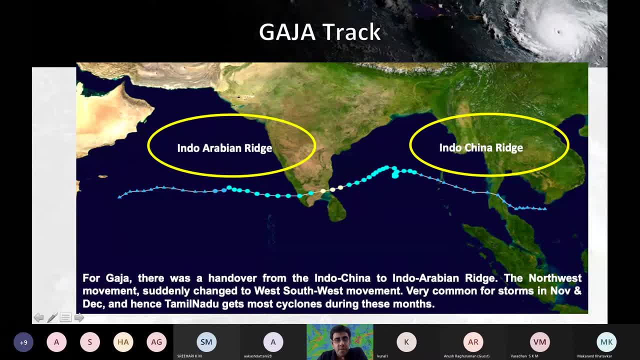 ridge is very far. However, during November and December, both the ridges are very close by And hence most of the cyclones move towards India, And so the cyclones they. Varda also had a very similar track, where it just came flat. 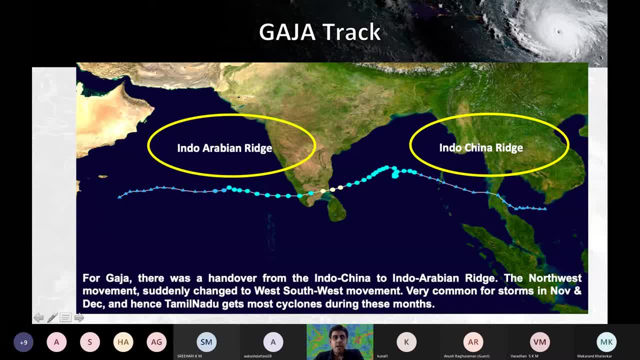 Okay, Because it was fully governed by the Indo-Arabian ridge. Okay, One other thing is, if you talk about Cyclone Niwar, Cyclone Niwar didn't follow a westward pattern, it moved north. It had a north-west pattern. The reason is because Cyclone Gati 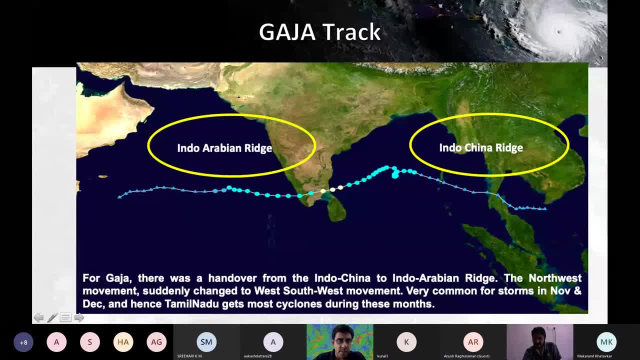 was forming at the same time and Cyclone Gati ensured that this Indo-Arabian ridge moved away from India. So Cyclone Niwar was kind of governed by the Indo-China ridge. Okay, Again, it was a very different pattern. Okay, I said that it was very common for 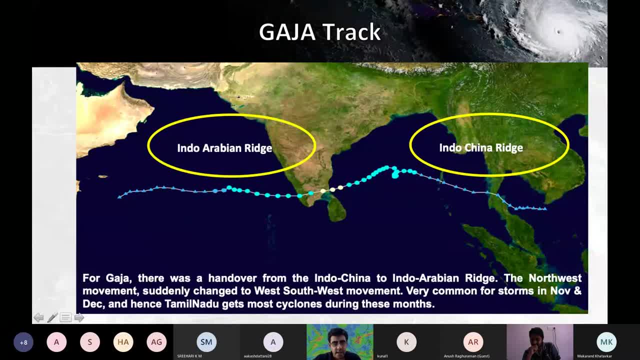 storms in November and December to move to have this kind of a pattern. But there can be some differences, because if a cyclone forms, if there are two cyclones which form around the same time, then the ridge action gets very ridge action gets changed. And because 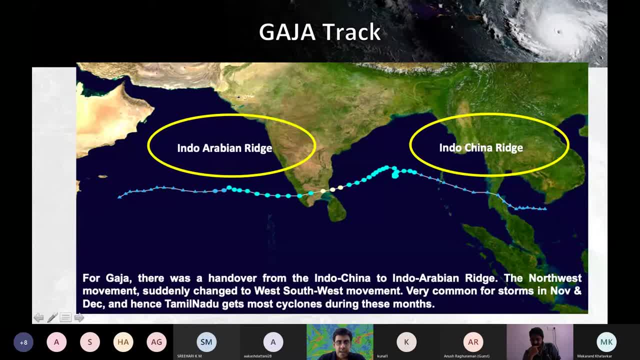 of that, your movement of the cyclones will also get changed. So that is very…. If Gati had not formed, then the Indo-Arabian Ridge would have been not formed. Okay, Okay, Yeah, nice Okay, Thank you, Okay, Thank you, Okay, Okay, Thank you, Okay, Thank you, Okay, Okay, Okay. 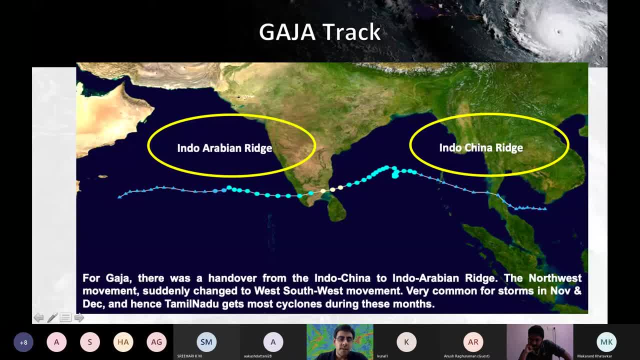 near India and that would have not allowed the system to move towards Pondicherry, but it would have moved it to. it would have allowed the system to move more towards southern part of India, southern part of Tamil Nadu. A question about Karnivar and Biravi. 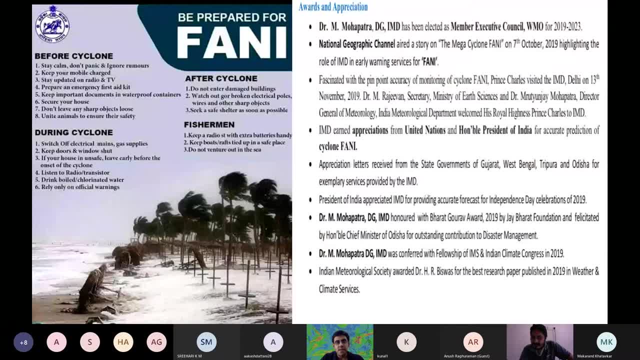 We have a very good track record of cyclone prediction. This is something that was given by WMO, which is the World Meteorological Office. India has a very, very good track record of cyclone because we understand a lot of things about cyclones, how they move, how the ridge actually. 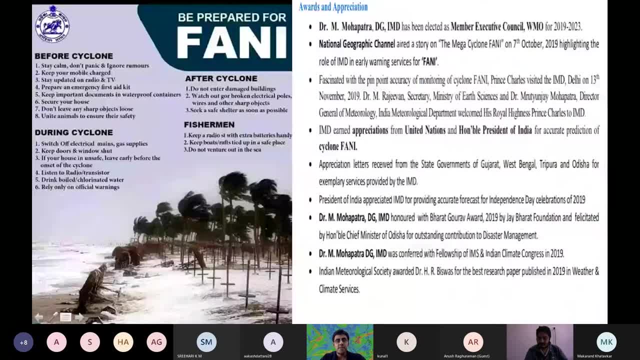 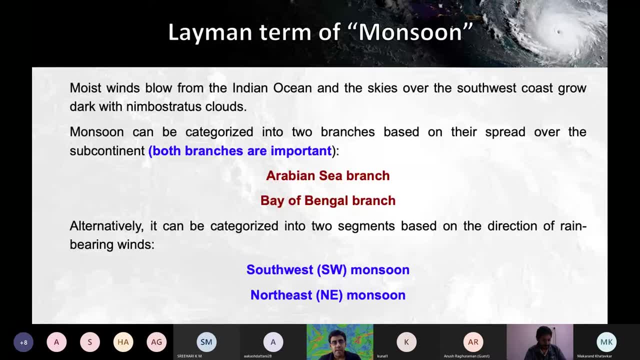 governs the movement. A lot of things we know about cyclone and hence we are- I think we are- ready for any kind of cyclone prediction, be it a very super cyclone or be it a cyclone like Nisarga. Both of them, I mean, we can predict and we are ready for. 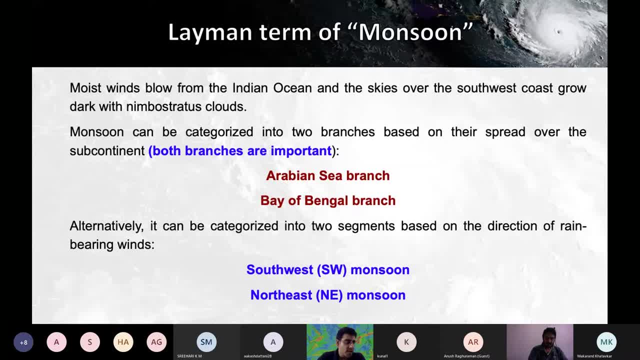 evacuation and all these things. So mitigation. So if there is any doubt I can before I move into Monsoon. There is a question? Hello, Hi, Hello, Hello, Hello, Professor Sridhar, there is a question about Nivar and Biravi. 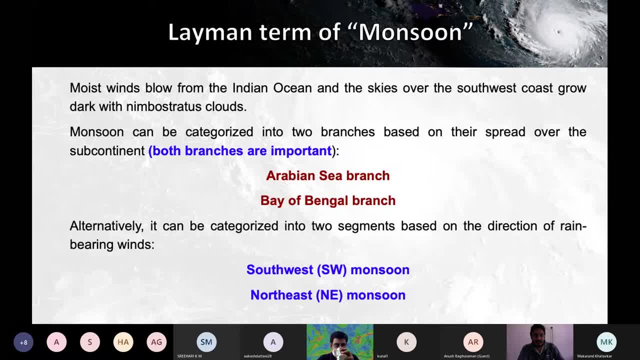 Yeah, Nivar. actually what happened was that there was some expectation of destructive winds Close to the coast, you know, because of low wind shear. But what happened was throughout the, towards the end, when it was nearing the coast, the wind shear suddenly appeared to increase. 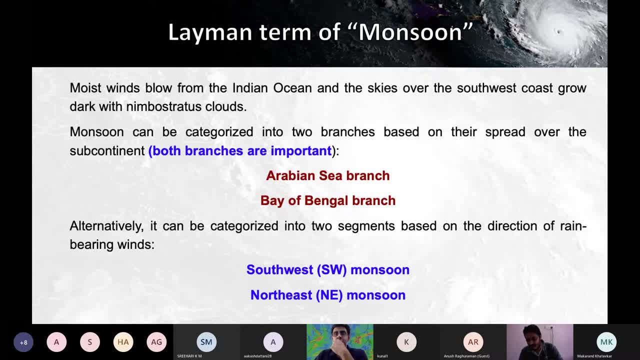 No one could have predicted that, but it was good, because in the end, we had only rains but no destruction. And also, regarding Biravi, what happened? it stayed as this, as we used to say: the uninvited guest in the Nivar Gulf of Mannar for several days, giving incessant rains to delta region. 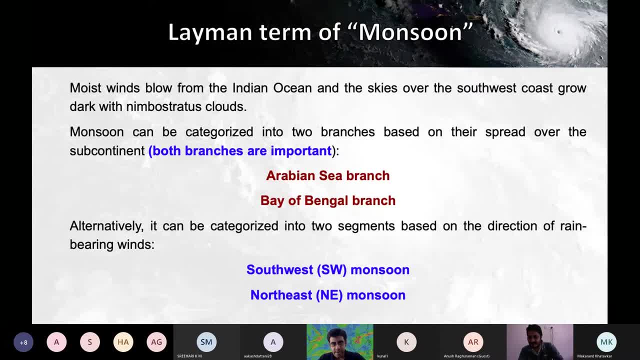 I mean the Cauvery delta region- for a long time, probably because the two ridges- neither of the two ridges- cared about the circulation and nobody took control, So it appeared to just get stalled for a while. I mean, could you comment on why? I only wanted to know why we are not able to predict. 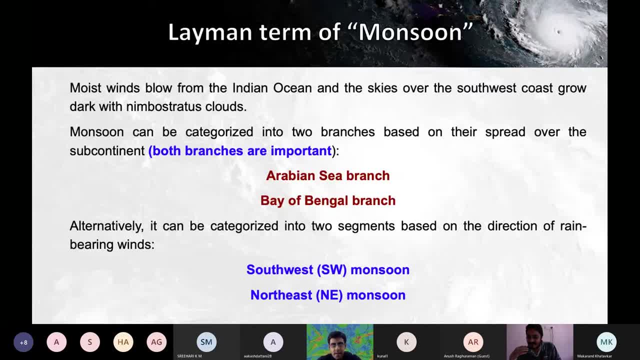 the wind shear pattern. what is going to happen next? Because you know, we were expecting that there's going to be some destruction with Nivar, but nothing happened. that's good, but at that time, just when I was tracking this for a long time and I just 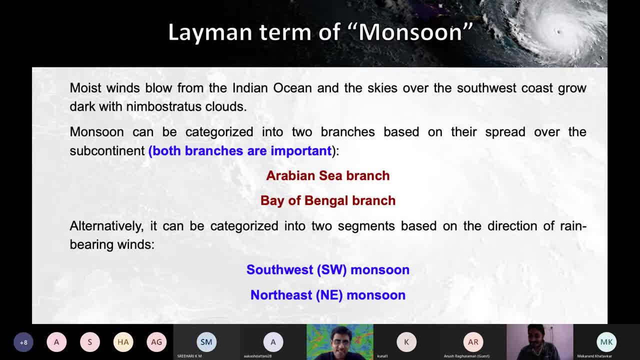 exhausted. I got exhausted and slept up. the next morning I woke up, there was absolutely no problem, Right. so that was actually expected, and I think, more than the wind shear for Nivar, more than the wind shear, it was to do with the, with the pattern of, I mean with the, with the system itself, And 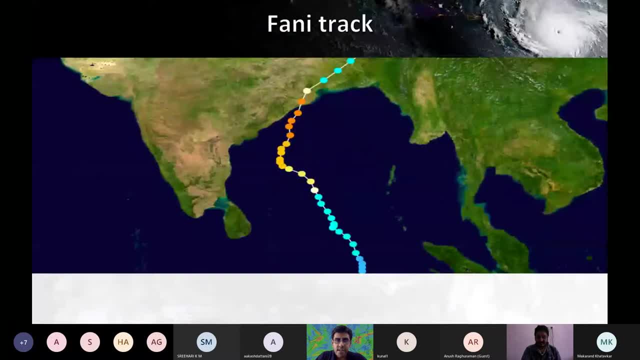 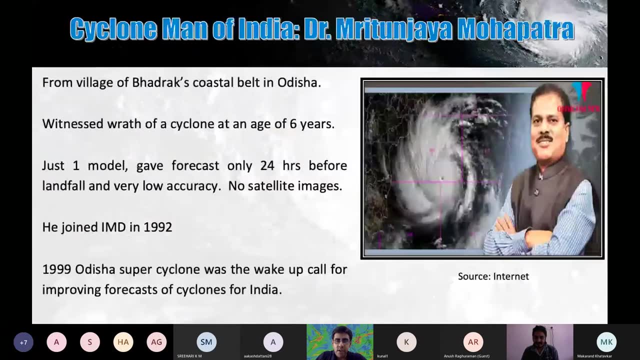 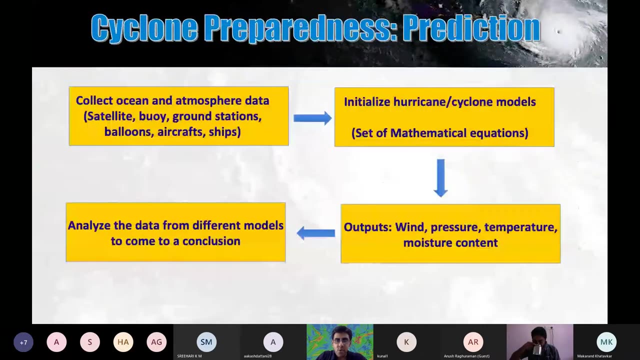 I will. I'll just focus your attention here to this particular chart. So one thing is, this particular cyclone, Nivar, was a very severe cyclonic storm. Yes, And generally very severe cyclonic storms. what they do is they, they. they usually form a very clear eye, so they become. 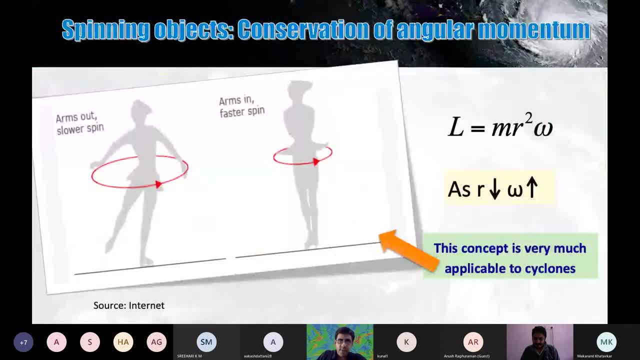 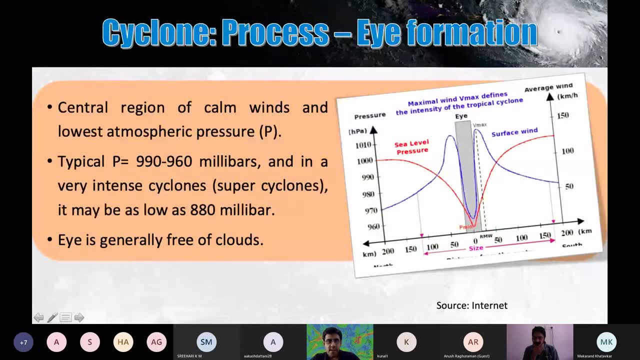 more compact and compact. But with cyclone Nivar, what happened was it couldn't become more compact, And the reason was because it was it, it kept getting hindered by the presence of topography. So first it was the north north Sri Lankan topography that interacted with the 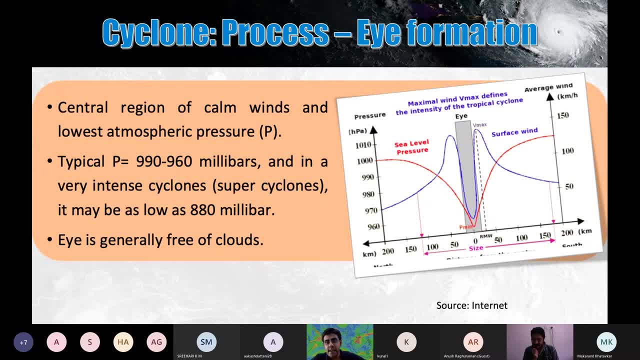 southwestern bands of Nivar and then later on it was a delta delta region that kind of interacted with the western bands of Nivar, Right. so the the cyclones, even though it's a very severe cyclonic storm because the winds were very strong at the near the eye wall. Okay, 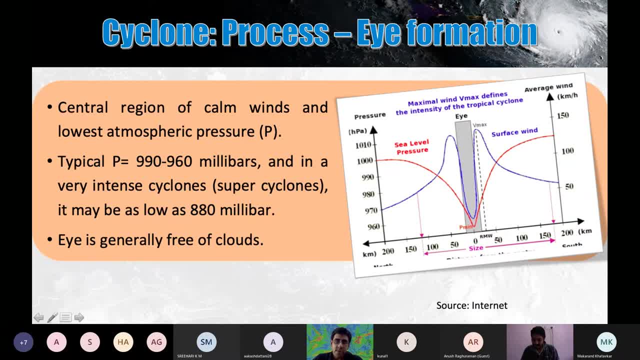 But the interesting thing about cyclones is, if you come outside of the eye wall, the winds actually drop exponentially. So this is what I wanted to show you. So winds drop exponentially. So near the eye wall the winds are strongest and as they move away, the winds drop exponentially. 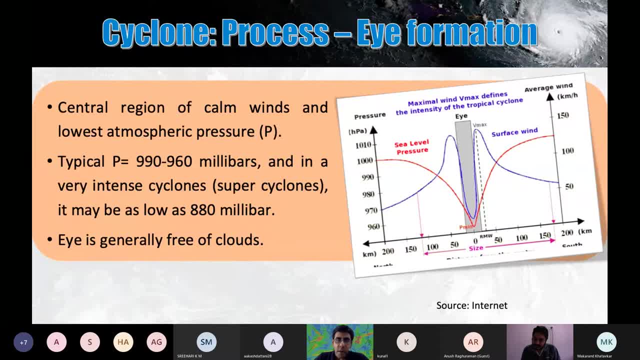 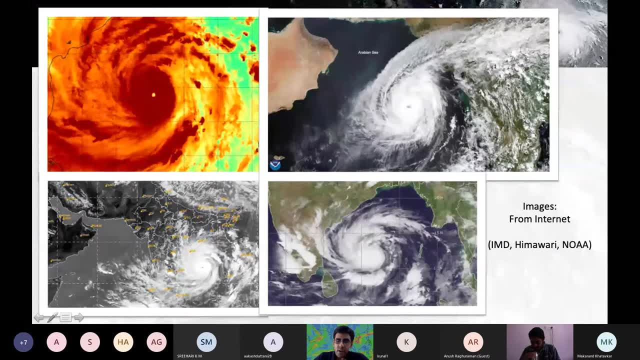 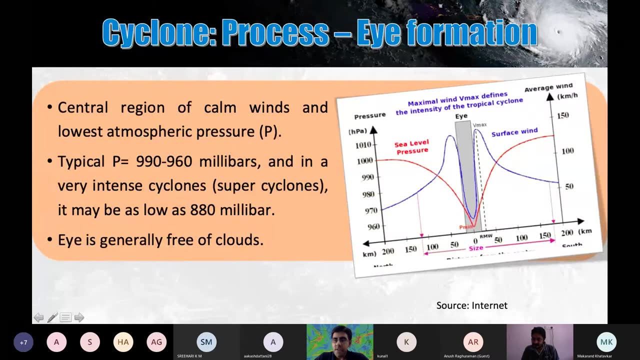 And for a, for a cyclone which is very well organized, for a compact cyclone like this, which has a which is showing a very clear eye. If you draw this particular, if you draw this particular diagram, you will see that the exponential decay is not very strong of the winds. So let us say from: 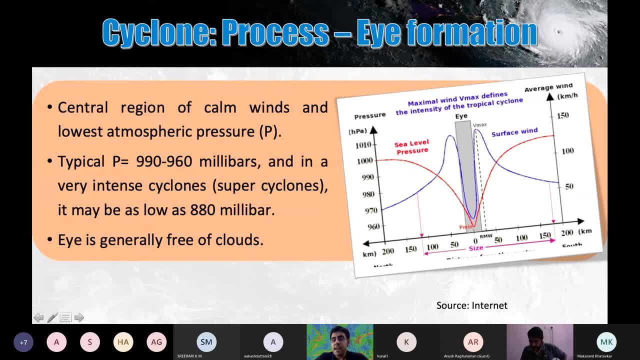 150 kilometers per hour. it will drop 100 kilometers per hour near the end of the cyclone, outer eye of the outer band of the cycle. But for disorganized cyclones like Nivar, this particular drop is going to be massive and what we feel during the cyclones as the cycle is approaching, the first thing we 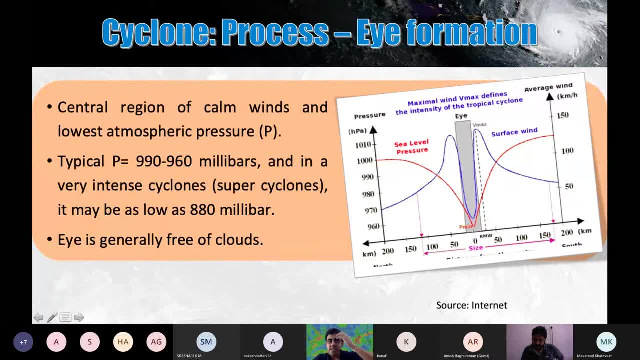 feel: is these, these winds, All right? So, More than the wind shear, because the wind shear is just one aspect and I think the wind shear is not the right. I mean it is, it is one of the metrics, but we do not have a very good 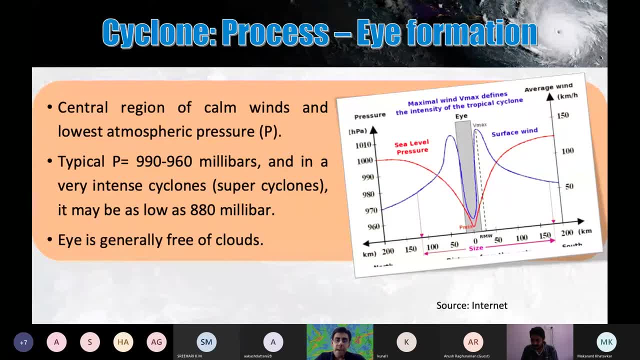 handle on what exactly is the exact value of the wind shear. But a better thing is the organization of a cyclone. So Nivar never had opportunity to get organized because of the topographical effect from Sri Lankan topography and also from the delta topography. So the winds 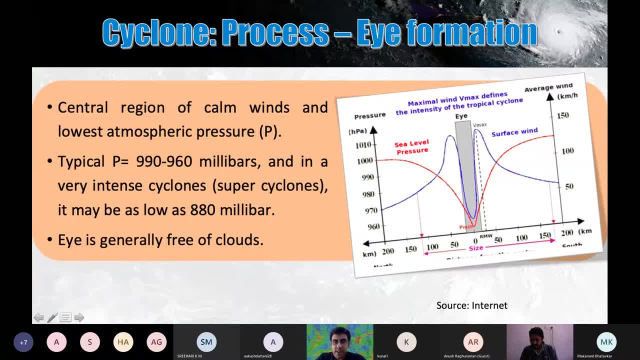 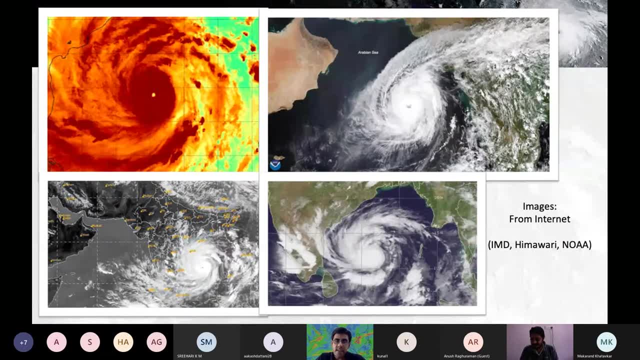 actually never could. so the cyclone could never become compact and that was one of the reasons why you did not expect- and it was expected- that even if it is a very severe cyclonic storm, the damage will be will not be too much, because the cyclone never could organize even before landfall. 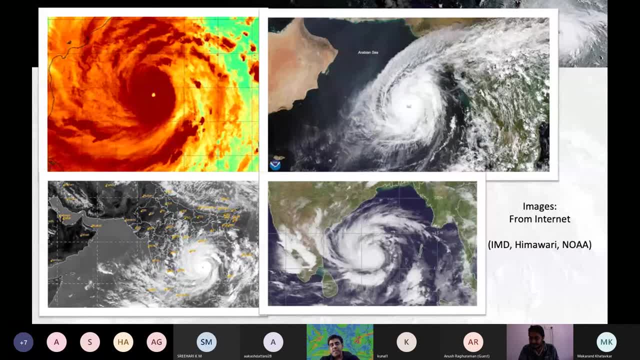 Yeah, Okay, Thank you, That was informative. So Burevi was a very. I mean I am still not very. I mean I am still in awe of Burevi because it was a. it was something I mean for a cyclone giving. it was more of a depression. I would say like: 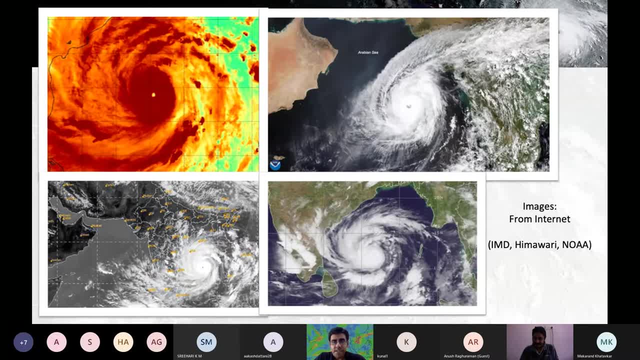 it, although it was getting a cyclone status, but it behaved like a depression which kept giving rains for almost seven or eight days continuously, and I am not too sure what happened there, but it would be interesting to do a case study on that. Okay, Yeah. 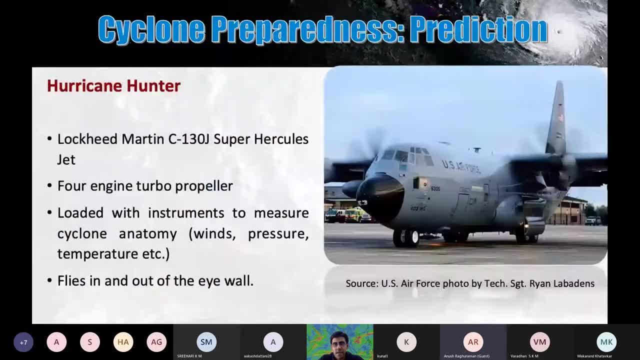 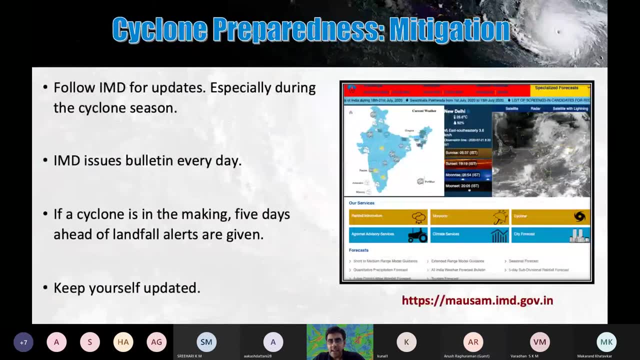 Sir, can you please tell about that Varkar circulation once again, sir, How it dominates the El Nino. Okay, Can I can? can I do it later? Yes, sir, No problem, I think we can start this month soon because 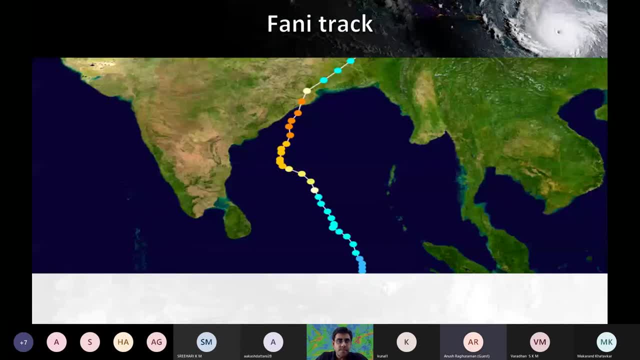 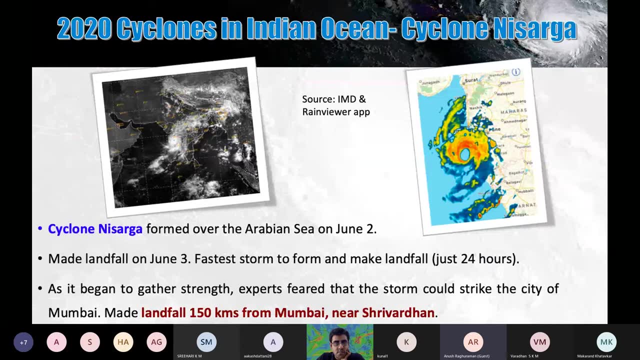 Yes, sir, Yes, sir, And Burevi on question. sir Burevi did not give rains to southern parts of the Tamil Nadu. sir, Even though it was near Ramanathapuram, nearby Toothukudi district did not get rains. sir. 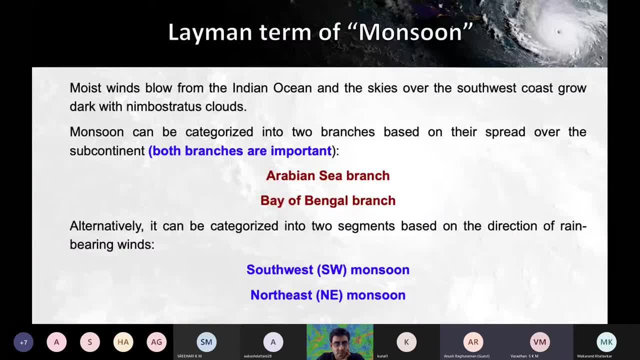 Oh, that's right. Only the northern parts, like Delta, Kavir, Delta, Tanjavur, through our districts, are getting heavy rain. Kadalur also was getting very heavy rain, sir. Hmm, What would be the difference? Hmm. 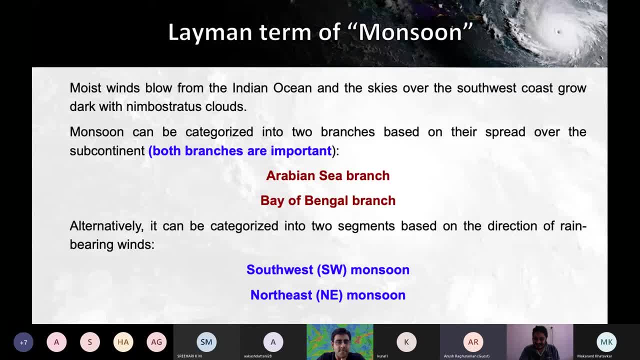 What would be the difference? There is an nearby Kanyakumari district did not get rain. Kanyakumari district did not get rains because that's on the southwest. I think the rain bands did not fall there. probably, Actually, if you see yesterday's rain pattern, as of yesterday. 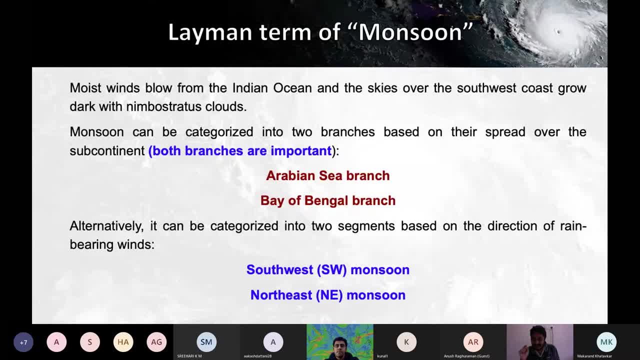 rainfall statistics. Kanyakumari district is having the highest deficit in with regard to NEM: minus minus 38 percent. Yes, sir, Kanyakumari is minus 38, sir, Correct, Right. So this is the problem with the. 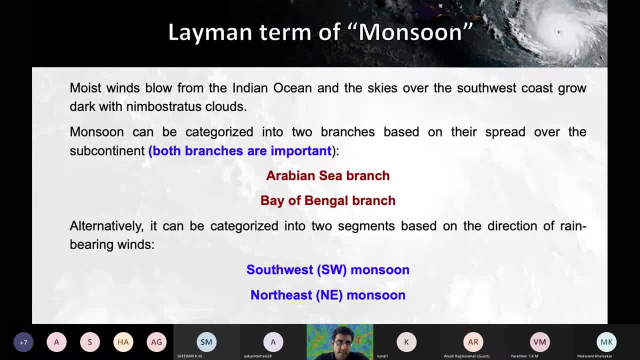 Correct, Right. So this is the problem with the Correct, So this is the problem with the. these is like these, these kind of patterns and systems, because the rain bands are very important and where the rain band falls is is the key. um, so it's yeah. so so most of the times when the system 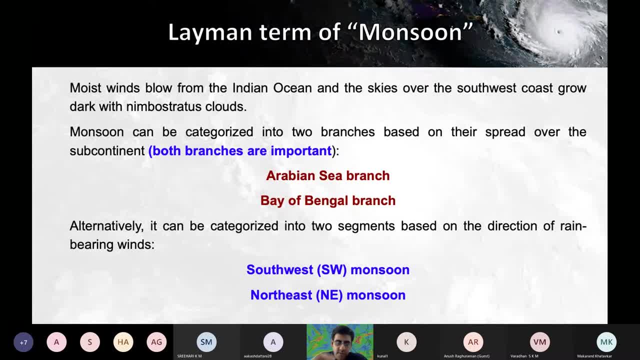 is kind of circulating uh, so. so one of the one of the issues is that this particular system, it was stationary for a very long time and it it never, uh it could never enter into kanyakumari uh, so the rain bands were always near, uh i think that uh region near tiruvarur and uh the delta. 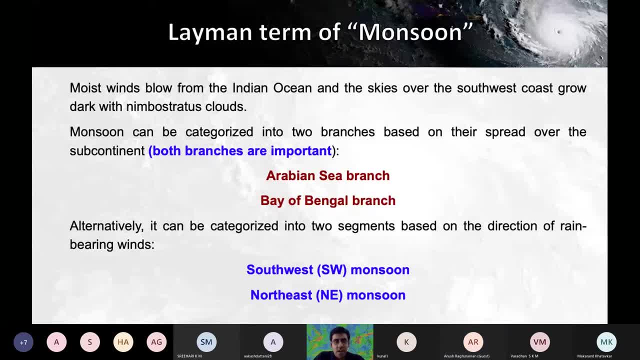 yeah, so, like i said, hyperlocal or not, even not hyperlocal, it's not very easy for me to tell what happens. i mean, yeah, so these are the things which are the questions for the future generation, probably like: what are the things which are the questions for the future generation? probably like: 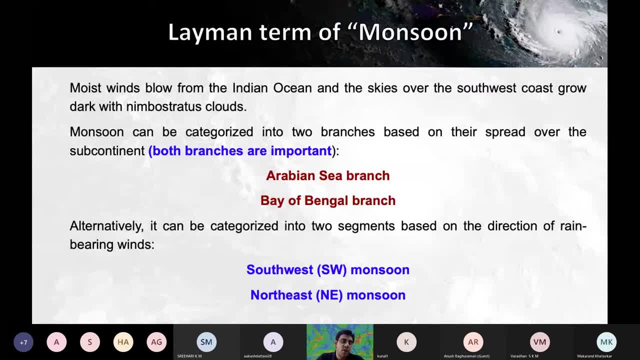 how can we improve these uh predictions of rainfall from these systems? uh, this, that, that's that. that has been a long-standing question, like even even during monsoon season. uh, what happens is some of the time, sometimes you get the very heavy rains, uh, even over. let's say, i take a place like mumbai. uh, the coast of mumbai will. 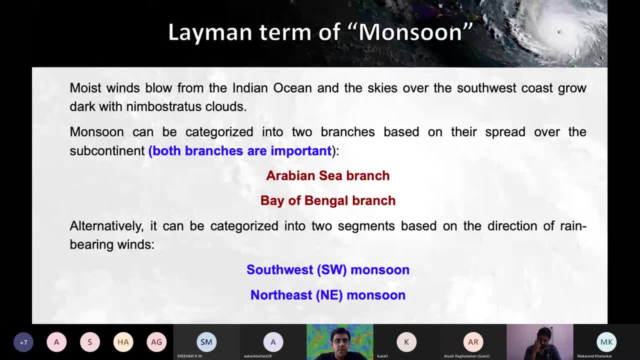 get, uh, let's say, 200 mm, whereas as you come 15 kilometers inward, you will only have like 10, 10, 10 train. so this kind of spatial variability is something which we don't understand, and that is. that is something which we have improved, of course. thank you, thank you, thank you, sir. 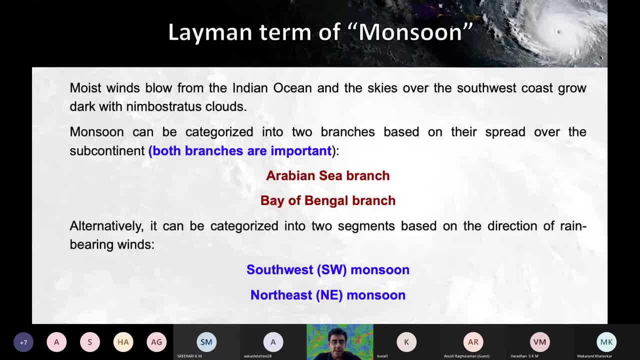 okay, so, uh, yeah, so we we'll get it, we'll, we'll, we'll, so in. so when i so i'm not covering not this one soon because there is no time, but yeah, um, i'm just going to talk about the southwest for the next 20 minutes before we head to the lunch break, and this is the last module, so, um, after that we will. 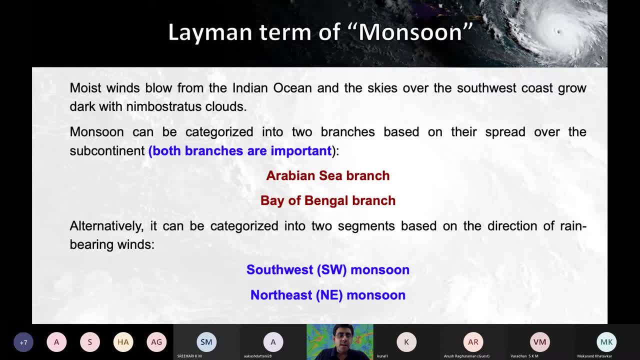 we will get into do in the afternoon session. we'll just do some- um, what do you call looking at some charts- not charts websites- from where we can do forecasting? okay, and then 3: 30 pm dr osalikar will take over. so, uh, of course the monsoon is a very important thing for india and we have 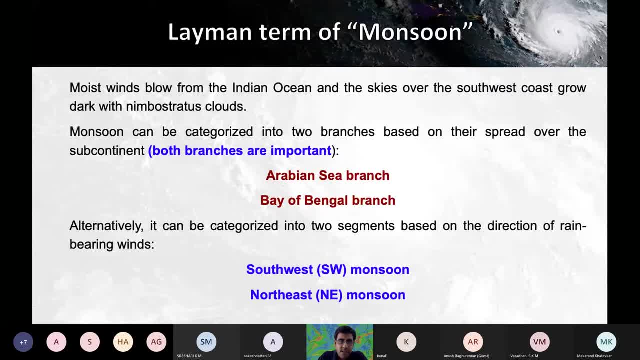 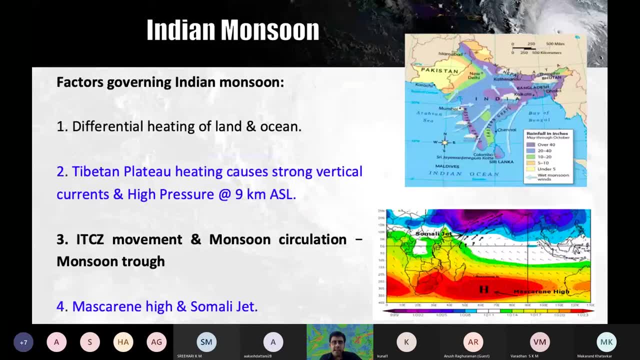 two important branches, which is the arabian sea branch and the weir finger branch, and both of them play a very important role in both the monsoon seasons, which is southwest as well as the northeast monsoon. so i want to actually focus on the mechanism of this monsoon for me, or the 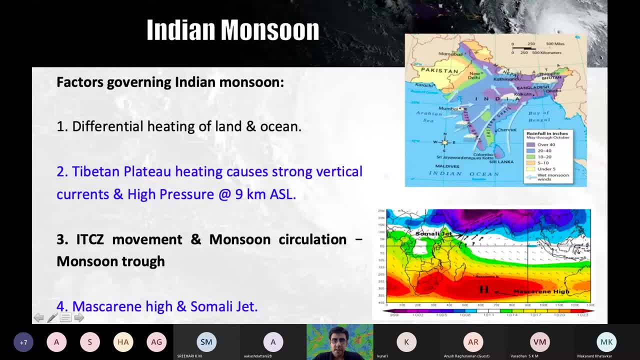 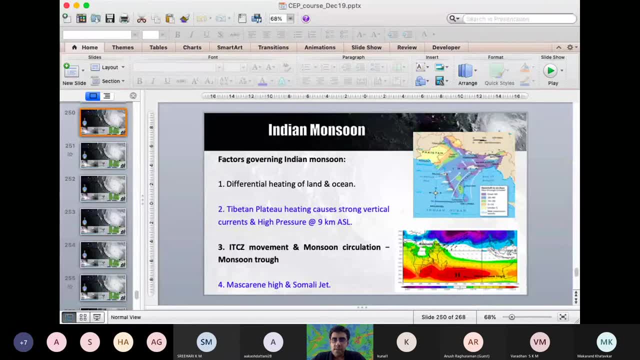 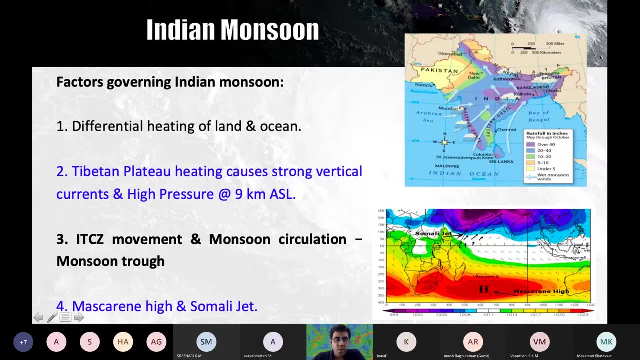 monsoon currents. so why do we see the monsoon currents? so, starting around may, or around april or may, what happens is that this particular. so what happens is you have this heating over land, definitely heating over land and ocean, because your tibetan plateau, which 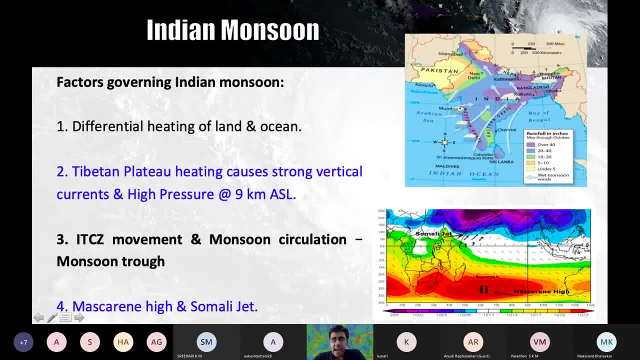 we talked about, which is now somewhere here. it kind of starts heating up, and that heating up of tibetan plateau is related to many factors. like i said, the siberian uh, cold air or warm air, how it intrudes into this region and the second thing is how the jet stream, the subtropical jet stream, moves. 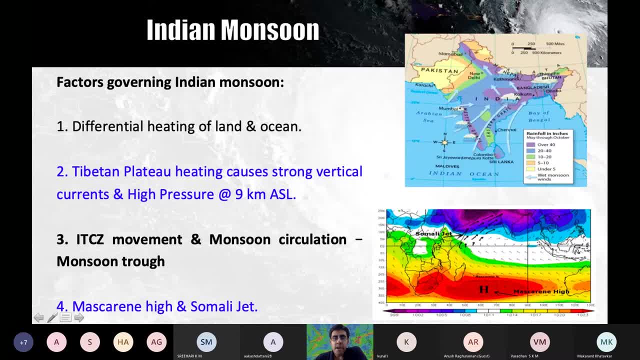 so those two actually govern how this tibetan plateau is going to heat up. okay, and that heating up is going to cause a very strong vertical uptract and it leads to a formation of a high pressure zone at around nine kilometer above sea level. so you have a very strong divergence at nine kilometer. 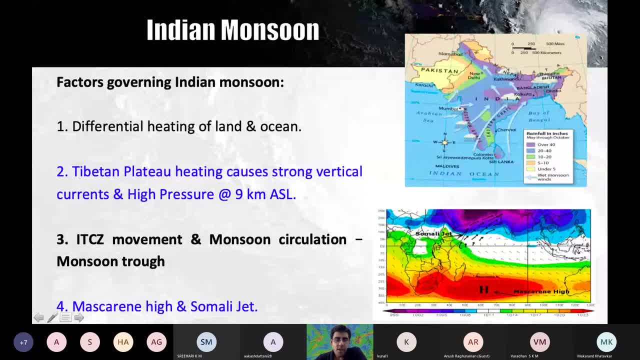 and you have a very strong convergence at low levels. so there is a low pressure which is forming here. so what that low pressure actually does is it actually pulls your intertropical convergence zone, starting from the equator to north. that is when the monsoon actually starts. 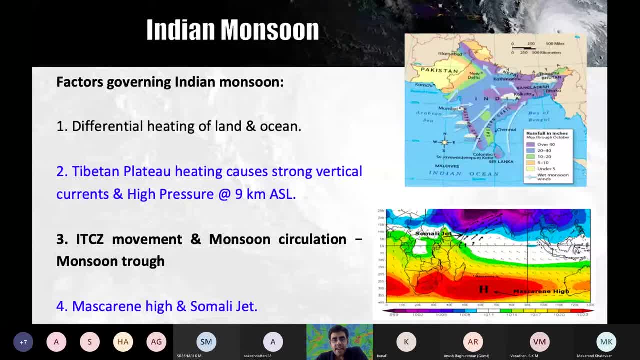 uh, its process over india. so the three things that we are on the lookout for is the differential heating of of the land wherein the tibetan plateau starts heating up, and the heating up of tibetan plateau is again related to- uh, these, uh, these, these extra tropical dynamics that we discussed. 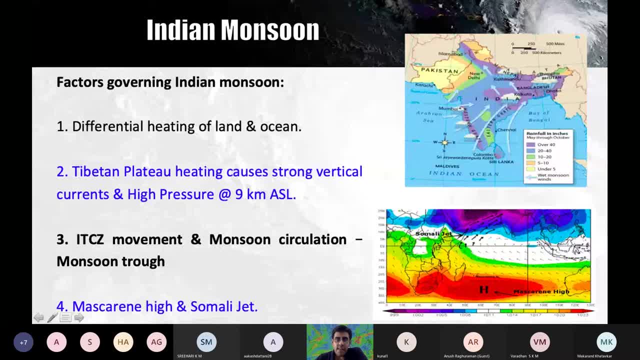 okay. and the second thing is we are on the lookout for when the it sees it, which is the band of clouds that we discussed yesterday, how this it sees, it starts moving. so at the time that it sees it starts moving, then our southern hemisphere is also very interesting because 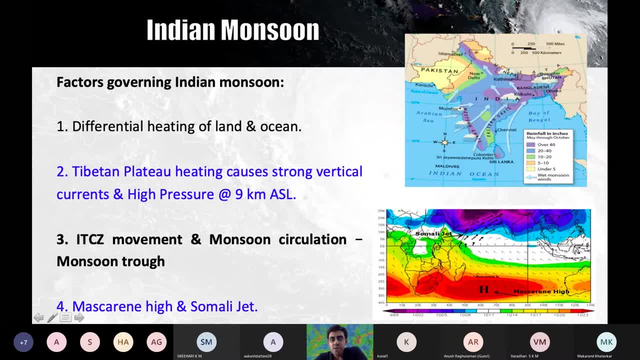 our southern hemisphere also plays a very important role in uh monsoon onset, because you have something in the masculine islands near the, near madagascar, you have something known as the masculine high. so this is: this masculine high is over the, over the ocean, so this masculine high. 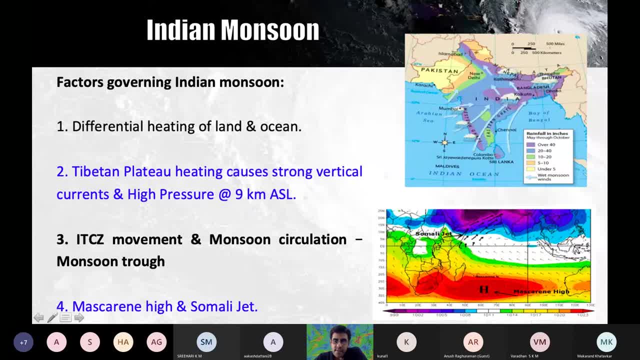 what it does is it deflects the winds coming from the southern hemisphere towards the northern hemisphere. so this deflection of the winds is what gives rise to your westerly patterns and, because of the tibetan plateau heating, these winds are pulled towards, towards the himalayan or tibetan. 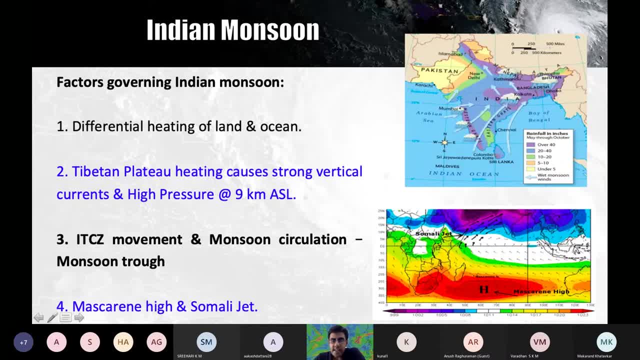 plateau and they cover, they enter the western part of india and then they slowly move towards, from towards the central part, northern part, and then this, this is the circulation cell that gets, that is, this is the monsoon circulation that i'm talking about. so this westerly winds actually. 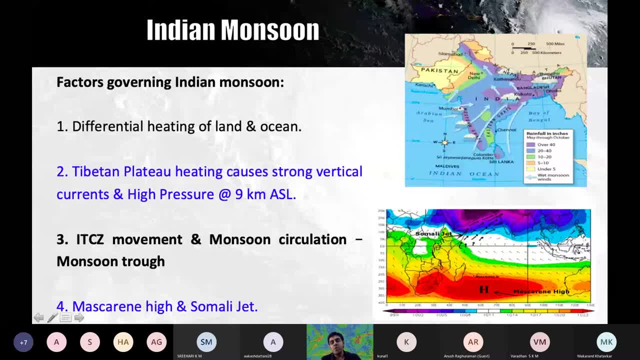 trigger a monsoon circulation, and then this is the monsoon circulation that i'm talking about. so all of these things have to happen together for the monsoon to arrive. tibetan plateau heating the masculine high, creating these low level westerly, which is also the somali jet, which 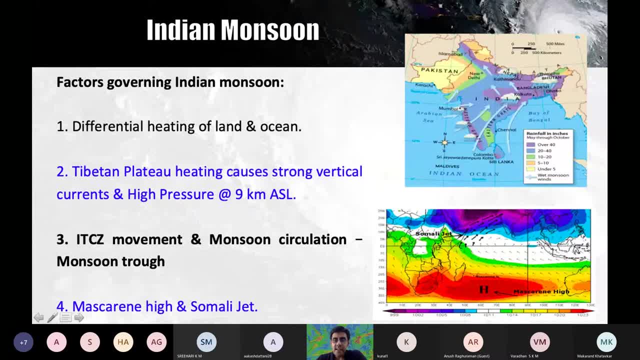 we call the somali jet, the formation of the somali jet and the initiation of the somali jet from africa towards india, so basically, and the location of the itcz, which is the intertropical convergence zone. so where is the itcz, where is this westerly wind and whether the 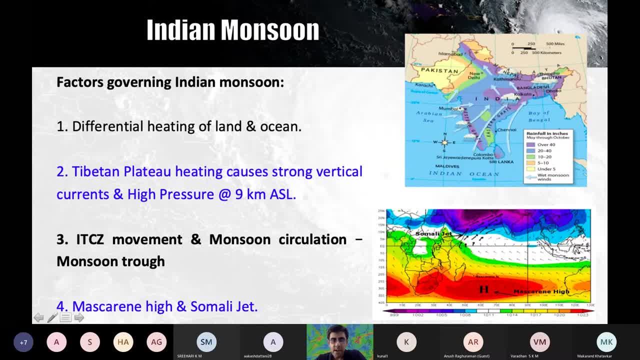 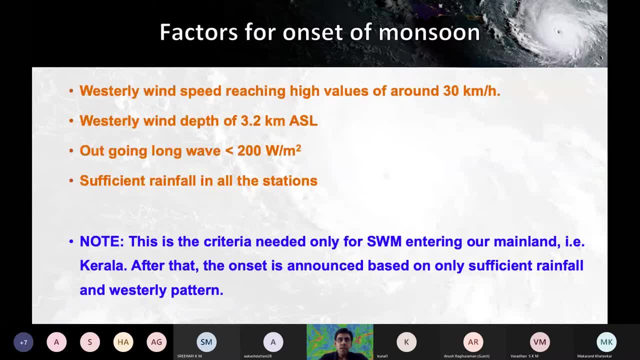 tibetan plateau is heating, whether there is a low pressure over tibet, over the tibetan plateau. these four things are actually the important factors that govern the onset of the monsoon. so what, what we are on the lookout for to announce the onset is the westerly wind has reached around. 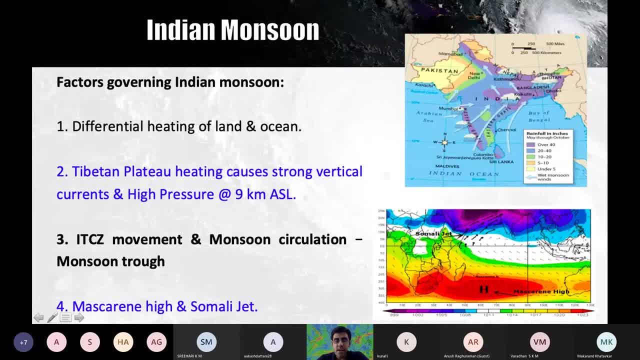 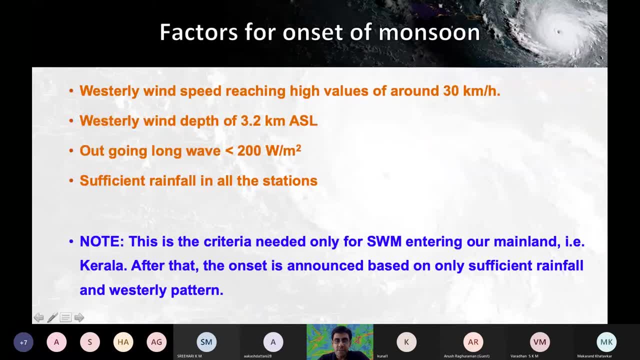 30 kilometers, so these westerly winds should be very strong. so the speed of the westerly winds should be, because it's a jet- right, it's a jet, so the jet should be very strong, so it should reach 30 kilometers per hour. wind speeds: the westerly wind should be very strong, so the speed. 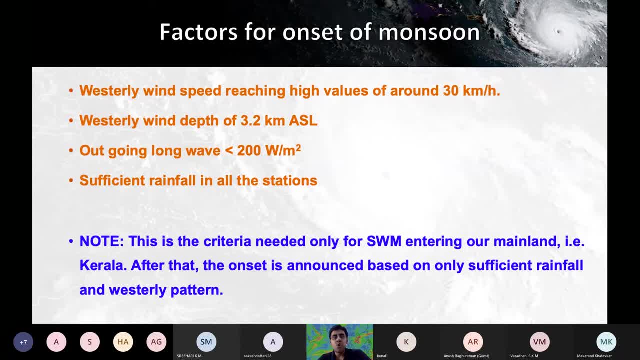 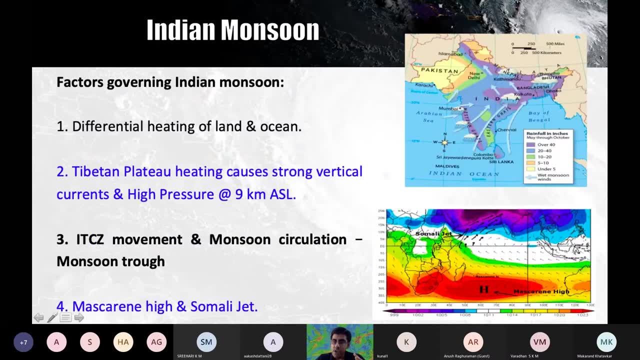 depth should have attained 3.2 kilometers above the mean sea level, So up to 700 HPA or up to 700 millibar level. the westerly winds should have settled Because during the normal time the winds over surface are easterlies correct. So right now, if you look at the wind charts, 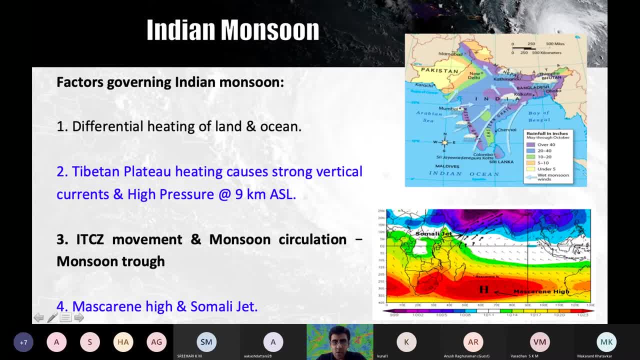 you will see that the winds over India are easterlies. Throughout the India you are seeing easterly winds, except for the northern region where the winds are westerlies. So what happens during monsoon season is the winds pattern reverse between the southern and central part. 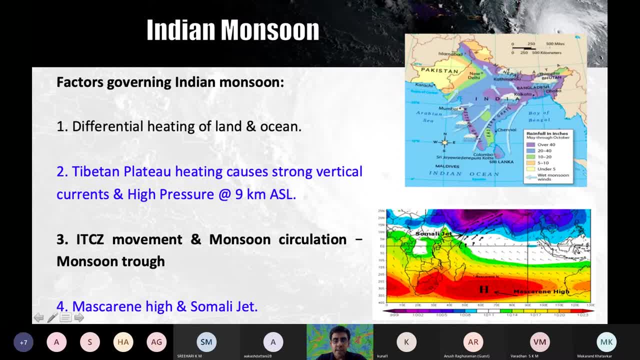 of India and northern part of India. Right now, the winds over western northern part of India are westerlies. During the monsoon season, the winds over the western, the northern part of India will become easterlies. okay, So that is one thing that we see. So it is clearly shown in. 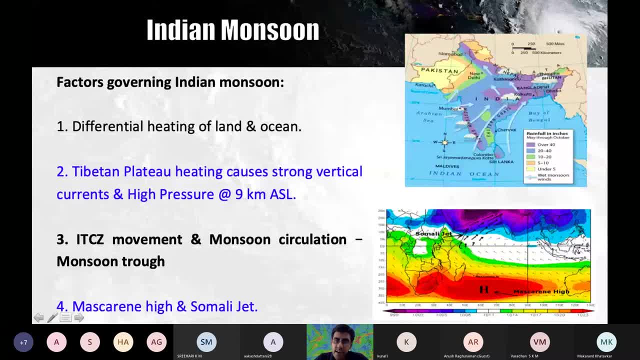 this image right. So there is a westerly wind in southern India and west coast of India or central India, and there are easterly winds in near Delhi and northern India. So this is what is the monsoon circulation, because if you draw a circle, then you see an. 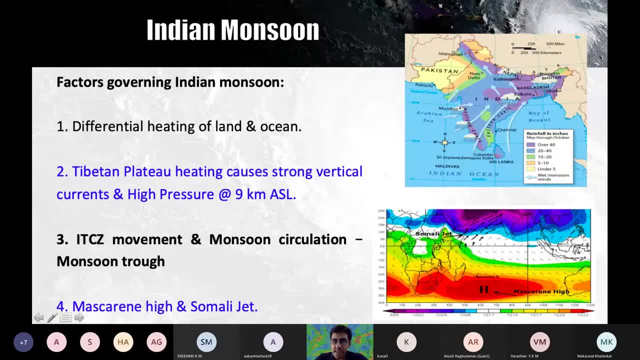 anticlockwise pattern, which is a low pressure system, and this low pressure system is covering this entire India and that means that a distinct low pressure system forms over entire India, which is going to allow the Arabian Sea branch to push the moisture and it is also going to allow 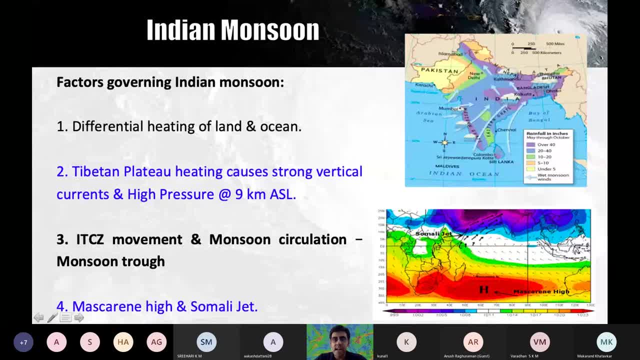 the Bay of Bengal to push the moisture, and this is the monsoon circulation that I am talking about. So you can see the westerly winds setting over central India and the easterly winds setting over northern India will automatically give a circulation which is very favorable for the 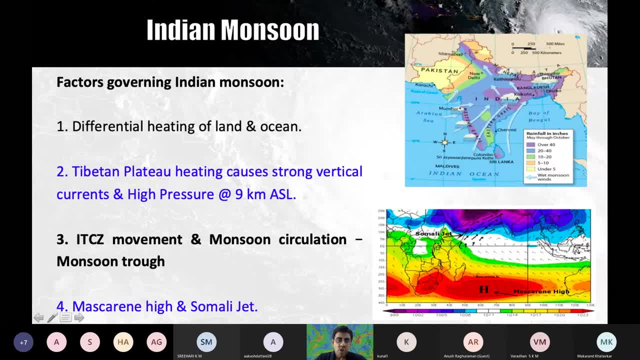 formation for the cloud bands to keep coming in from both the basins. okay, So this ITCZ plus the monsoon circulation is what we call as the monsoon trough or MISO. So the ITCZ is the line which is the line between, is the line where your westerly winds and the easterly winds meet. 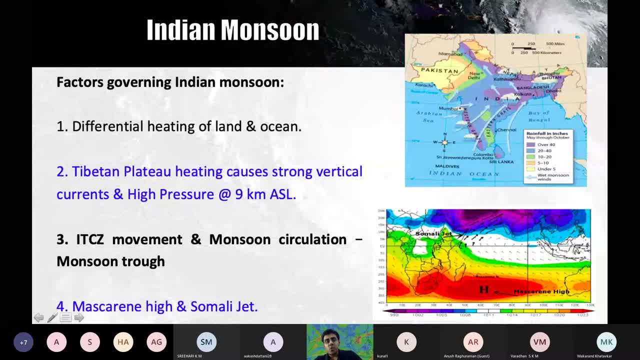 is the location of ITCZ right now. So during monsoon season, how do I find the ITCZ? I take a 850 HPA wind chart. I will show how to do that. Give me some time. I look at the wind and I see. 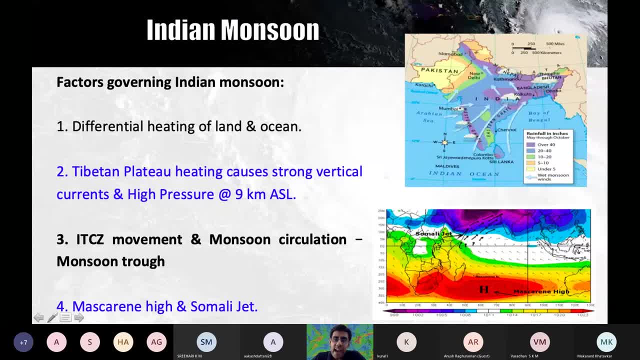 where these two winds are meeting and that is the location of ITCZ, And the circulation cell is also active there. So my monsoon trough is lying around this line right now. So, extending from Bay of Bengal to somewhere close to North Hong Kong, is where the monsoon 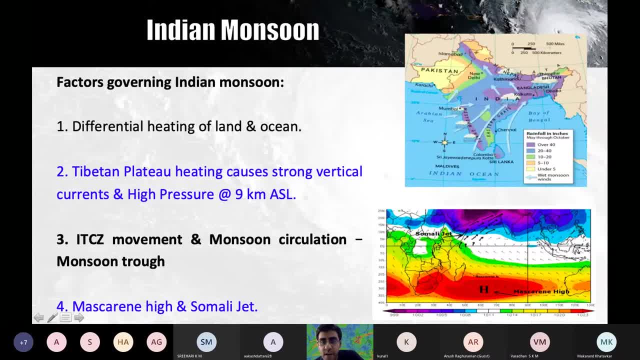 trough is lying In this image. this is how I find the monsoon trough And this monsoon trough, which is MISO, also synonymously called MISO. this monsoon trough is not stationary, It will move up or down. So I have to track the monsoon trough because that is where most of the action. 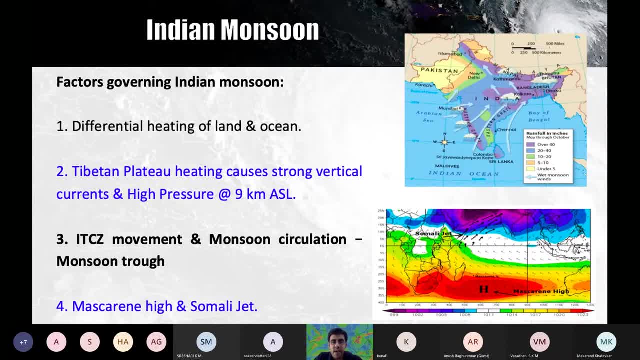 is going to take place Where the monsoon trough lies. that is where flooding rains are going to most likely occur. So whenever I am talking about monsoon, I need to find the monsoon trough. And how do I find the monsoon trough? Where the westerly and the eastern 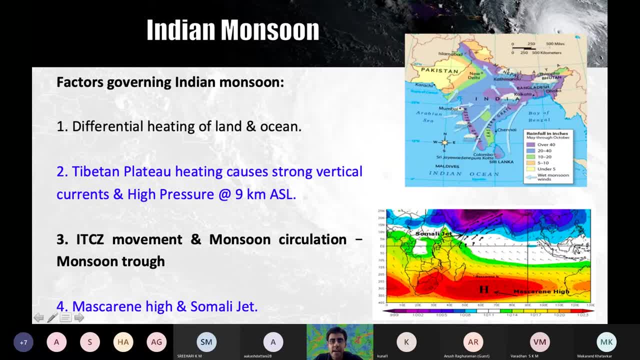 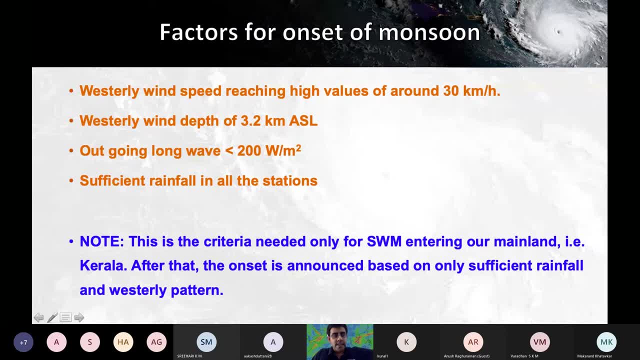 Where the westerly winds meet and where the ITCZ is present, which is the cloud band, is present. Okay, All right. So this is the criteria for onset of monsoon: Westerly wind depth: 3.2 kilometers. 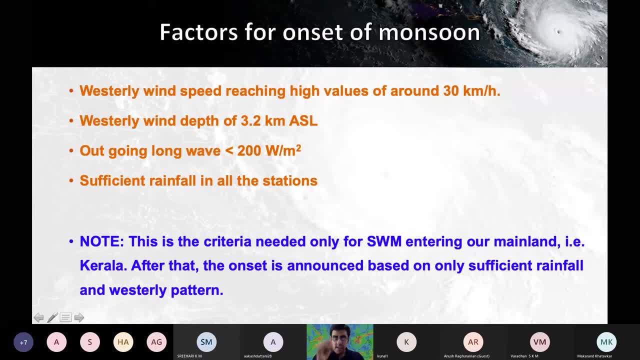 outgoing longwave radiation less than 200 watt per meter squared. So this is the onset of monsoon factor. only for Kerala, only for entering our mainland, which is Kerala, After it has entered Kerala, we all these, so only for Kerala. all these four parameters have to be maintained. 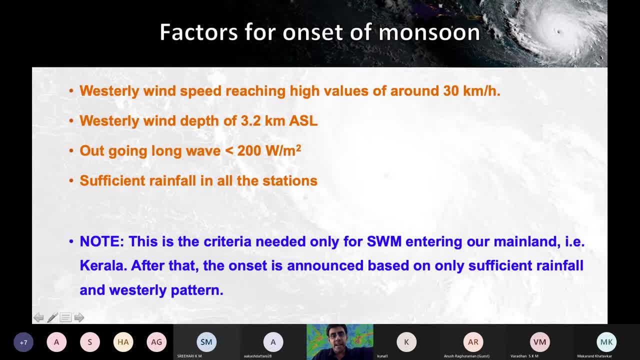 After it has reached Kerala as it as the monsoon starts propagating up north. all these parameters do not matter because even if I do not have a westerly depth all the way to 3.2 kilometers in Mumbai, but if I have sufficient rainfall and a westerly pattern at low levels, 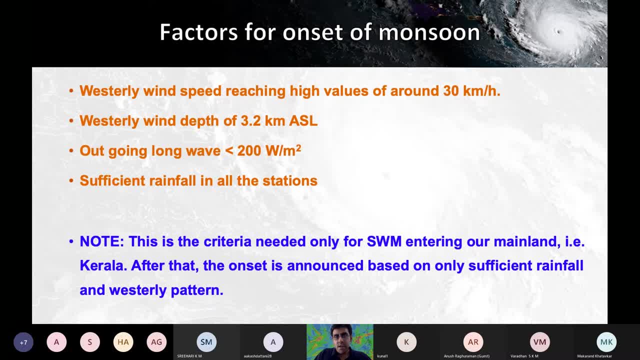 that itself is good enough for me to announce onset of monsoon. So this is very important mistake that lot of weather bloggers do- that the IMD announces. See, this is where I am saying that IMD has a set rule And weather bloggers do not have a set rule and they keep saying that IMD is wrong. IMD is. 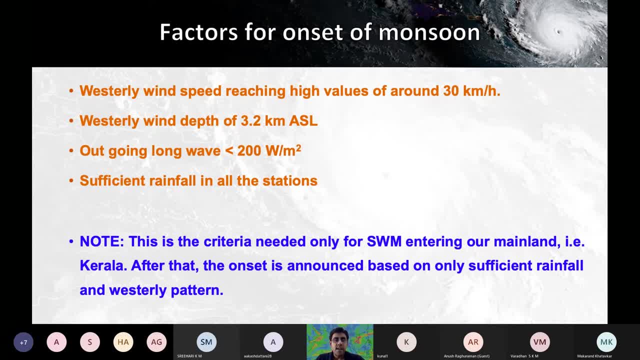 no, that is not true, because IMD has clearly said in its record that this particular criteria is only for the southwest monsoon to enter the mainland. After it enters the mainland, the only thing that is important is the sufficient amount of rainfall, So I do not care whether the westerly 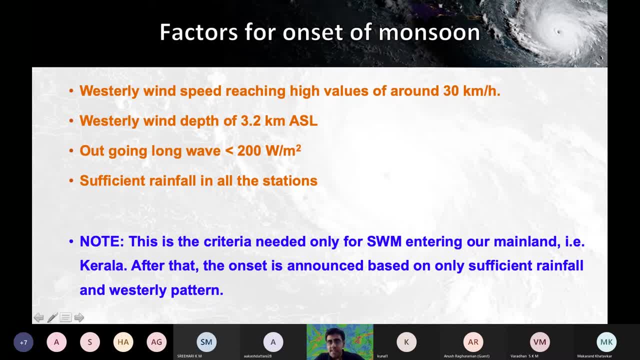 wind depth has reached 3.2 kilometers or not, in central India, or, let us say, Konkan coast. Even without this 3.2 kilometer low sea level wind depth there is, I can still get a lot of rain. okay, I can still get a lot of. 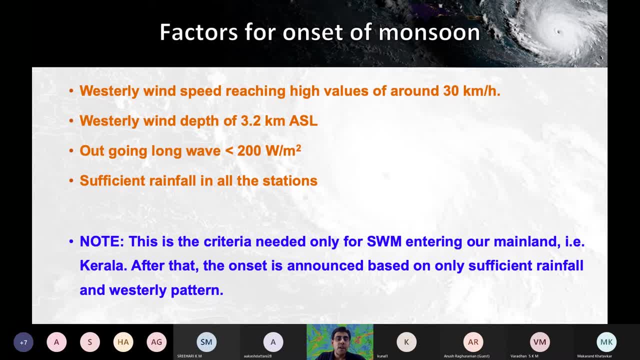 rain through some other mechanism, which is a trough or a weak monsoon circulation or many different regions, many different factors can give me rain. So after so onset, all these factors have to be kept in the mind only till the time onset has announced over mainland. After that, 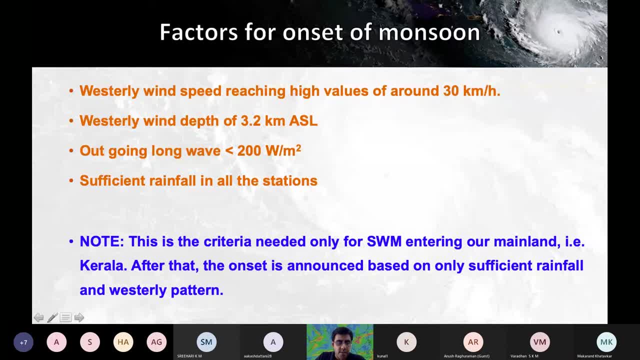 even if we do not satisfy this, but sufficient amount of rain, we can still get a lot of rain. Now, if we do not satisfy this- but usually we do not satisfy that- right then what happens When we do not satisfy this, we do not satisfy the monsoon, downfall and estawn. 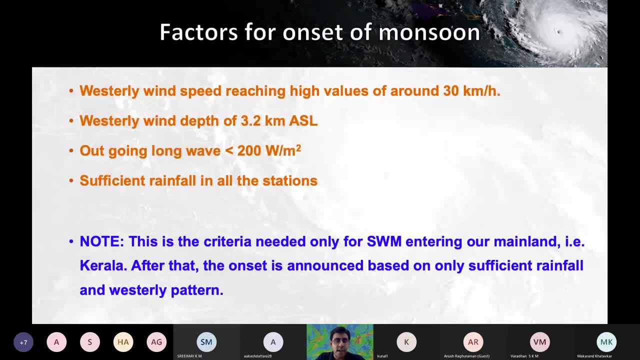 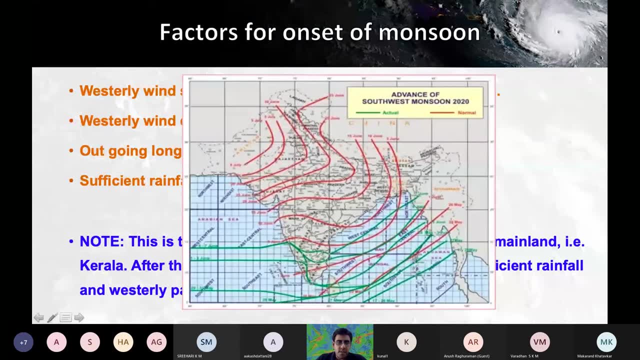 so after that we can still get a lot of rain. So this is an interesting thing. this is the recent initial analysis of the monsoon analysis from the last monkey wrestling. So this is a monsoon analysis, So we can see that there is this. 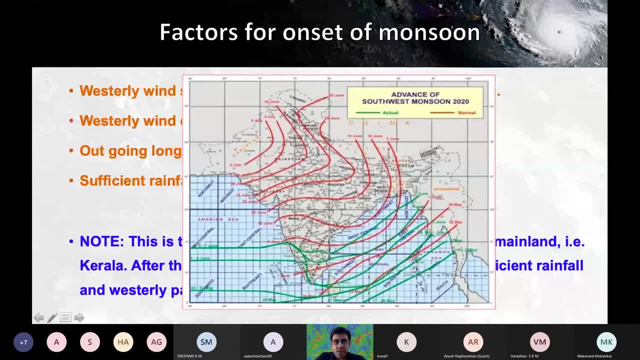 easterly and this level the winds are westerlies during during the monsoon season. this reverses. what happens is, in this region up to up to gujarat, the winds become westerlies and after that the winds are easterlies in the north north india. so that is the. that is the shift that happens during. 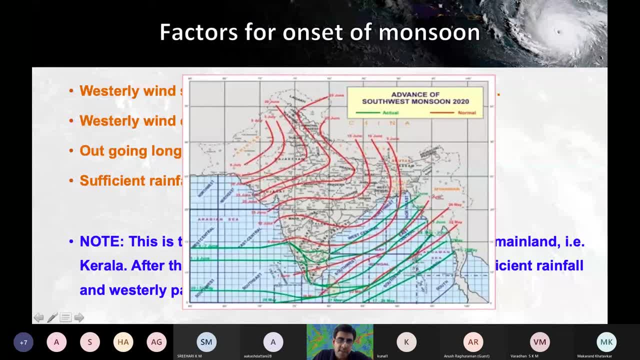 monsoon, and that shift is very important because it automatically gives rise to a monsoon circulation, and i have already spoken about monsoon circulation because i feel like this monsoon circulation is one big parameter which actually governs lot of things. so it so climate scientists are now saying that the monsoon circulation which is persistently there for 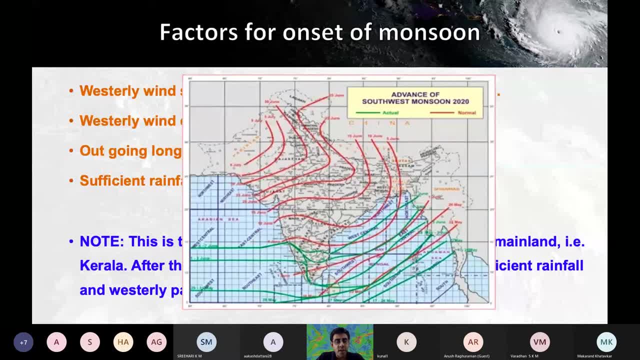 a period of three or four months in india can affect the onset of el nino or onset of iod. so it is not the other way, it is not the. it is not that iod or el nino affects this monsoon circulation, but it's the other way around, where the monsoon circulation affects these. 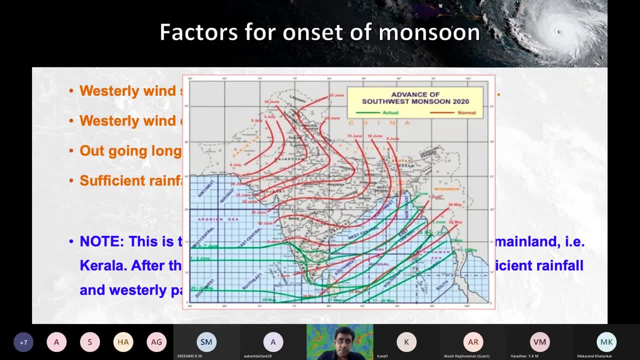 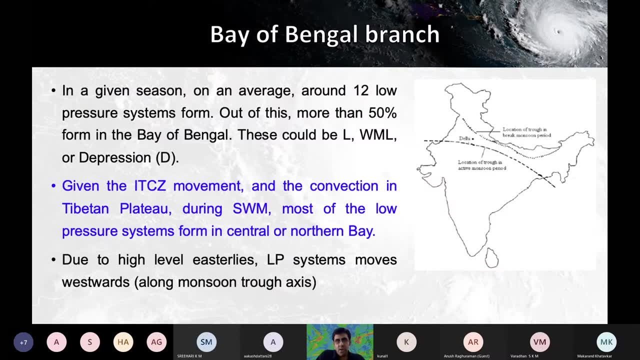 el nino or iod. that is what is the claim, which still needs to be uh kind of corroborated with a lot of evidences. okay, so bay of bengal branch plays a very important role because on a in a season, on an average 12 low pressure systems will form. 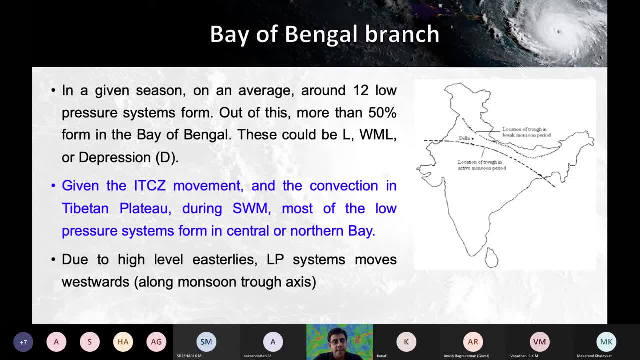 during the monsoon season. so 12 is an average. so starting from june to september or october, 12 low pressure low pressure systems should form. out of this. more than 50 percent of the systems form in bay of bengal, which is very interesting. uh, most of the time what happens is the system. 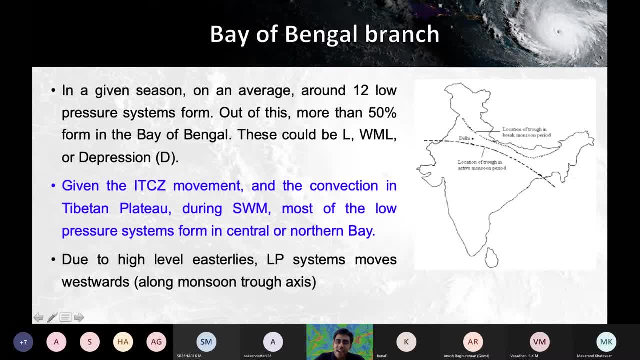 forms in bay of bengal, let's see, in the northern bay of bengal, and it always moves. always it will move along the line of the trough. so this is why the monsoon trough location is very, very important, because, if i am able to find, 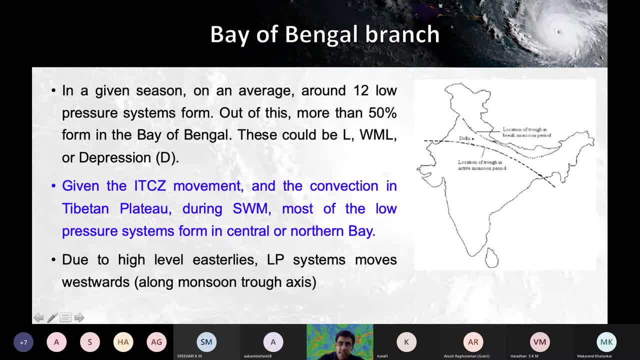 the location of the monsoon trough. and if a way of bengal system forms in the arabian, if the system forms in the bay of bengal, then it will 100 move along this line of monsoon trough. so location of monsoon trough is very, very important. uh, because that is what governs the movement of any system. 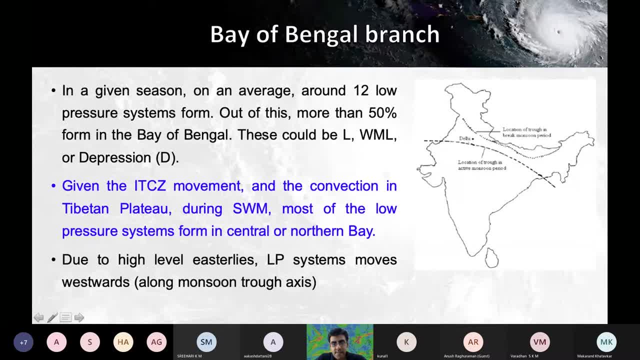 so it is very important for us to understand what is the role of monsoon trough in bay of bengal. then what is the role of arabian sea? the role of arabian sea is very straightforward: once a system forms in the bay of bengal, the role of arabian sea is that it will push moisture towards this. 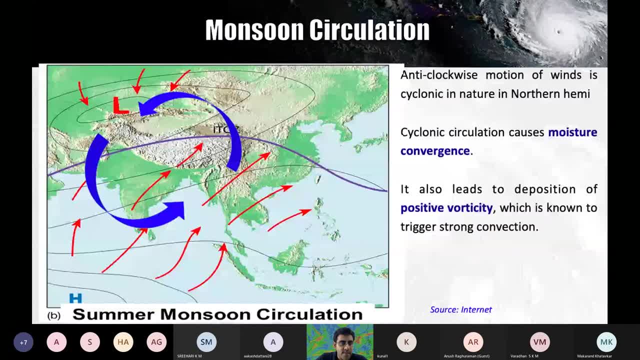 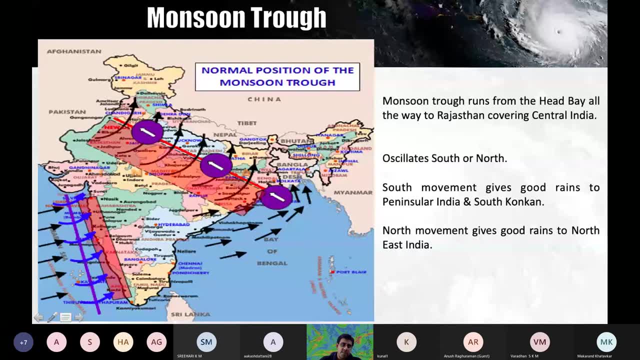 system in bay of bengal. as it is pushing moisture, it will form something known as an offshore trough. you don't have that here. let me just see. yeah, so this is the monsoon trough, this is the offshore trough. so as this system forms in the bay of bengal, this particular thing will bring in lot of. 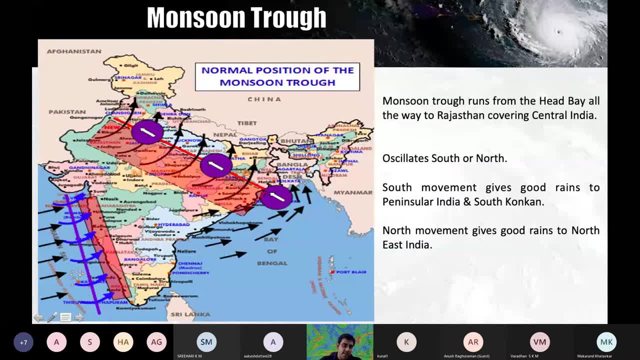 moisture from the arabian sea and you will form a something known as an offshore trough, which is one of the important mechanisms by which the entire west coast- west coast of india- gets massive rains thanks to the arabian sea branch. so this is how the arabian sea branch plays a role. 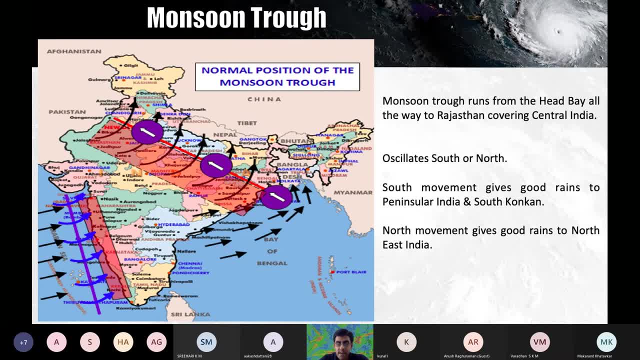 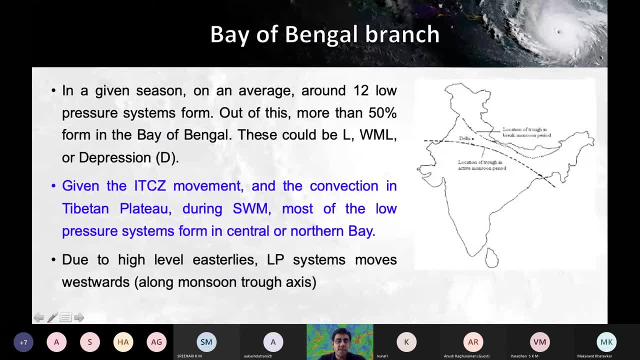 so, even though arabian sea branch doesn't- uh, it doesn't- produce a lot of strong systems- most of the strong systems are produced in the bay of bengal- but arabian sea actually plays a role of this moisture source. arabian sea is the source of moisture, and especially for west coast of india and central 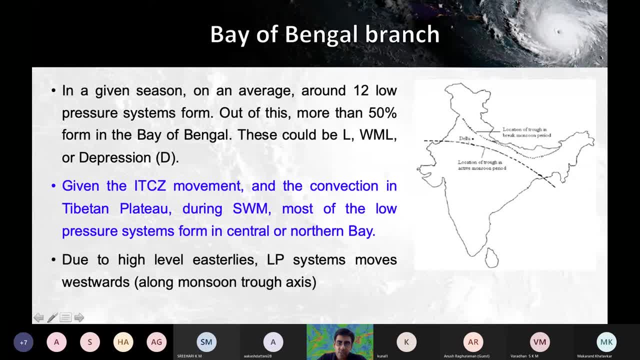 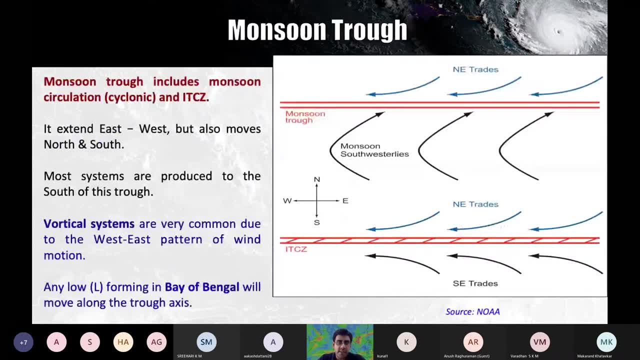 india, because whatever comes will get affected in this way, and it will because of the presence of western guards. thanks to the presence of western guards, we get massive rains. okay, the west coast of india gets massive rains, so monsoon trough is the location where the westerlies and the easterly winds meet, plus the itc that location. 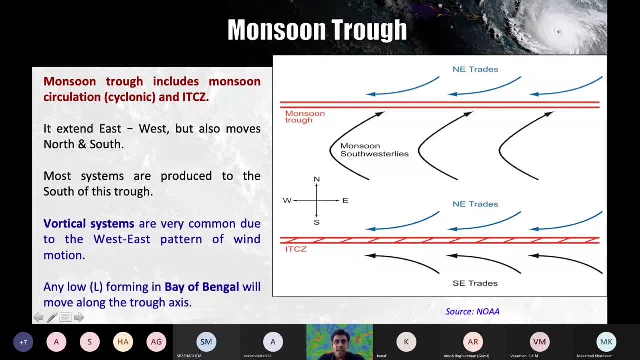 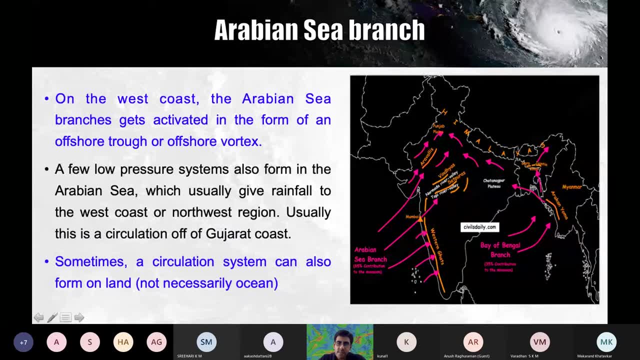 so i have already told you that no. so if you are interested in tracking the monsoon, my, my uh suggestion is that look for a system in bay of bengal and look for the location of the monsoon trough. these two things should be good enough for you to find out which places are going. 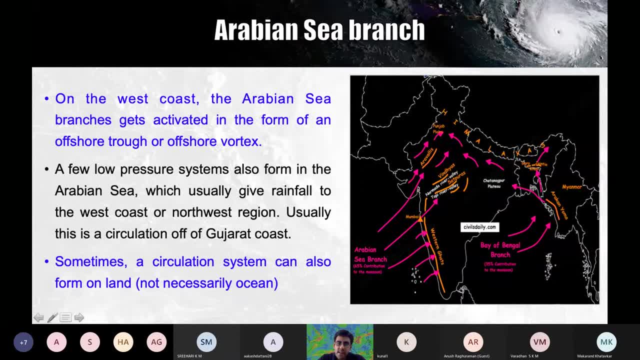 to get raised, because if the monsoon trough is located here, let us say in this region, and the way of bengal system is going to form here, then it will give heavy rains to coastal and the pradesh, telangana, maharashtra, southern south maharashtra and also to the north hattagiri coast and all those. 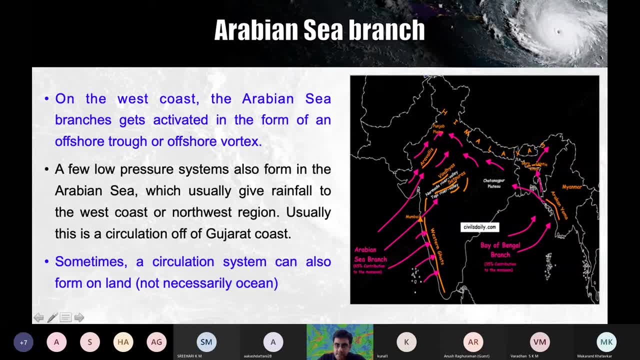 including mumbai and pune and all those places. as this monsoon trough shifts here, you will have a system forming in the northern bay of bengal which will automatically move towards gujarat, because your access, monsoon, monsoon trough access is going to be uh, from extending from. 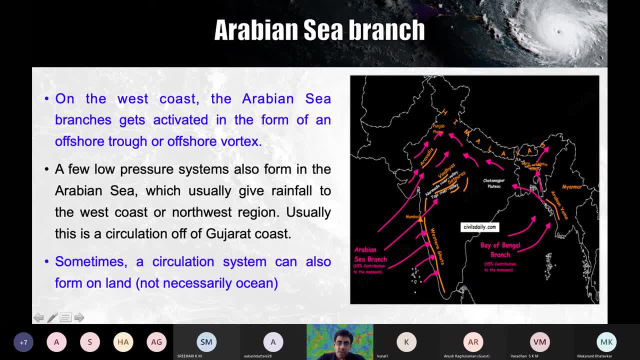 bay of bengal to gujarat. uh, this is what happened in 2005: the the mumbai floods. there was a very strong system and the monsoon trough was very active, which was see, the monsoon trough has a very distinct- i mean, it has a very interesting physics, because it is- yeah, it is true that most of the 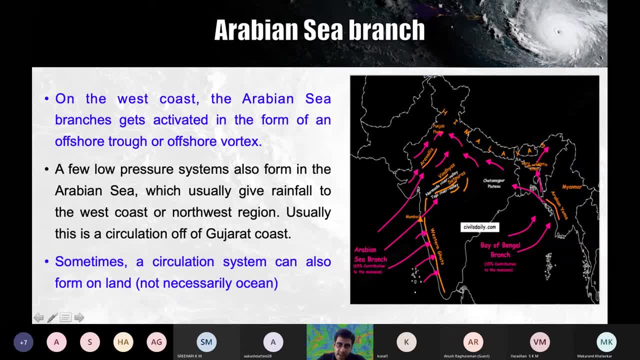 systems will move along the monsoon truck, but sometimes the systems can move slightly, wobble up or down. okay, so as that wobbling happens, you can. it is very hard to predict which region will get affected the most, so we know that most of the regions will get heavy rains, but it is very 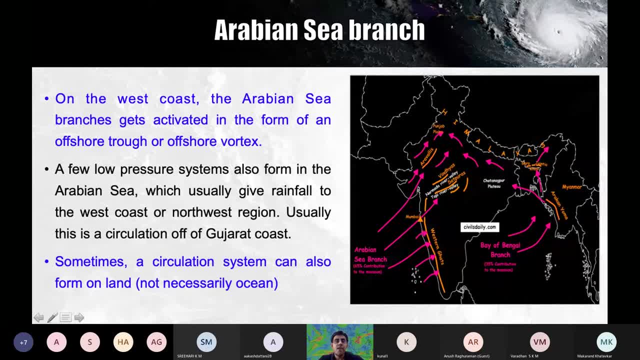 difficult to predict which region is going to get extremely heavy rains. that is the one of the most i can overall i can say, tell the picture what is going to happen. i can convincingly say, say that any system in northern bay of bengal is going to give rains to central india, including madhya. 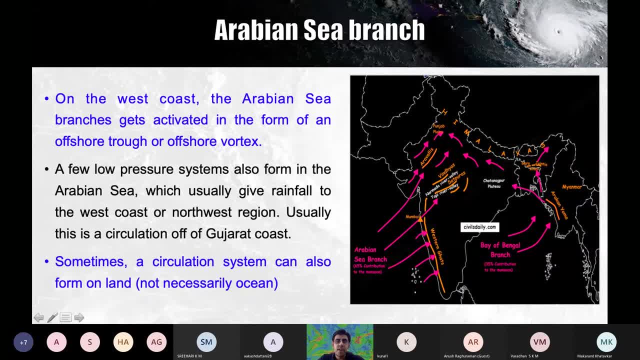 pradesh. so expect floods over madhya pradesh, expect, expect floods over uh, uh, expect floods, floods over, uh. not conquered, because any system here is going to affect north kongan directly, because arabian sea branch is going to bring in a lot of moisture due to the offshore. 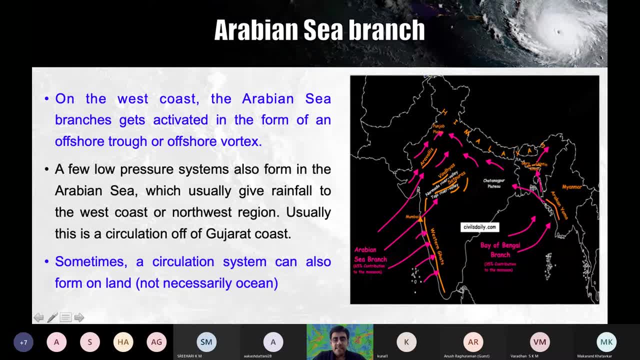 but the thing that i cannot pinpoint is which places in mumbai is going to get extreme heavy rains or which places- uh, let us say in gujarat- is going to get extremely heavy rain. so that is where the uncertainty lies. so, although i understand this monsoon system decently well, 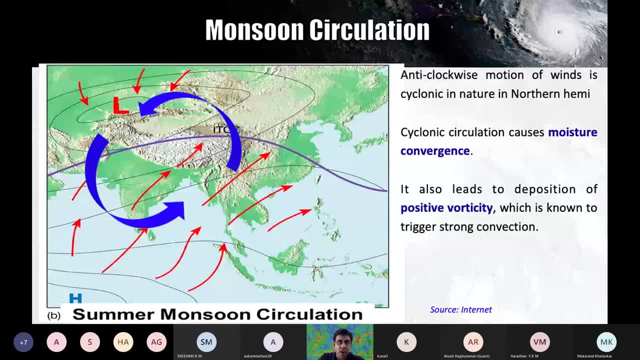 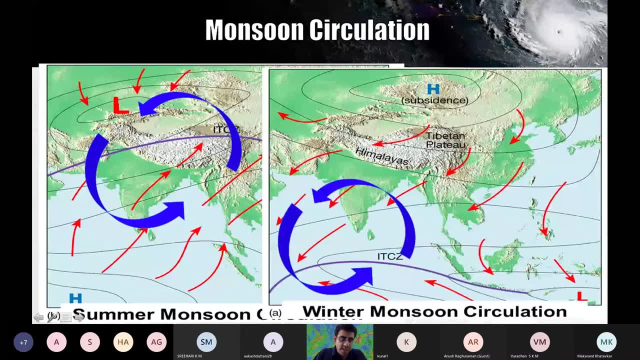 but again, the spatial variability is something that i am, i am not able to- none of us are able- to predict that. okay, so that is where the challenge lies. so this is the monsoon circulation during summer monsoon, which is southeast monsoon, and as the monsoon fades away, this circulation. 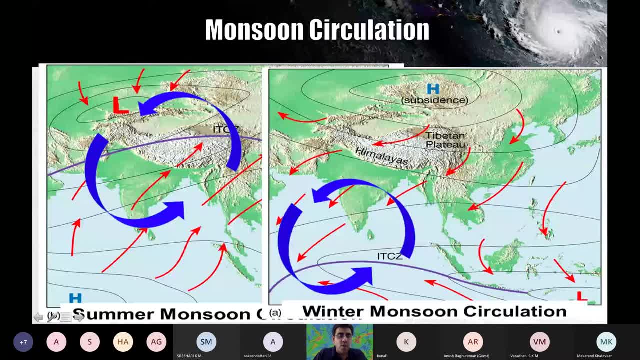 and it becomes weaker and weaker, and that is why you do not have a distinct monsoon circulation during the northeast monsoon. so during the winter monsoon, which is the northeast monsoon, the waves and the mjo take over. so this is the complete picture. uh, i am showing the somali jet, which is: 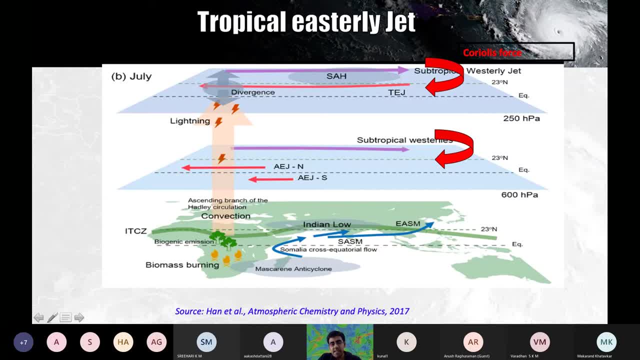 the cross equatorial flow. so this cross equatorial flow is extremely important, uh feature, because that is what is going to give you the somali jet. so we are always on the lookout for this cross equatorial flow from the southern hemisphere to the northern hemisphere. that is what is going to change the wind direction from the east, from easterlies, towards westerlies. 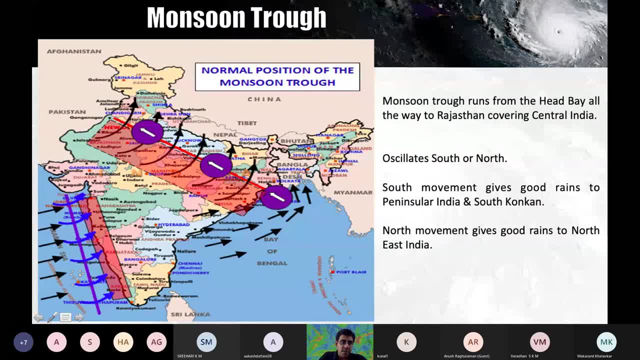 okay, so this i already talked about. the location of the monsoon trough is very important, because wherever the monsoon trough access lies, that's how the systems are going to move and that those are the hot spots for a very heavy rainfall. last thing is the offshore trough before i. so this is the 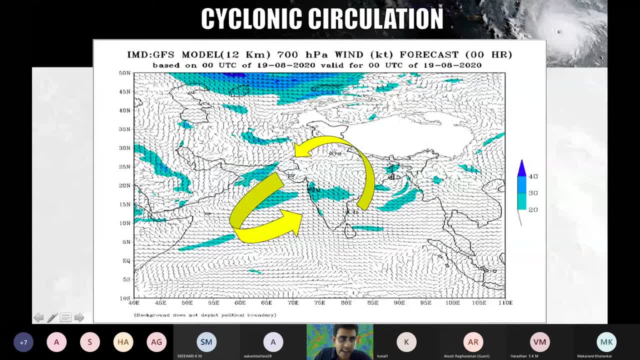 cyclonic circulation. you can see that the winds are easterlies near delhi and the winds are east coast and central india, and this is the automatic monsoon circulation cell which will which will be persistent, and this monsoon circulation cell is one of the reasons why 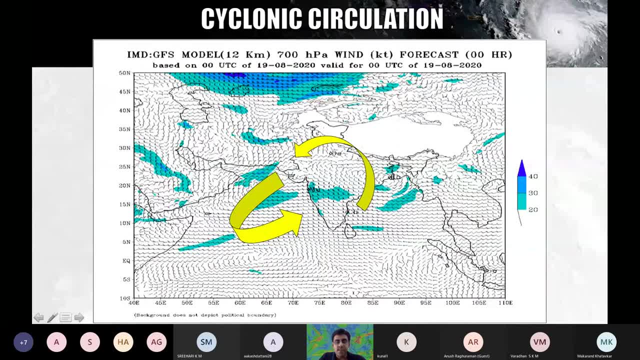 strong systems develop in way of penguin, like all these depressions, all these uh, deep depression systems actually originate from way of penguin. not many strong systems form in arabian sea, but arabian sea is the powerhouse of moisture. a lot of the moisture. without the arabian sea branch west coast of india would be dry, so that so the amount of moisture is. 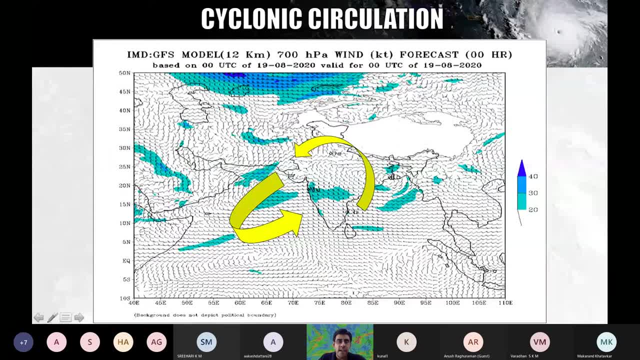 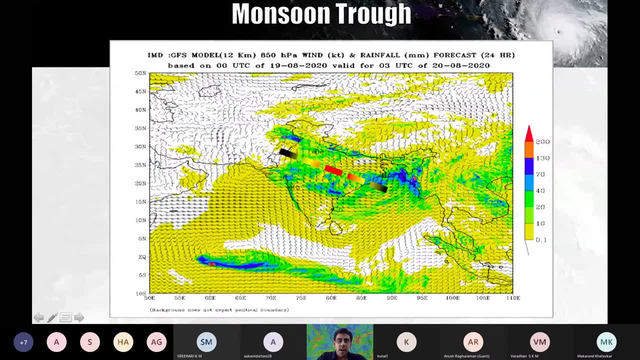 that somali jet brings in is the key for the west coast of india, where we record like 2000 mm of rain or 3000 mm of frame, which is massive, okay, uh. so how can you find the monsoon truck? you look for the place, you look for the line where the westerly and easterly meet. so this is the easterly wind. 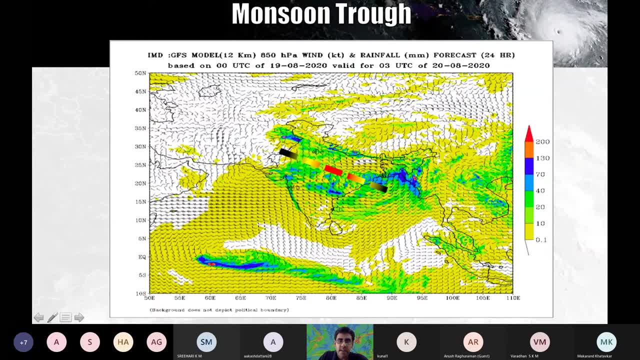 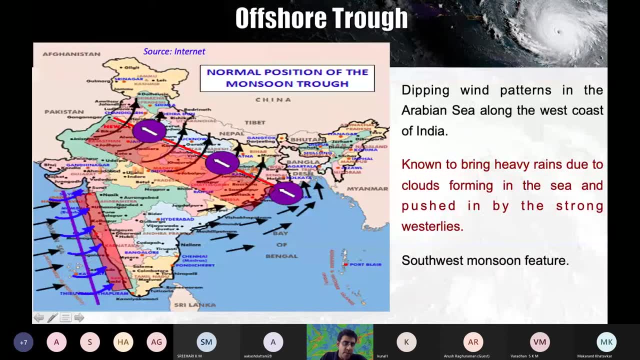 this is the westerly wind. wherever they meet, that is where the monsoon trough access is going to lie um: offshore trough. so offshore trough is nothing but the dipping down pattern of the winds because of the system in the way of penguin, and that actually is known to bring very heavy 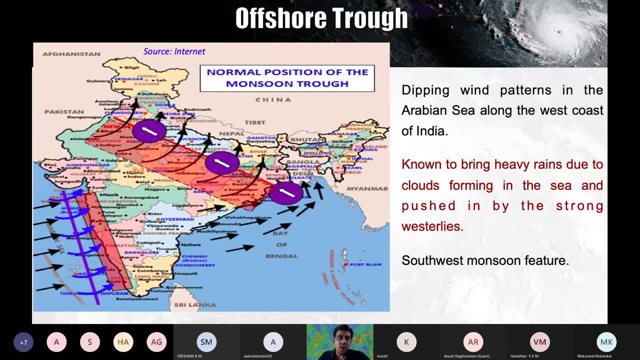 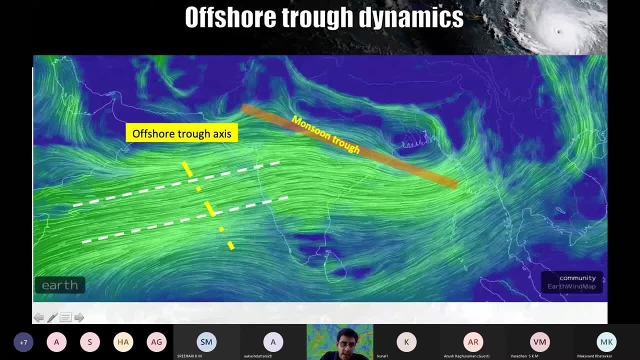 rain, and this is a very unique feature of southwest monsoon, especially for the for the west coast of india. how to find the offshore truck? look at the wind patterns. as the wind patterns are are showing a dipping kind of, so this is, this is the wind pattern and as they start coming towards the coast, 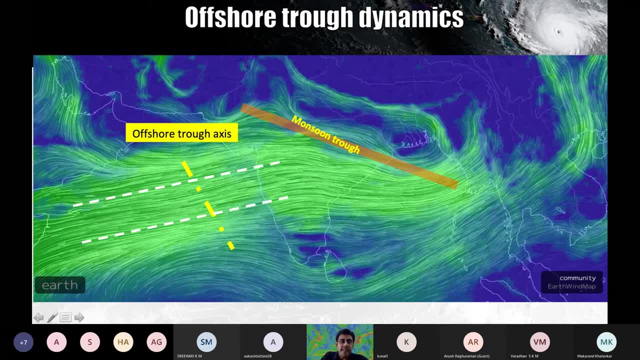 they actually show a dipping pattern, and that's where the trough axis lies and that's where the cloud bands form. the cloud bands always form close to the um, i mean in the arabian sea, and because of the presence of these strong westerly winds, these cloud bands get pushed. that is what i have tried to, uh, schematically show. okay, so these 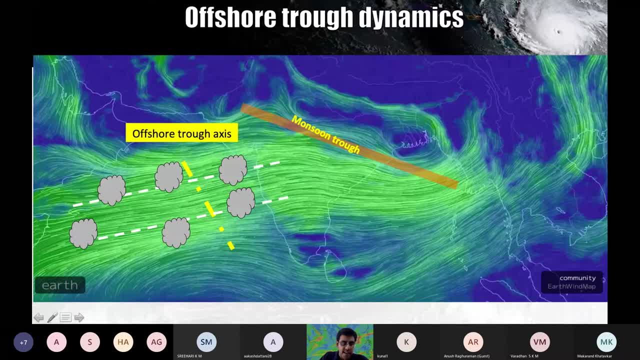 cloud bands. so during, uh, during southwest monsoon, you can see that arabian sea is always cloudy, okay, uh, so these cloud bands will get pushed because of the strong westerly winds which are present, and that is what gives rise to these rains for west coast of india, all the way from north to 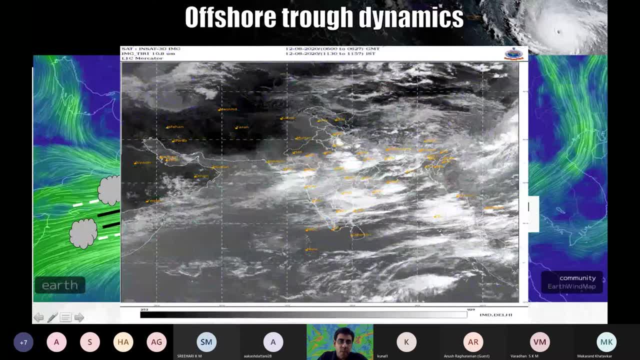 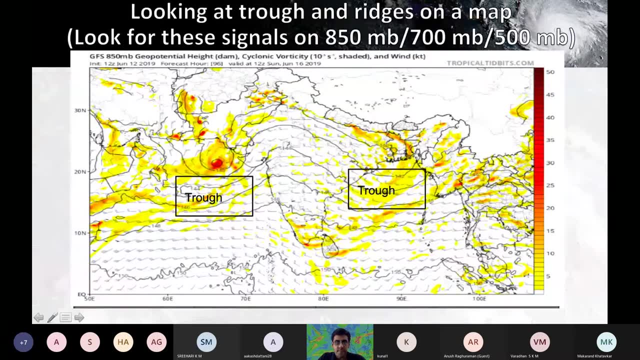 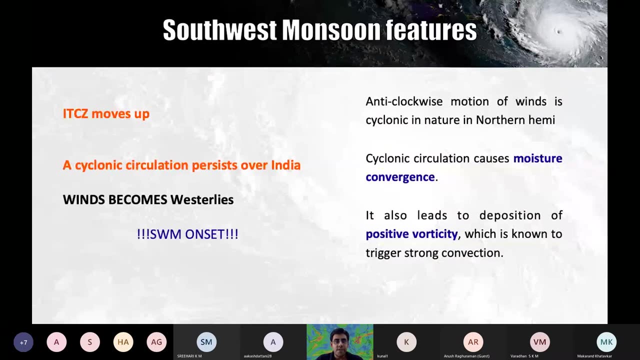 north of india. nothing is Spiritual at all, so that's how we get a lot of rain. yeah, so you see, this is the offshore truck dynamic, so these cloud, cloud bands will get pushed in and that's how you get a lot of rains. so, uh, before i wrap up, the features of southwest monsoon, or ITC said, moving up a cyclonic. 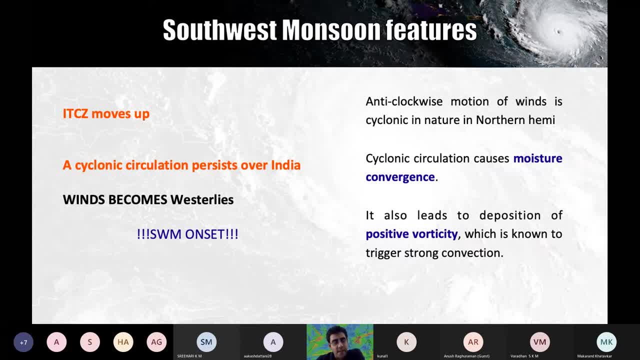 circulation persisting over india and winds becoming westerly. that is what is the classical, uh, the south-east monsoon onset. So you are on the lookout for these three distinct features. These are the what do you call the repercussions of this So cyclonic circulation actually. 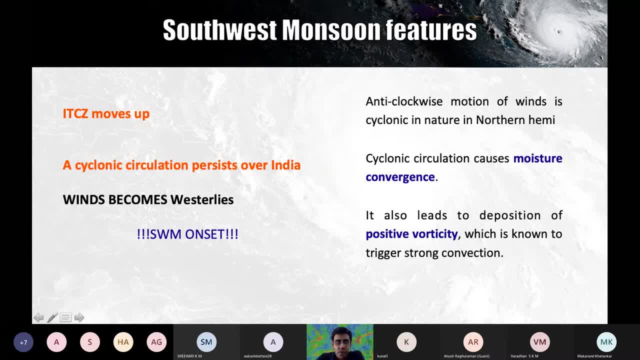 allows for moisture convergence. Westerly winds will always allow for a positive vorticity to get deposited in Bay of Bengal, which will create strong systems in Bay of Bengal which will move along the monsoon route. What is the signal of south-east monsoon ending? 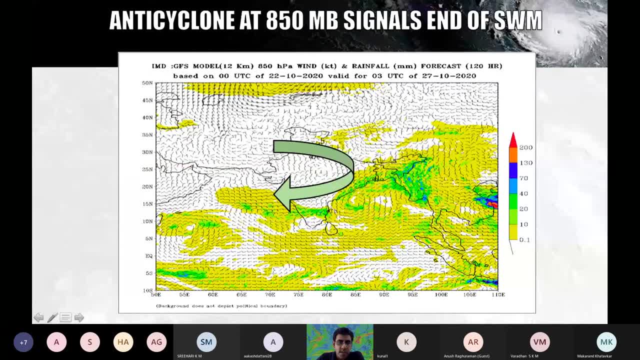 And anti-cyclone settling over India. So during the monsoon season the winds were like this, They were cyclonic. When they become anti-cyclonic. so basically, westerlies setting over Delhi and easterlies setting over central India is the signal of end of the monsoon. 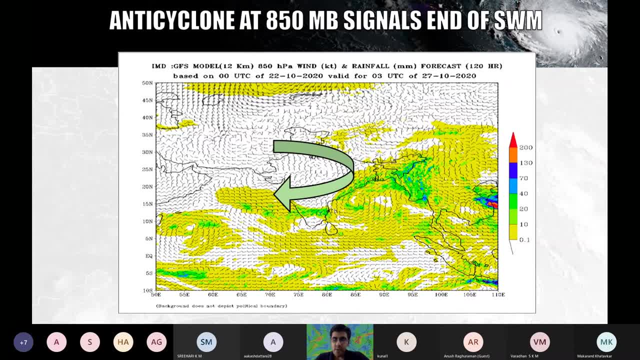 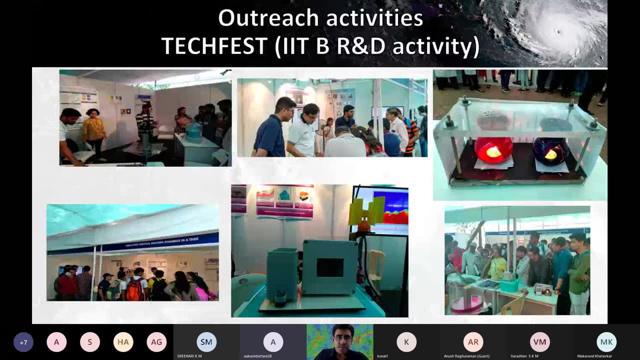 season. So the wind patterns reversing is the signal that it is going to end. So any doubts about monsoon, I mean? so let me wrap up and if you have any doubts, we can have five or ten. We can reconvene at around 2.20 or 2.30, no problem. I just want to show one slide before. 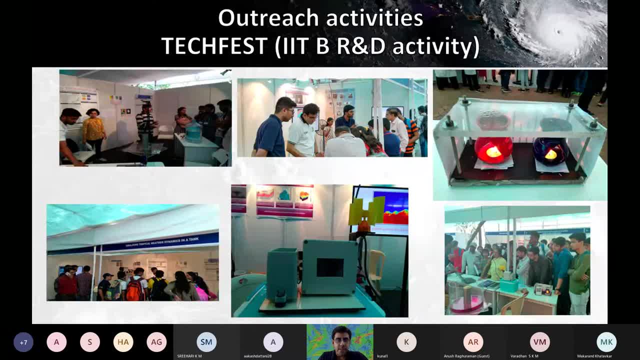 I wrap up. So we do a lot of outreach. So there is a tech fest festival thing that happens in IIT Bombay. It is a festival which it's an R&D festival where we have, where we set up these kind of stations, where we demonstrate many things- This year, of course, because 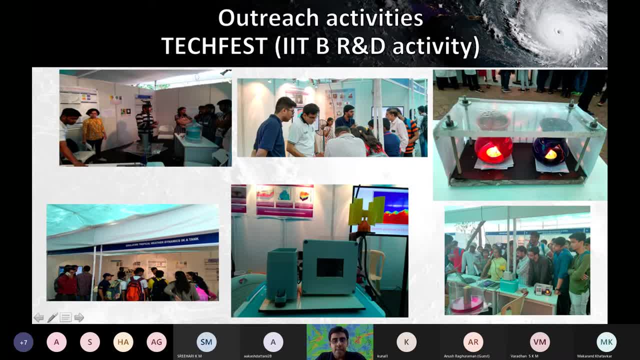 of COVID, we couldn't do it, But last year we had done it and it was actually a lot of people came, they visited and we demonstrated a lot of things. So this year, of course, we are going to demonstrate small, small things in a tank, which is a small, small phenomenon. 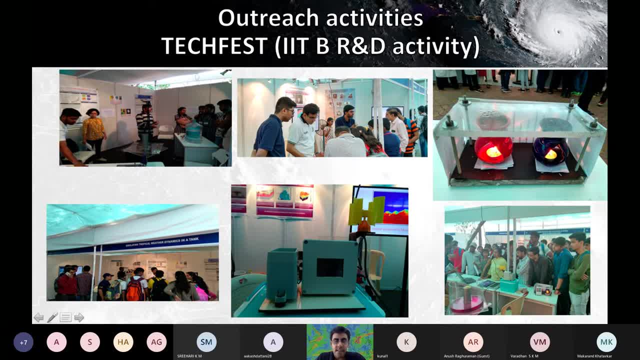 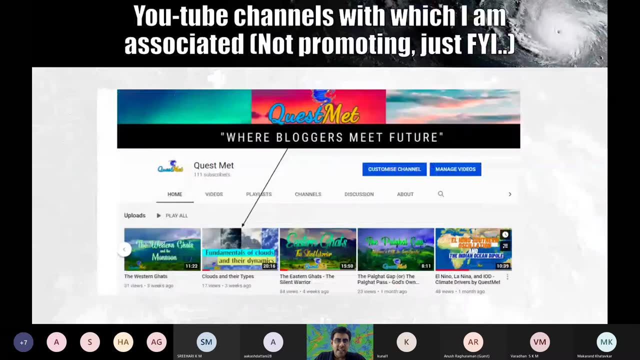 of waves and these kind of things in a small tank. So next time it happens I will keep you in the loop and you guys can just visit. and it is a very good activity for kids because they get enthused about these kind of things. And last thing is there are a couple of YouTube. 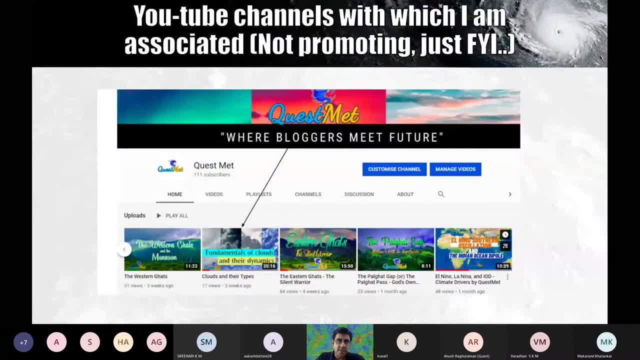 channels which I am associated. I am not promoting. This is just for your information. There is a QuestMed channel. I am not promoting it. I am not promoting it. I am just promoting this channel, which actually we try to make very professionally edited videos We have 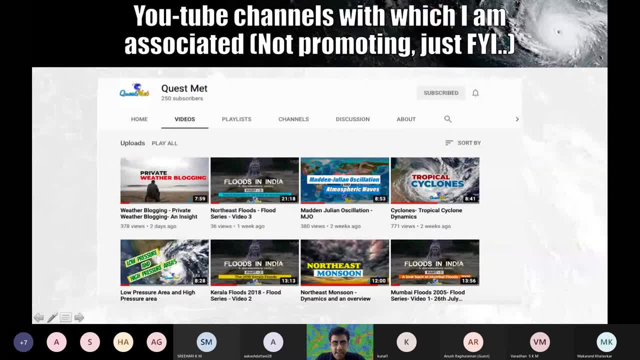 a professional editor who actually makes nice videos for kids, especially Some simple eight or ten minutes video maximum which tells a lot of things about what is managing oscillation, what is, what are cyclones, what are low pressure, high pressure areas, So you guys can take. 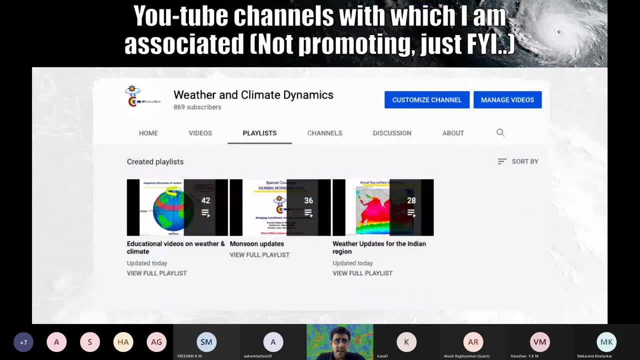 a look at it And I have my own weather channel, which where a lot of information will be available. So if you, if you have any suggestions, you can tell me and I will be ready to make a video and upload it. All right, So yeah, I am done now. 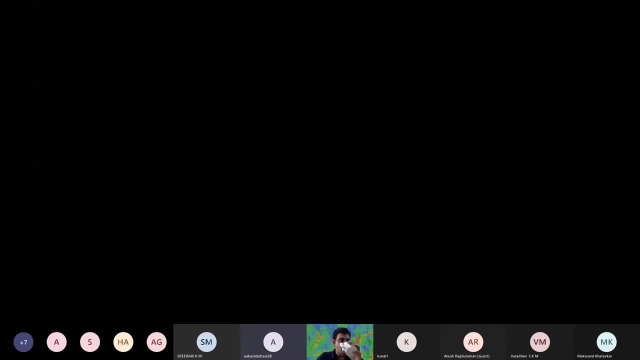 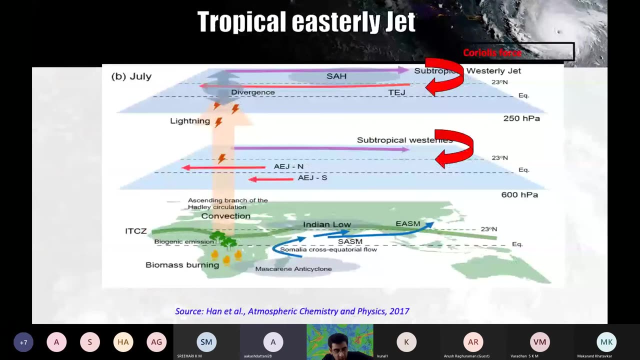 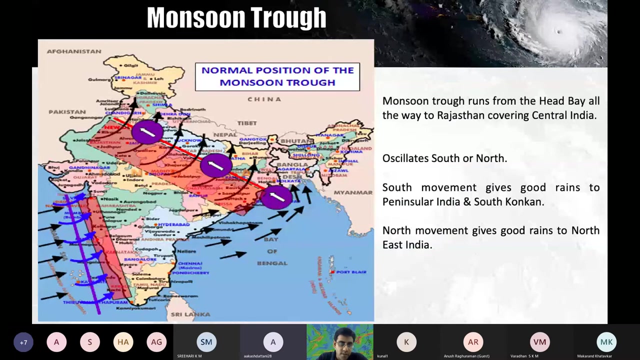 Can I ask a quick question on the offshore trough? please Yes, please Yeah. So what is the role played by the Western Ghats in the formation of the offshore trough? Western Ghats actually do not play a role in the formation of the offshore trough. The 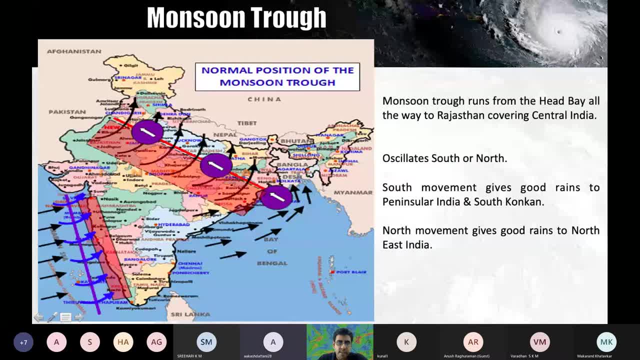 only thing that actually plays a role in the formation of the offshore trough is a system in the Bay of Bengal which pushes the, which allows the winds from the Arabian Sea to travel towards India. The role of the Western Ghats comes into picture in form of blocking this. 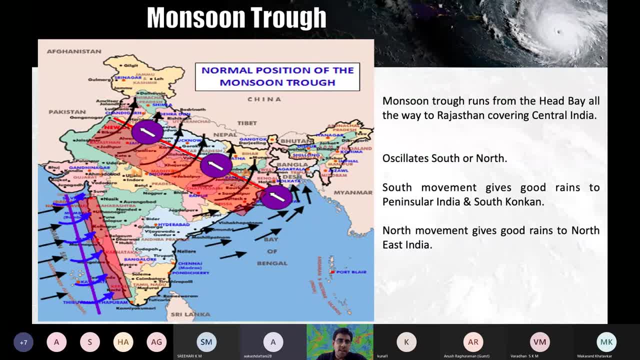 moisture and giving dumping lot of rain over the rain over the windward side of the Ghats. So that is the reason why the other side of the monsoon, other side of the Western Ghats, is usually dry And offshore trough usually favours regions which are on the windward side of the Western. 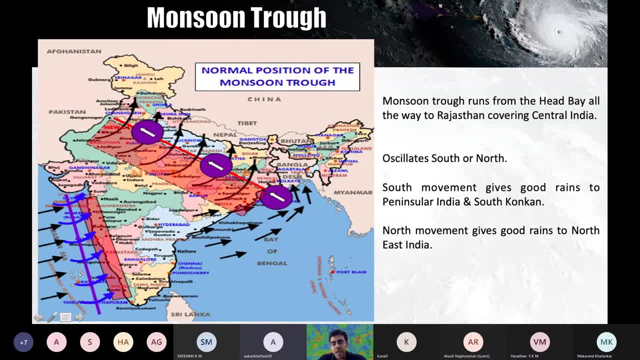 Ghats. So could one possibly argue that, say, a coastal station like, say, Bombay or Dhanu, if the Western Ghats were not present, the offshore trough would form regardless and those stations would receive probably the same amount of rainfall that they are receiving. 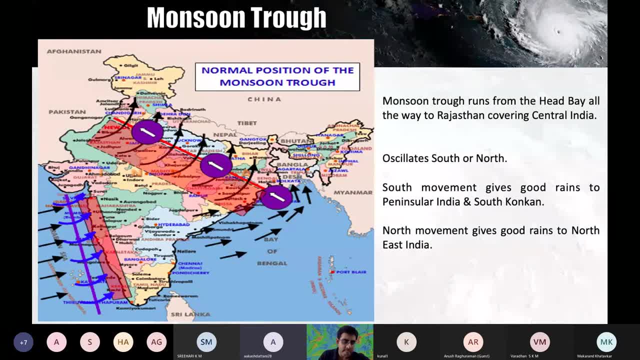 today, Yeah, Whereas other stations, like say Lunavala or Mahableshwar, would not receive as much rainfall. Yeah, So there was one kind of a hypothetical study that was done. I do not know if there is a paper published. 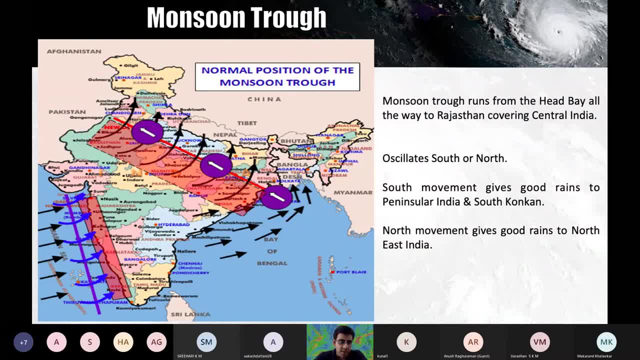 So offshore trough will form, no matter what, Because the offshore trough is a monsoon feature which forms mainly because of the winds. So winds are no way kind of offshore winds. are not affected because of the water, um, affected because of the presence of western guards. okay, so if you remove the western hearts, 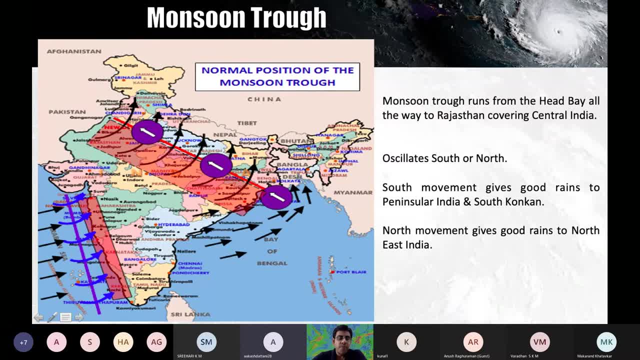 then what happens is? they found out that the moisture will reach all the way towards hyderabad, and they, what they found was that, in the absence of western hearts, these moisture which is coming in from the arabian sea has the capacity to dump lot of rain all the way up to. 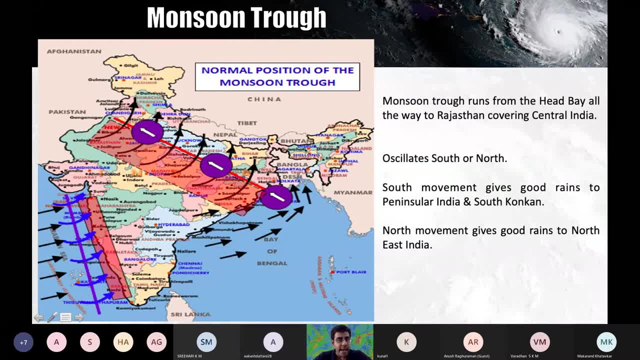 up to chennai, which is massive. right, because that doesn't happen because we have the western one. so hence, uh, southwest mountain season, chennai only receives like 400 mm of rains. so if you remove the western guards, then the only thing that will change is the variability of rainfall, so the 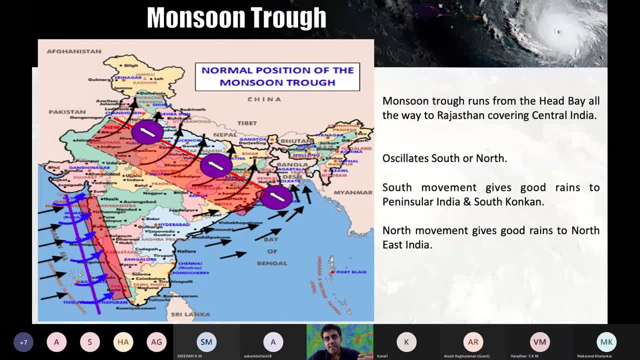 posture that that is now not getting blocked, has the free hand to move much interior and it's due to the presence of this western guards is the reason why you have marathwada and all these places are like that drought affected region: because the western. so because the marathwada and all these regions 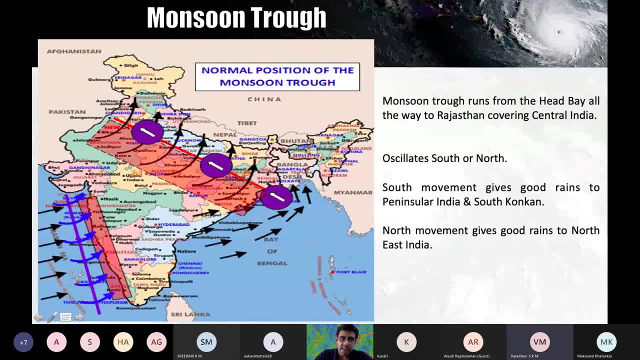 mainly depend on the monsoon troughs access. so any system in the bay of bengal moving from uh east to west is what uh these things are these regions are actually uh dependent on in terms of rain, in terms of rainfall. offshore trust is only for giving rains to these. 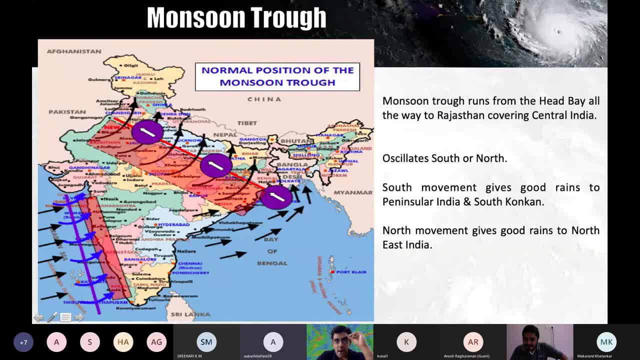 places on coastal. also the reason why we have all those rivers, right, uh, all those, uh. i mean that feeds the millions of people, correct, the reverse of them starts the people of chennai and tamil nadu. we are not looking for the monsoon, we are always looking for the breaks in monsoon because we 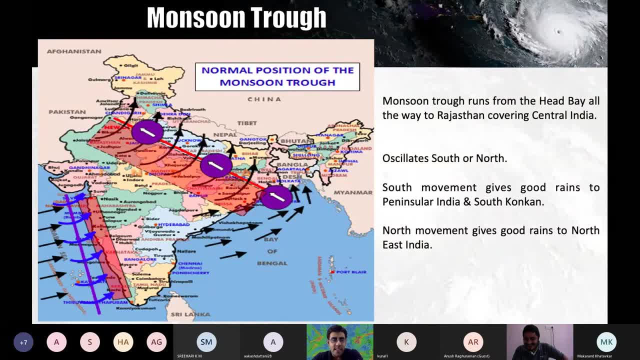 are looking for the thunderstorms. right, you are, you. for you, the break in the monsoon is when you get. uh, when is the break? because you know we, when it is active, we don't bother taking the umbrella or car, we usually take the scooter, but when it is thunderstorm, we always take the car, and so 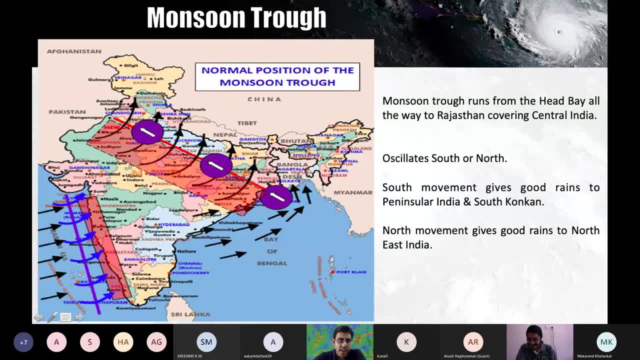 so, yeah, you're right, the break trace in monsoon over. so when it doesn't rain in mumbai, chennai gets rain. that is the correlation. yeah, sir, so marathwada obviously makes sense. it's the extended rain shadow region and we get such less. 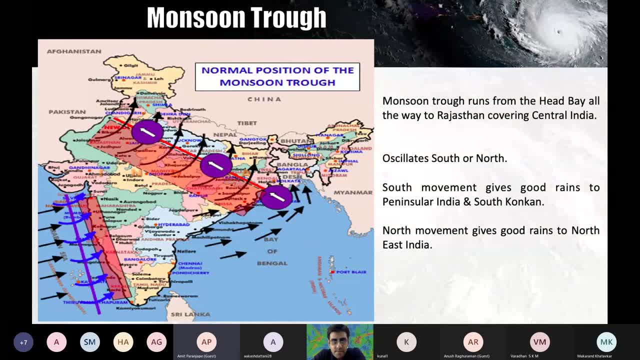 rain, but what explains, uh, the significantly higher rain average rainfall in witherba? then that's it, so, so, so, that is again due to the presence of monsoon draft. so it's you, you, you raise an interesting point which i was going to cover. uh, so what happens in uh witherba, or? 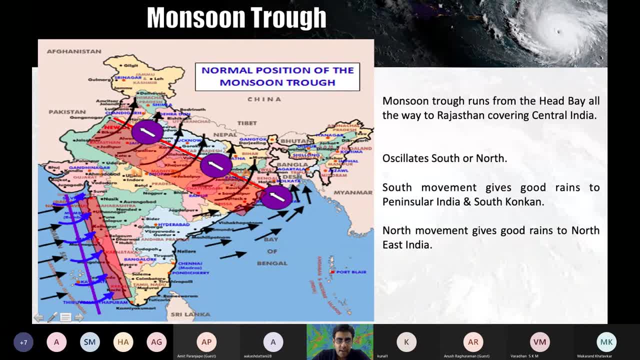 this, uh, this region, uh, is the location of that. so this monsoon draft has the inclination. so, starting from the east end of the arabian, sorry west end of the arabian sea, sorry west end of the way of bengal, uh, the monsoon trough is not a straight line. it always has an inclination. 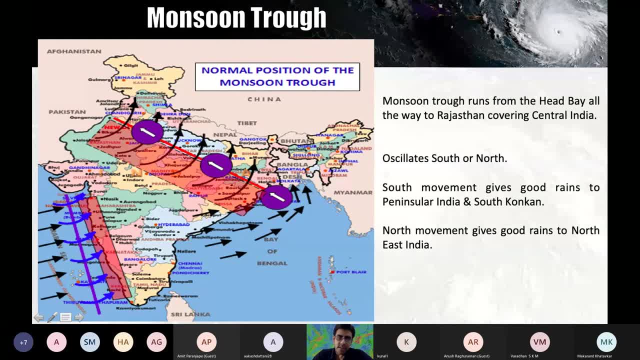 and for some reason or the other, i i don't, i this is something which is uh, which is which which i think we are researching. this particular monsoon axis trough most of the time passes through witherba, okay, and when that happens, the monsoon trough, uh is a, is is a very important aspect, because any 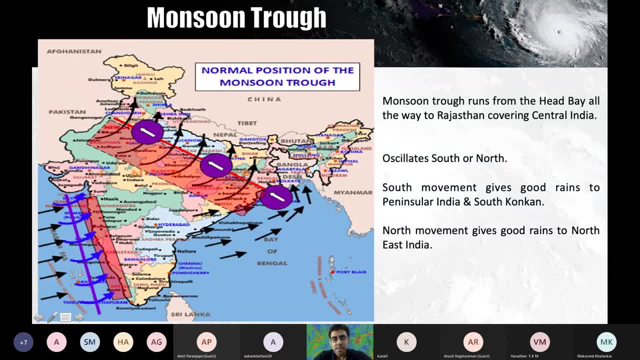 system, any, even any low pressure system. it doesn't have to be a strong system. even a low pressure actually moves along the monsoon trough, like i told you, and that is the reason why your places in madhya pradesh and witherba actually end up getting more rainfall, because your marathona. 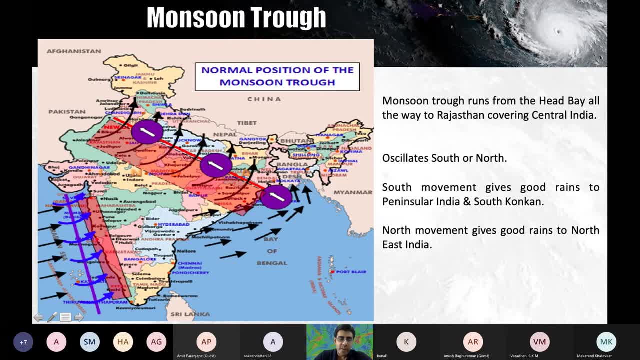 regions are much south of it and the monsoon trough doesn't, for some reason, doesn't cover this, cover these, uh, these regions. okay, so there's a preferential- i would say there is a preferential- alignment of the monsoon trough, which is something which we, which i don't understand. why is that? 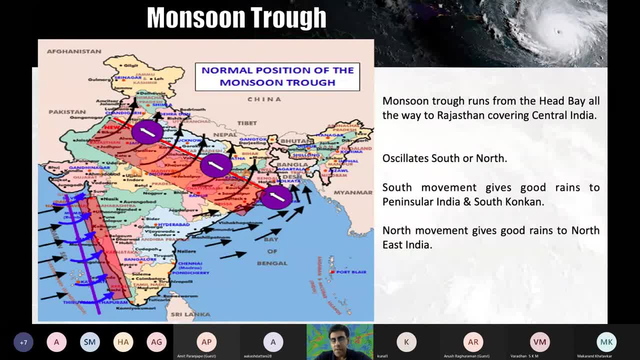 and it, most of it, most of the time, it misses marathwada. so that is the reason, and of course, the offshore trough, this offshore trough doesn't enter all the way up to uh, up to marathwada. so that is why this pocket is kind of always a deficit, because it is not. 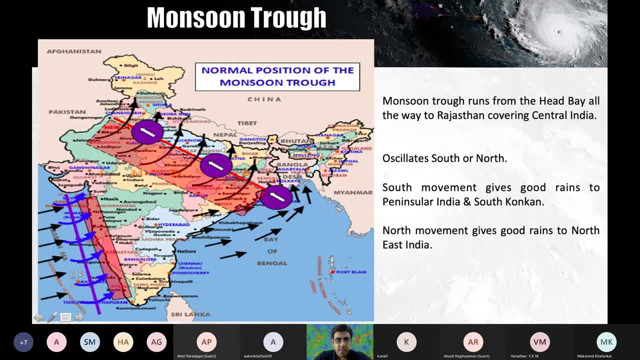 it is not uh. it is not uh held by this monsoon truck and it is not also held by this uh monsoon axis which, for some reason, move. sometimes it is over kerala, it dumps a lot of rain over kerala and then it swiftly moves towards this place. 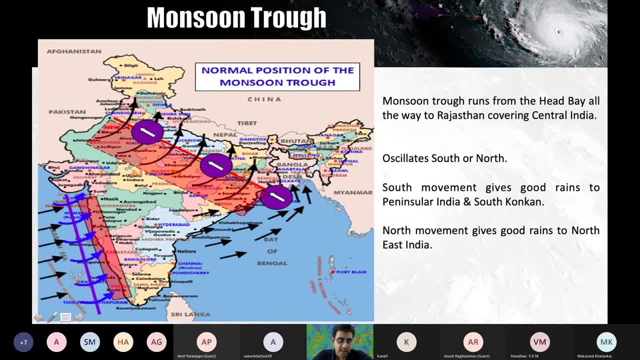 i don't know why it misses this region, that i i still i mean that's, uh, that's, that's something which we should think about, but it swiftly moves very quickly from this place to this place. uh, one reason could be: uh, due to the formation of storms. if you look at historical records, uh, most of the 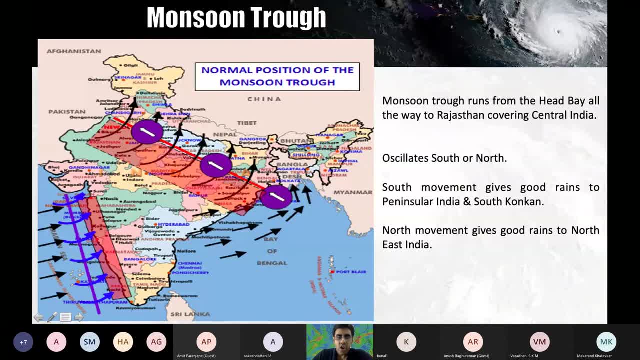 systems in bay of bengal either form uh in the southwest bay of bengal or northwest, not the bay of bengal. they don't form here. last year, october was the only reason, only one uh, one off situation where a system formed in kind of this central bay of bengal which actually moved along. 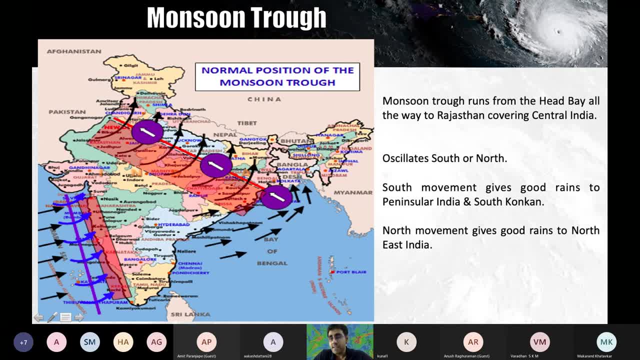 this monsoon trough axis through marathwada which i gave a lot of unseasonal, not unseasonal rains, which gave a lot of rains towards to marathwada in october last last couple of months. sir, yes, sir, actually yesterday i asked one question north of vijayavada, only this. 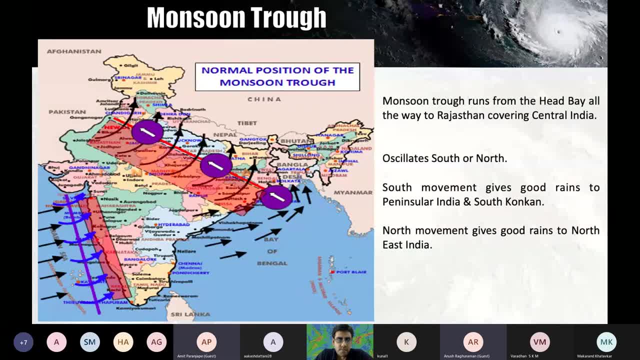 southwest monsoon is very active, sir. below that, that south royal simon, that velo region, right right. so that again, i think, is it due to the curvation of the course, sir, i don't know whether the coastal belt- see again, i'm not a, i'm not a topographic, i mean coastal kind of an engineer- uh, i, i still like to pinpoint it. 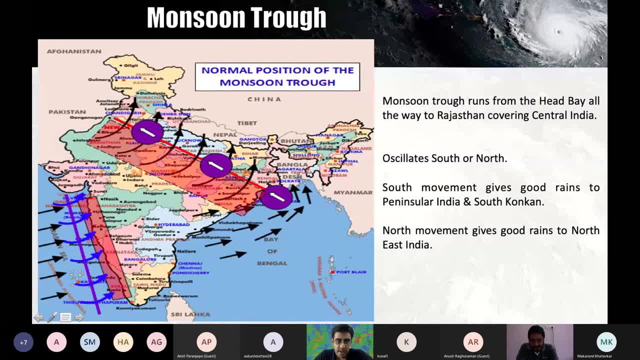 to the dynamics, and the dynamics is again telling me that this monsoon truck is the reason why this particular place doesn't get much, because the monsoon truck for some reason misses this uh place and uh, historically, uh, i have i have seen that systems in bay of bengal, either form, 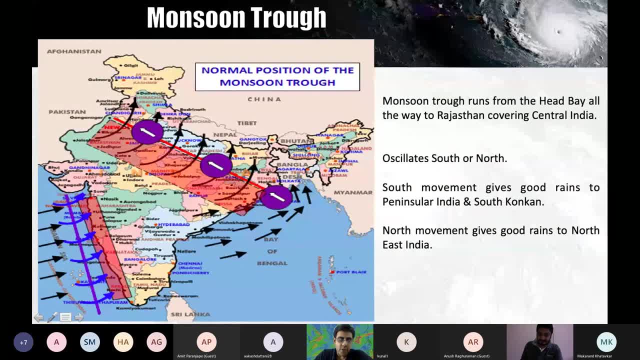 uh, kind of south of it or north of it, and that is we have to understand. so systems forming means vorticity. deposition happens either here or here. so one of the things that is a question is why these places are the hot spot for deposition of vorticity, or deposition of low pressure, low 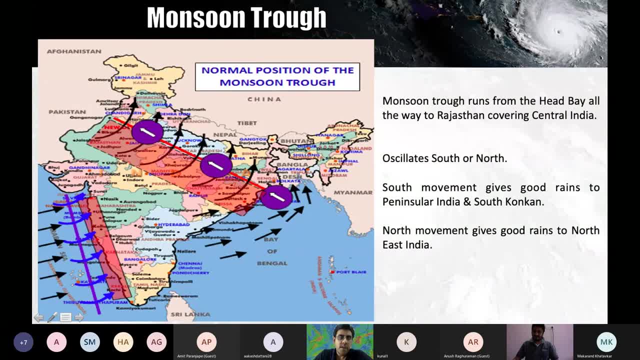 pressure systems. why don't? why doesn't the low pressure system form here, near, uh? let us see, because the low pressure system forms here, then your monsoon truck access will actually move along, uh, and that will give you a lot of brains. so for some reason that doesn't happen during. 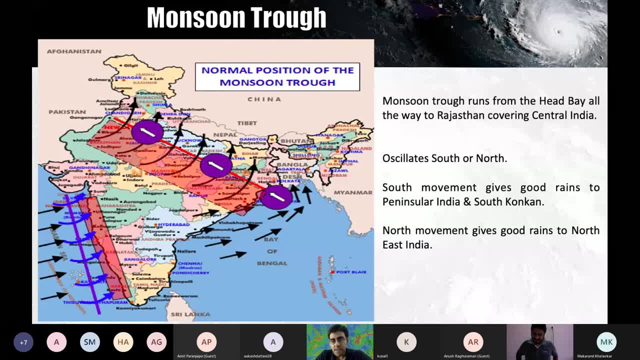 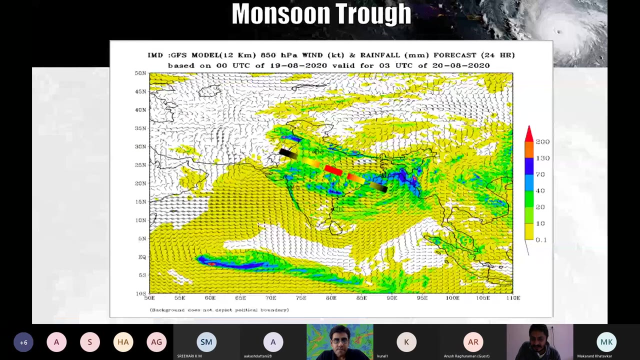 that that doesn't happen multiple times during, uh, southeast monsoon and an extreme south, sir, around two to good eternal million. there is a very less southwest monster about only one centimeter or two centimeters, and only wind flows during the. the reason, sir, in tamil nadu, anush, uh you know, uh southeast monsoon, kanyakumari, and uh you know. 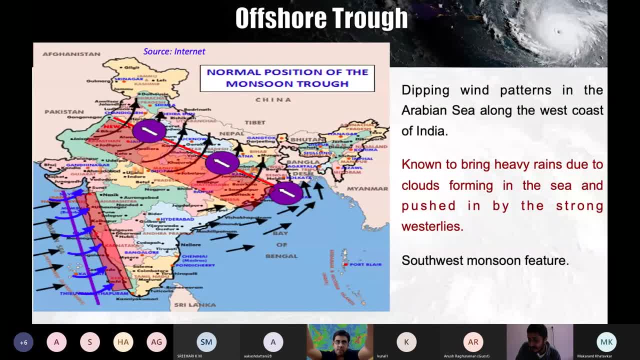 gods of, uh, gods of tinselville district, they all get rains. yeah, yeah, they get, they get. but, uh, those, those regions that we are talking about, tuticorin and uh, you know we are in the range from june to october. yeah, we get from thunderstorms. we should be thankful for whatever little droplets that fall. 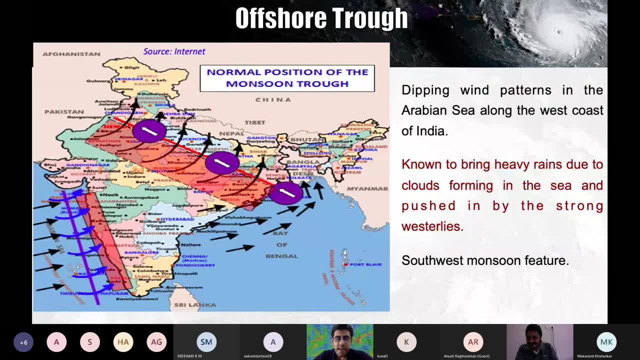 on us, correct? because, see again, like i said, the western guards play a very important role in blocking these moist, moistly moist laden winds. because if you remove these western guards, then you what you? you will get a lot of rain in other places as well, but the western guards block everything and they dump a lot of rain on the other side. 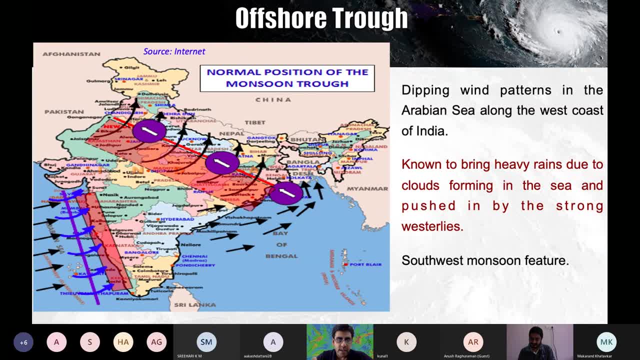 the western side of india and i think we we get only rains during the june to september or october, and we should be thankful because we have western class. uh, from june to september, that's it, that is the quantum, and we should be thankful because we have western class.